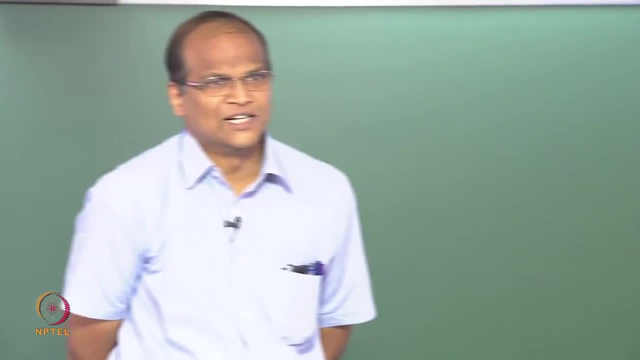 like this. So the average has to be less than 0 degree centigrade for it to remain as frost. So you can see that there is some the permafrost. we have depicted it up to 50 meters right depth. 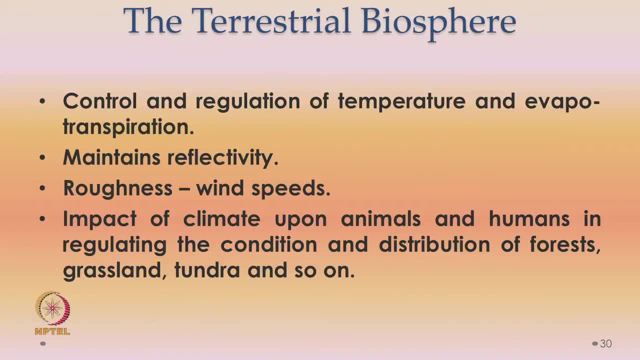 Okay, The terrestrial biosphere was the last component which we saw in the last class. We went through these slides very fast. So, actually the most important thing, it controls and regulates the temperature. Vegetation always controls both temperature and precipitation, So you. 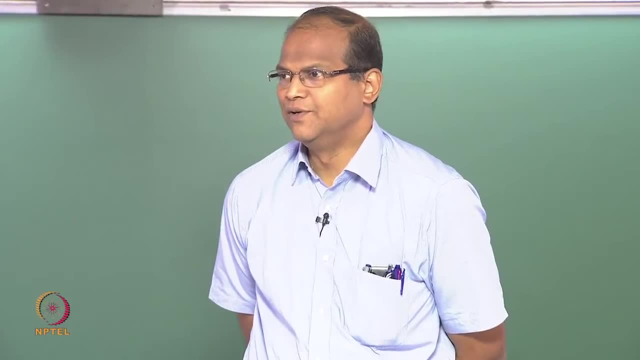 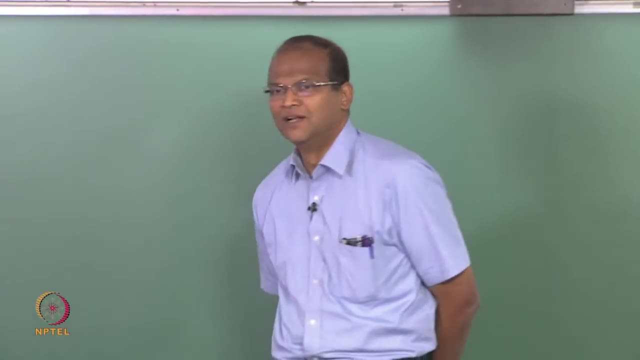 can see. for example, in Kerala you get more rain, okay, Basically because the monsoon hits there first and so on, and also if it is more green. For example, IIT, we have a temperature drop of 1 to 2 degree centigrade when you enter the campus from outside. That. 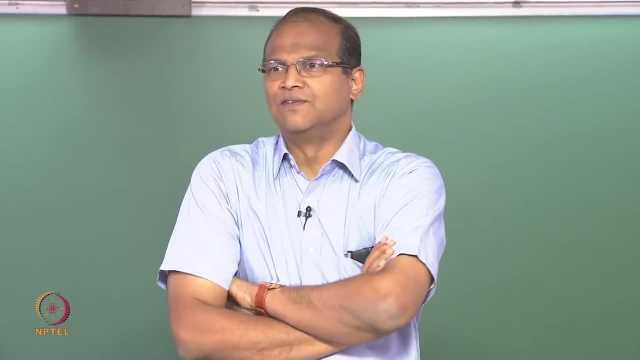 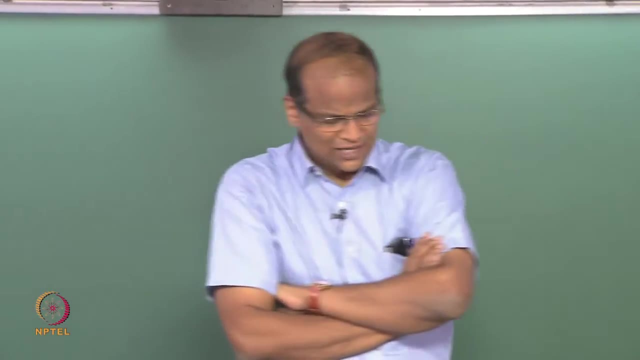 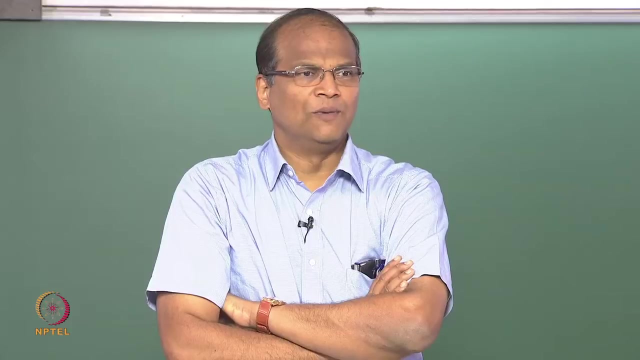 is because of the thick vegetation. Okay, So there is also an important process which is basically the evapotranspiration which takes place in the plants, and also this vegetation maintains a particular kind of reflectivity right. So, as you can very well imagine, the reflectivity from a tropical rainforest is. 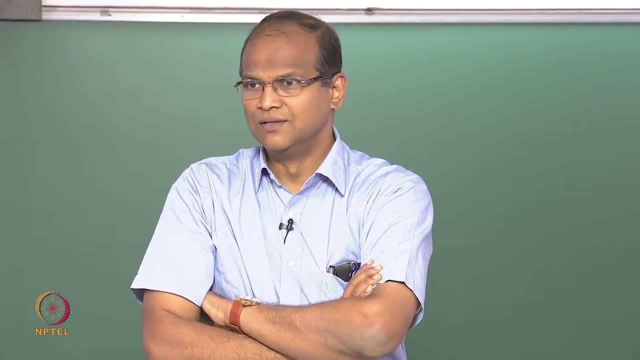 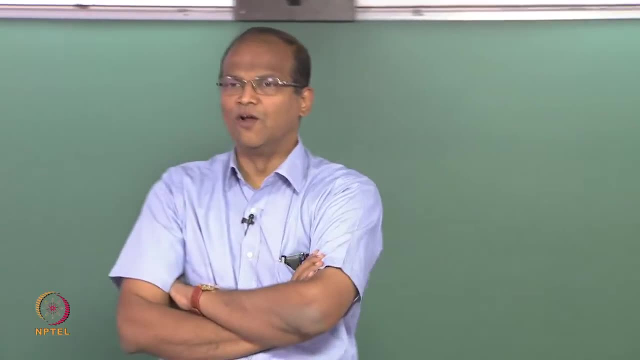 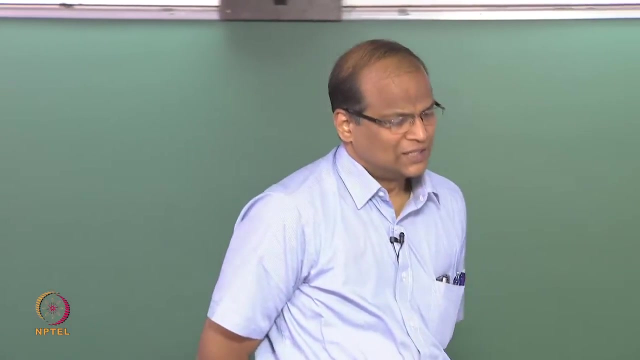 quite different from a reflectivity from a just barren desert in Saudi Arabia, for example. right, So this has ramifications in basically outgoing long wave radiation, incoming radiation, the amount of radiation which is captured, the reflectivity Okay, And all this radiation balance and also this vegetation can alter the roughness of the 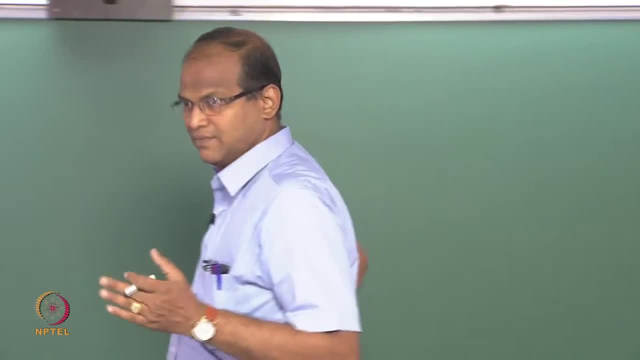 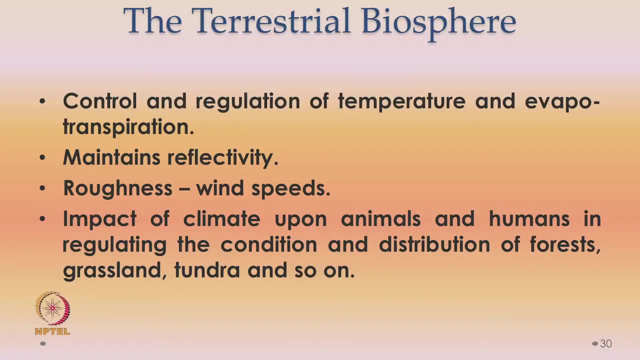 surface, The roughness will alter, the wind speeds correct, And then the impact of climate upon animals and humans. and in regulating, because of the terrestrial biosphere, we are also there, animals are also there. So the impact of all this animal life on regulating the condition and distribution. 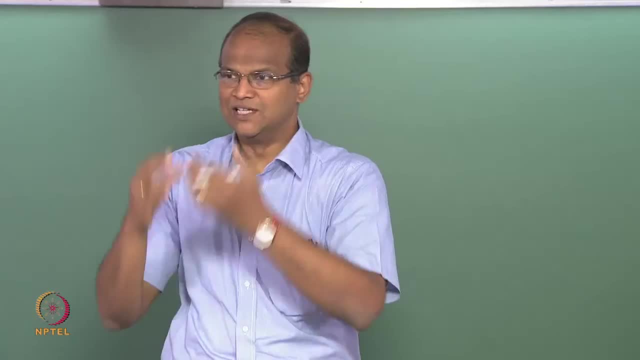 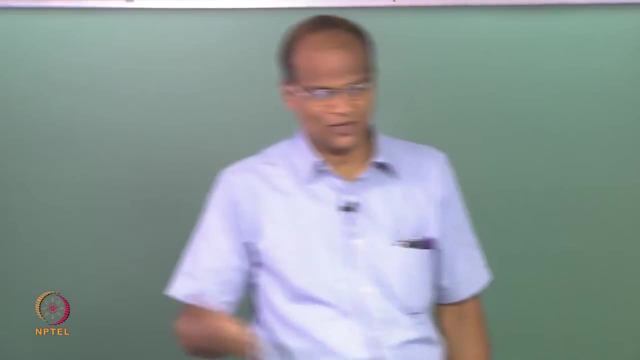 of forest by afforestation, deforestation, etc. Okay Okay, Forest fires, natural, natural induced forest fires, man induced forest fires, all these things have a big role to play in deciding the climate of the earth. So the terrestrial 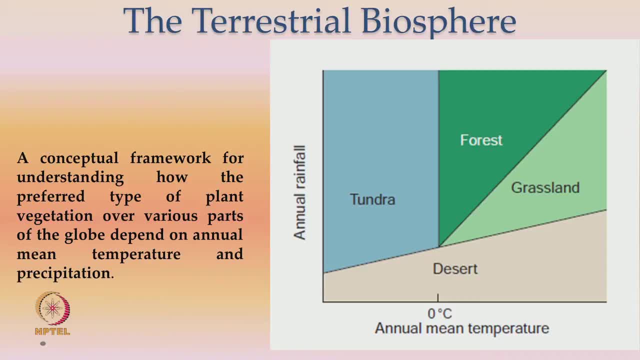 biosphere. this is a good conceptual framework for understanding how the a particular type of plant vegetation with various parts of the globe, how it depends, or how they depend on annual mean temperature and precipitation. So on, the ordinate is rainfall, Rainfall. 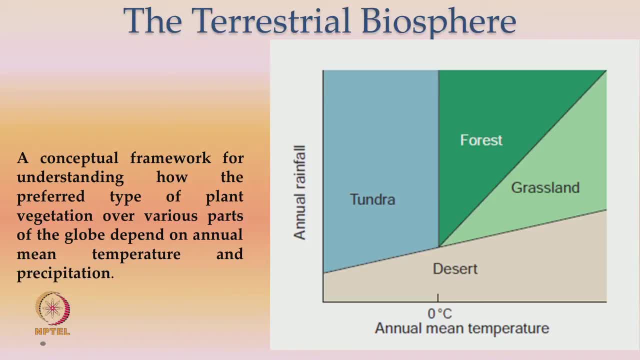 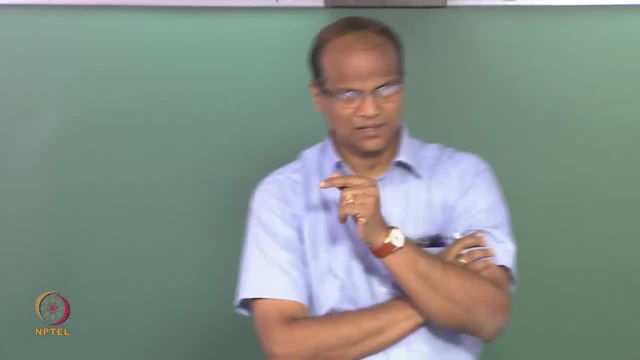 And on the abscissa is the mean temperature. So you can see that as the temperature increases- for regardless the type of vegetation, as the temperature increases, the amount of rainfall which is required increases, right, And obviously the temperature is going to be very high in. 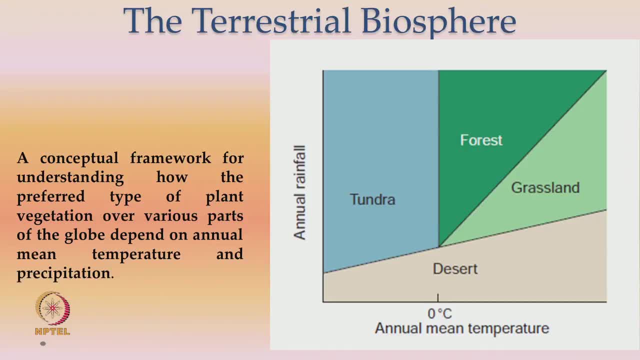 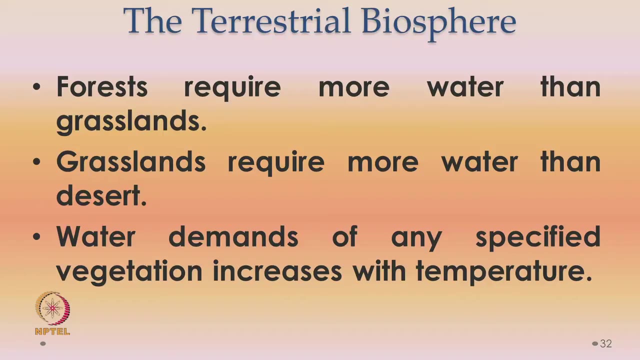 the desert region and tundra region, the temperature is low and so on. So you can move from left to right and understand how things vary. You can also move from bottom to top. We have already discussed this in the previous class. So to summarize that we have view graph: forest require more water than grass lens. 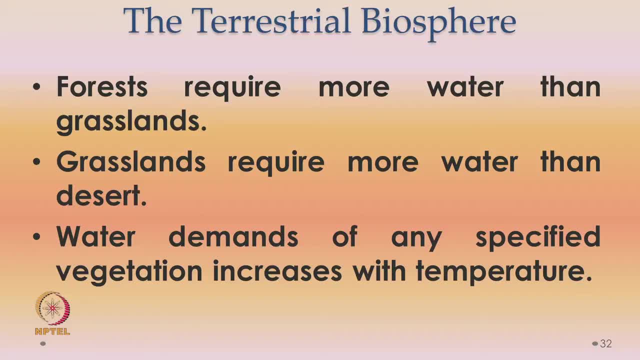 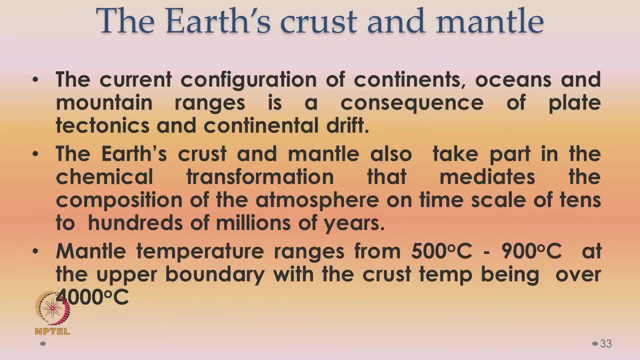 grass lens require more water than desert And for a within a particular vegetation. the vegetation, the water demands of any spec particular type of vegetation increases with temperature. Okay, So the last part, basically, which we are going to look at in today's class, is basically: 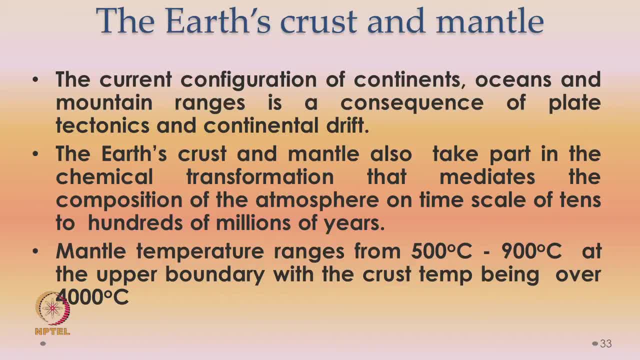 the earth's crust and mantle often not studied because it is considered as geology or geophysics and so on, But this also major role to play. One of the most important things. we have what we call the wetlands and the mud. 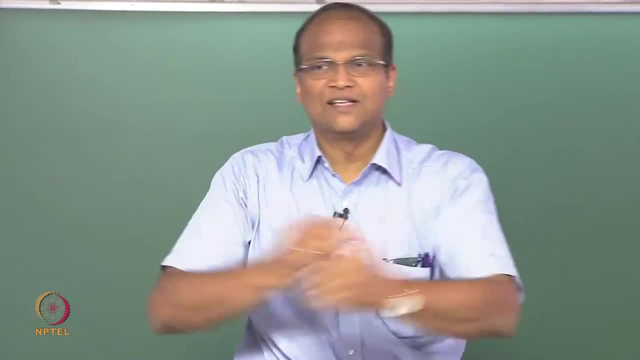 Now let us talk about the dry land use that we have done in the last class. So the dry I will to break the suspenses. the earth's crust and mantle have a big role to play in the way the continents have been shaped. 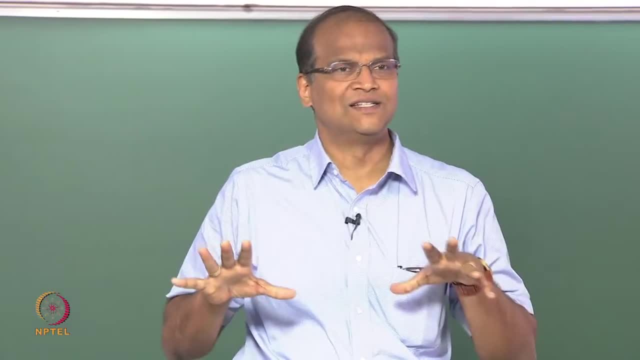 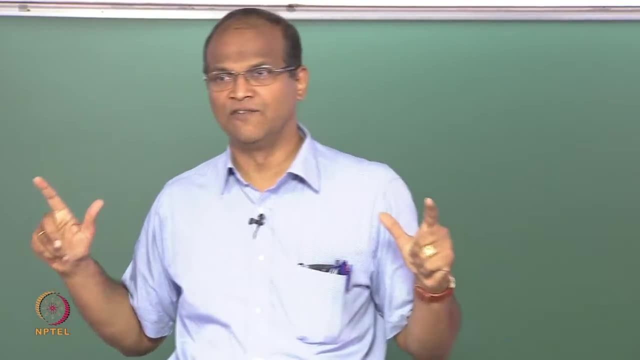 The way the continents have been shaped also is responsible for the way there are ocean currents, climatic regions. which regions prospered first? where did civilization start first? why did? why was steam engine figured out in Europe? and all that because life started. 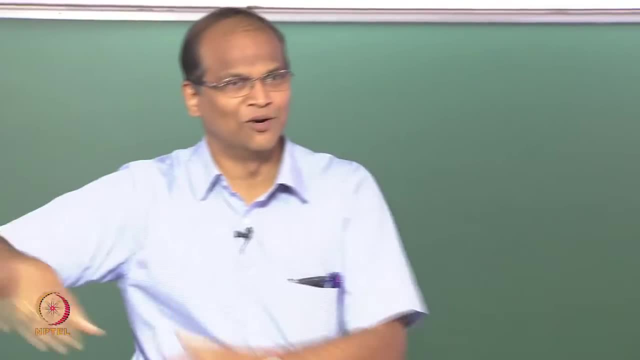 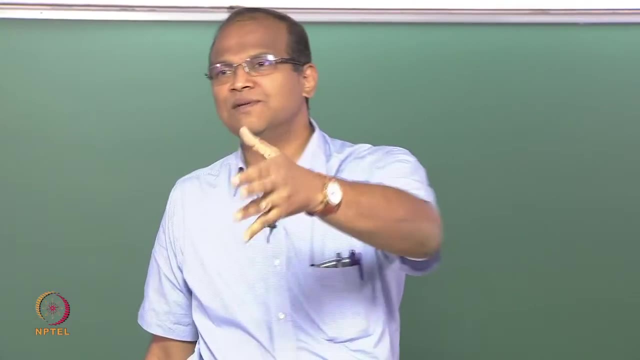 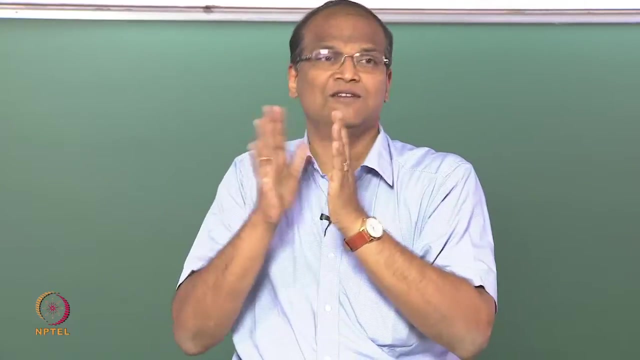 in Europe. first and all that It is not that some race is particularly too over smart compared to others, and so on. Here the Euphrates river, actually Iraq, if you guns, germs and steel- there is a book called Guns, Germs and Steel. so this earth's crust and mantle have a major role to play. 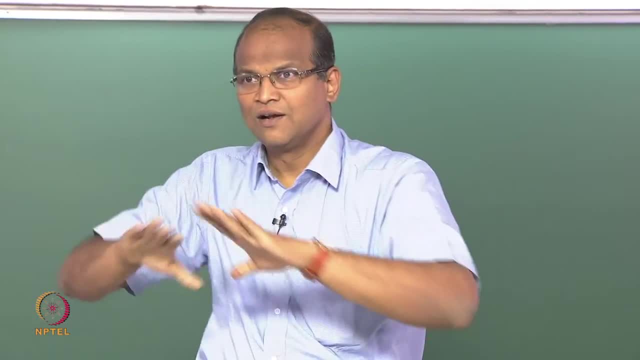 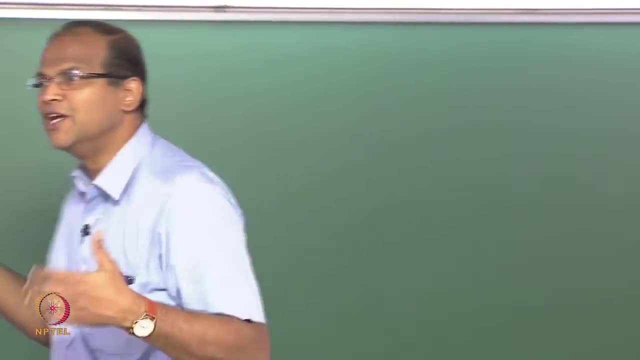 in deciding the shape of the continents. otherwise there is something called an aqua planet. When you do simulations, what we do is in atmospheric scientists when they do simulations, we can do simulations on what is called an aqua planet, and aqua planet is a simulation. 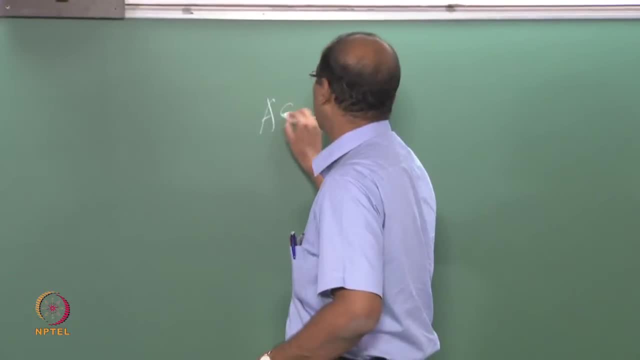 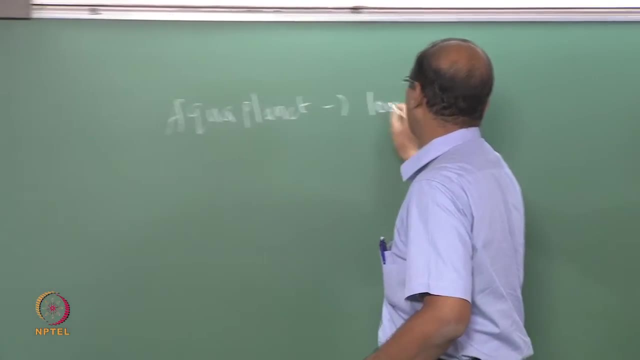 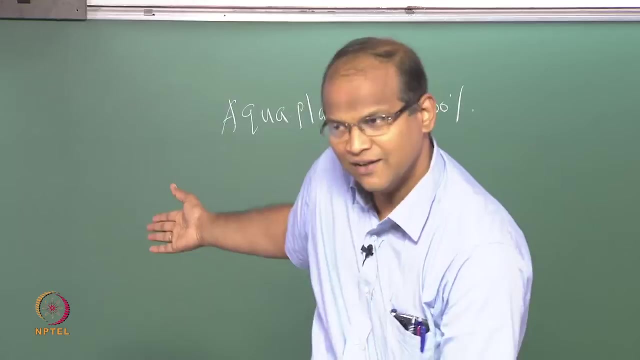 where it is 100 percent water. So in order to get quick estimates, we also look at this aqua planet simulations. it is not an aqua planet. it is only 72 percent aqua planet. 28 percent is still land. 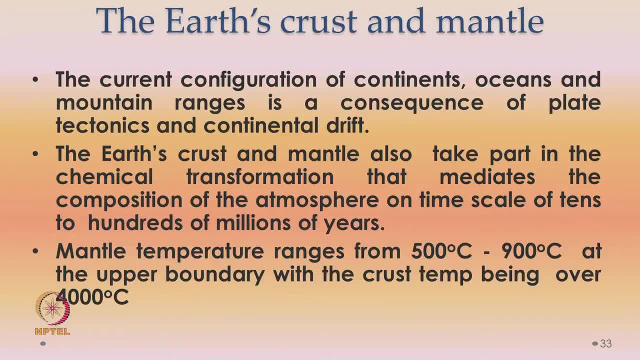 Now let us get into this. the current configuration of the various continents, oceans and mountain ranges is basically a consequence of what is called plate tectonics and continental drift. The plate tectonics is actually a theory. ok, it is now believed that it is correct, but 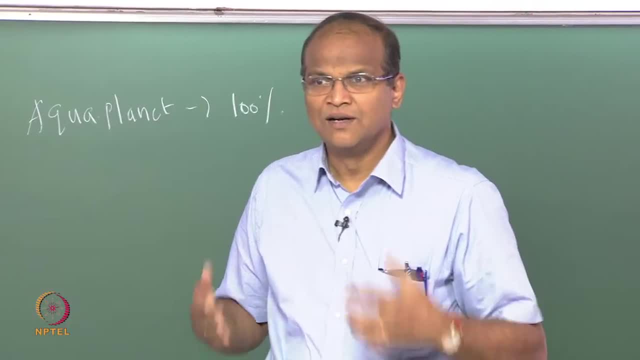 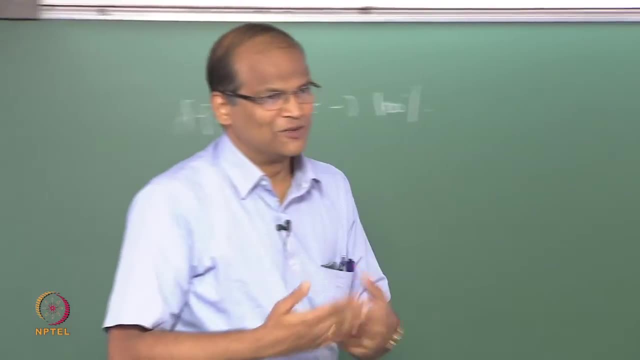 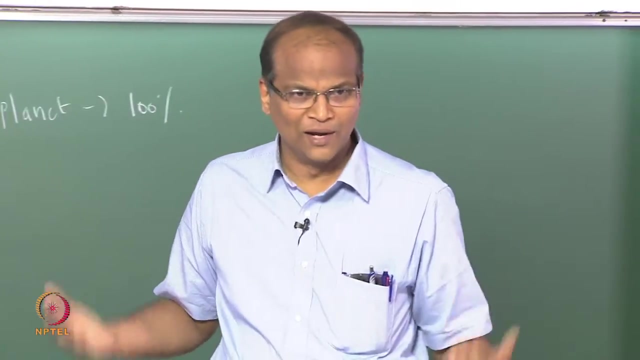 no theory is so sacred or sanct that it cannot be challenged. The goal of human creativity, enterprise and knowledge is to basically challenge any theory. ok, The hydrodynamic theory was challenged by Prandtl, and Prandtl's boundary layer theory is now considered to be the theory. it is not the be all and end all of fluid mechanics. 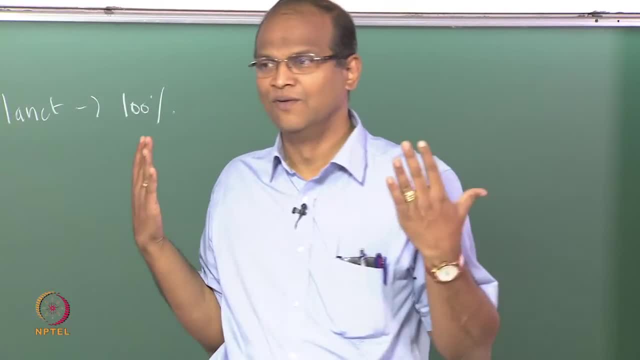 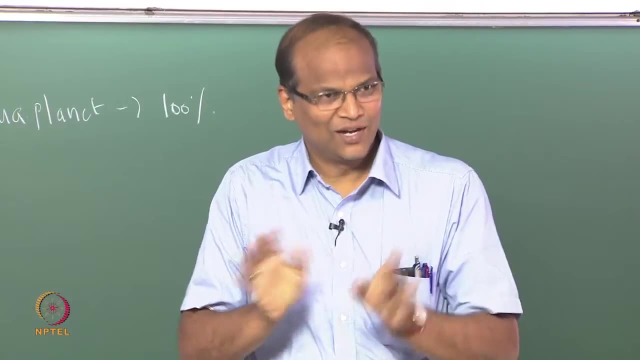 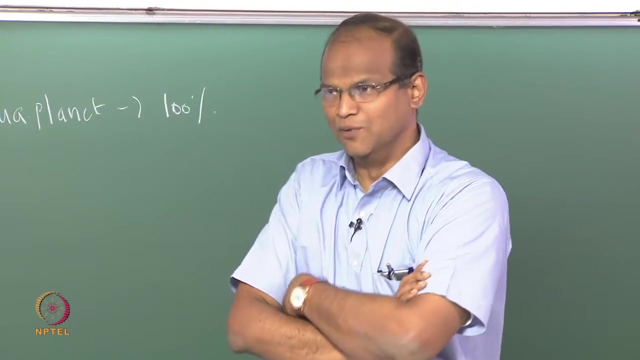 there could be a new theory which could explain things better as of now. as of now, E is equal to h, nu. As of now, E is equal to m, c squared. ok, as of now. boundary layer theory: delta by x is much, much less than 1, there is something called the slender length of the boundary. 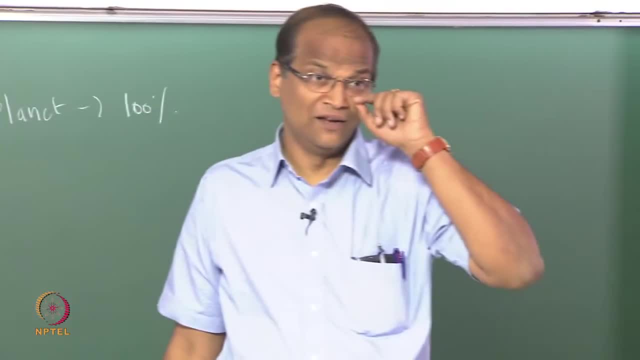 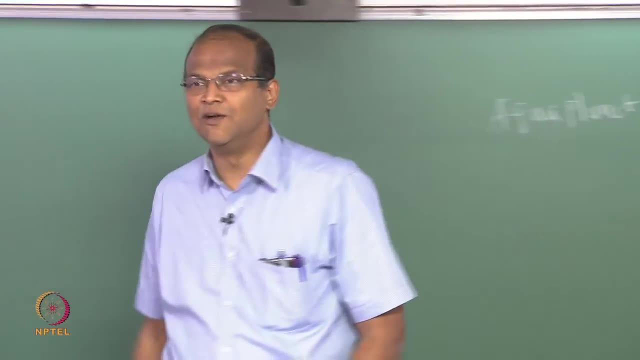 layer theory with which you can, with which you can simplify the governing Navier-Stokes equation and create and make them into boundary layer equations, which will transform the elliptic equations into a parabolic differential equations which lend itself amenable to mathematical analysis through a similarity transformation which leads to the Blasio solution. 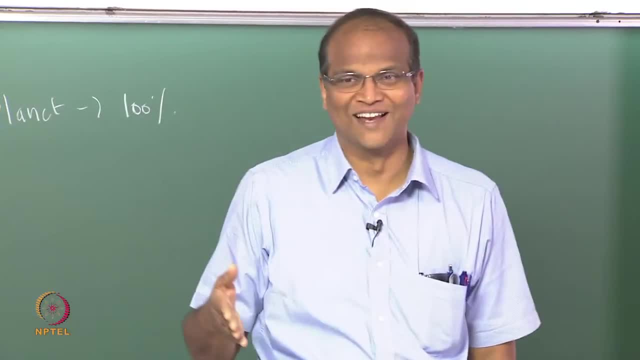 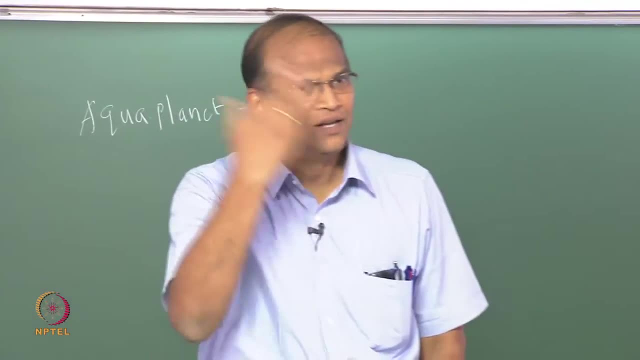 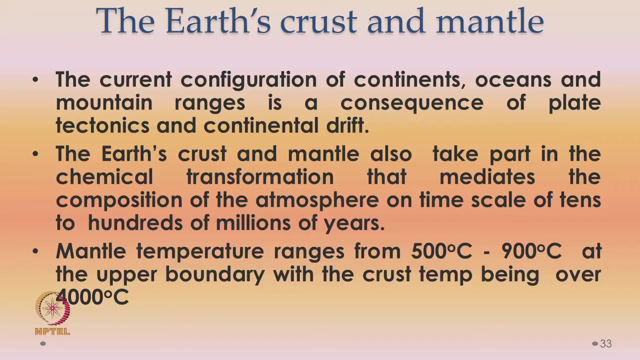 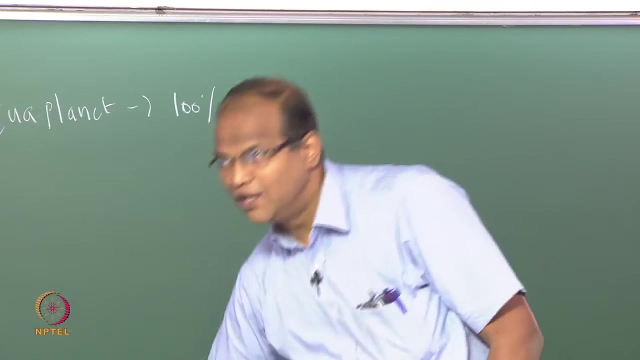 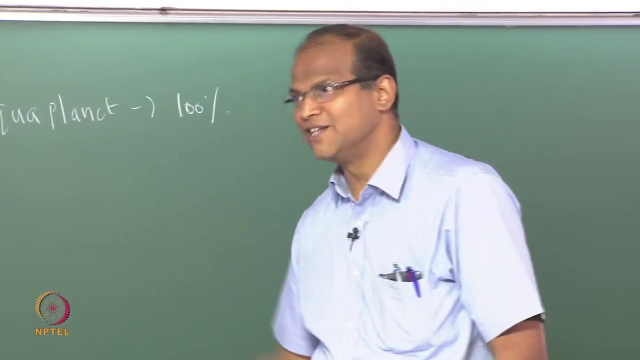 So it is a 2 minute course on this. Thank you, Thank you. Yeah, You also like. Thank you very much. Thank you very much. You also like to do its art supplies from deep inside the mantle to the atmosphere, So they also take part in the chemical transformation. 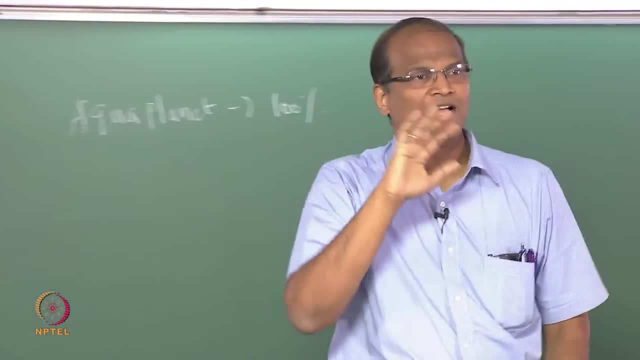 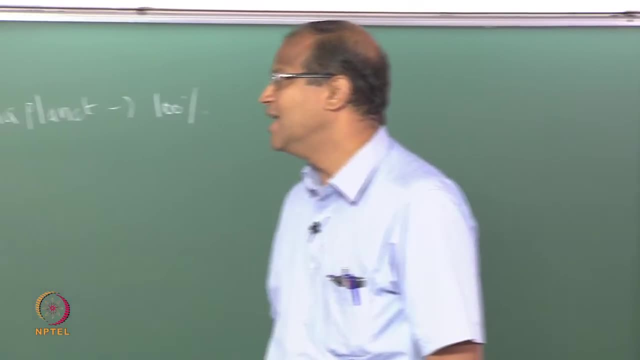 this can lead to changes in the carbon budgeting as well as the oxygen budgeting. Carbon budgeting means automatically carbon dioxide in the atmosphere, So that mediates a composition of the atmosphere and time scales of, but the time scale is not seconds or days or weeks. 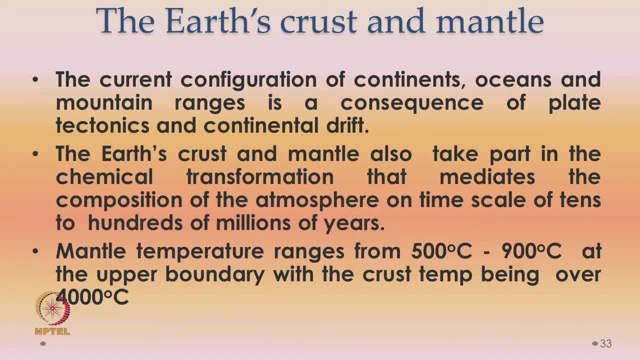 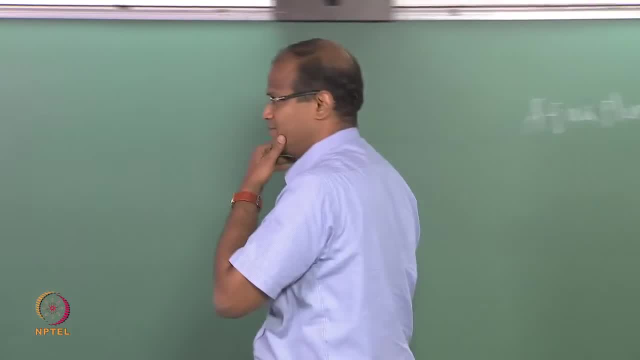 it is of tens to hundreds of millions of years. it is a very slow process. ok, So the mantle temperature ranges from 500 to 900 degrees centigrade inside the earth's surface at the upper boundary with the crust temperature. the crust temperature can be. 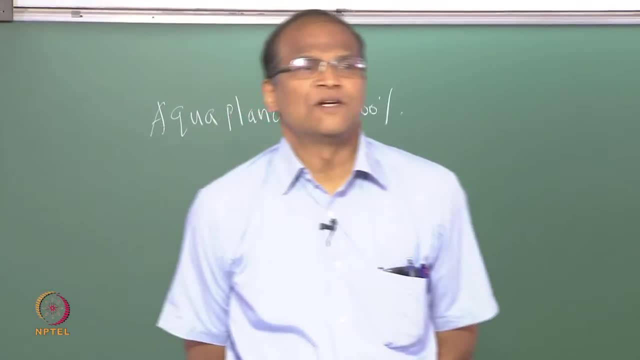 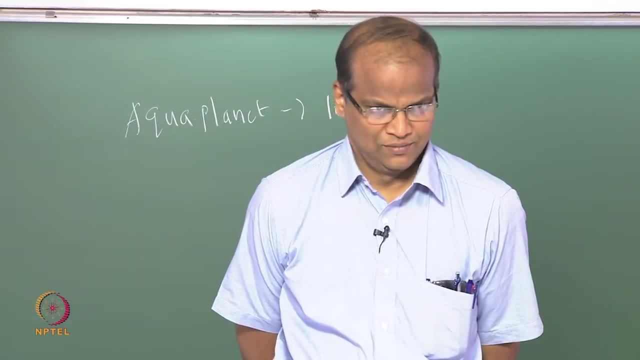 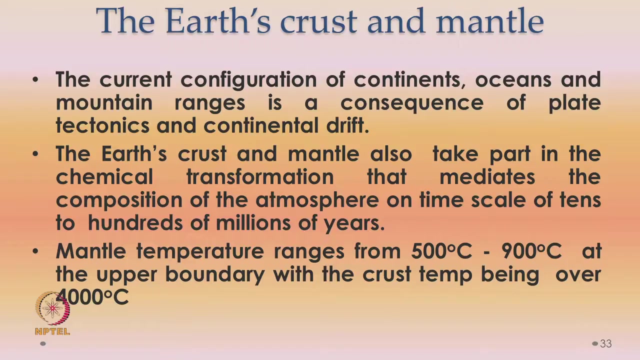 over 4000 degree centigrade. So this is a special plan. So this, if you are interested in doing this, you are going to study, as you are interested in, a subject called mantle convection- ok, Which comes under geophysics or geology or ok, mantle convection is same. 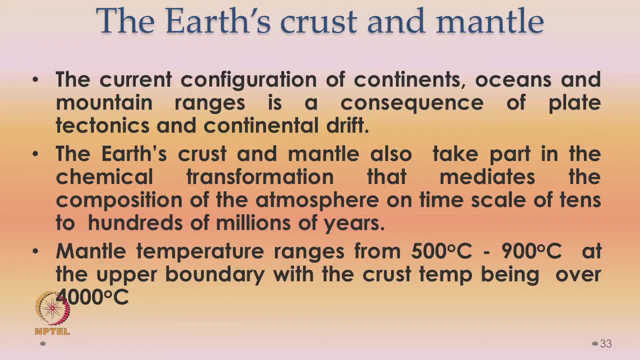 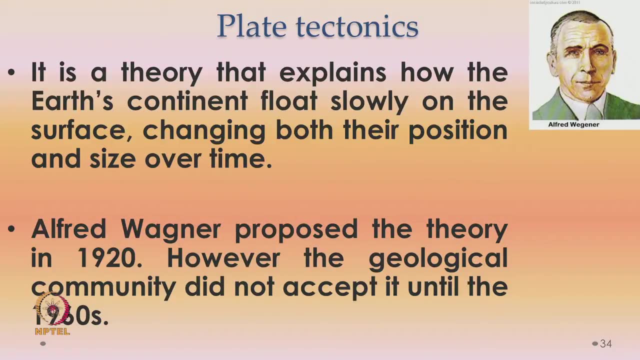 equations, fluid method, ok. mechanics and heat transfer equations will come, but scales will be very different, temperatures also will be very different. So your Boussinesq approximation and all that, we do not know whether they will be valid or not. ok, That is Alfred Wegener. so 1880 to 1930 lived for 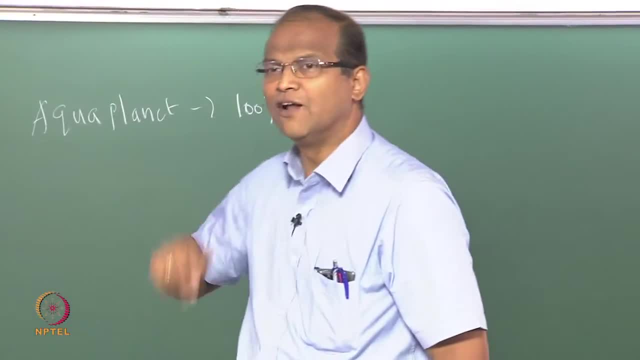 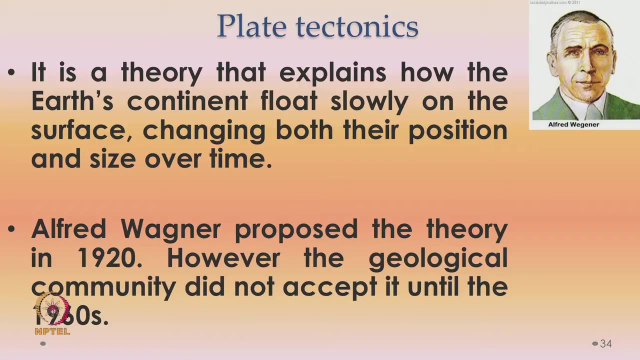 50 years, a German, ok, So he figured out this theory. he proposed this theory of plate tectonics. What is plate tectonics? Plate tectonics is theory that explains how the earth's continents float slowly on the surface, changing both their position. it should be earth's continents. 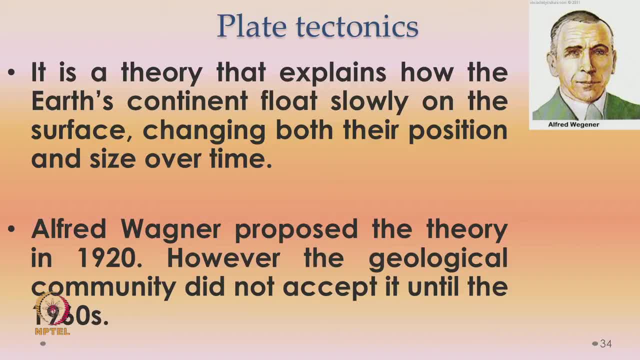 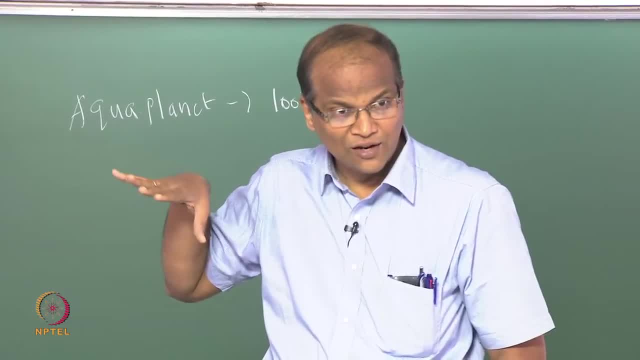 changing both their position and size over time. ok, the shape and size of continents. So they are saying that they are. everything is floating. that is what he is saying. ok, everything is floating on the mantle. ok, He proposed a theory in 1920, but, as usual, people, 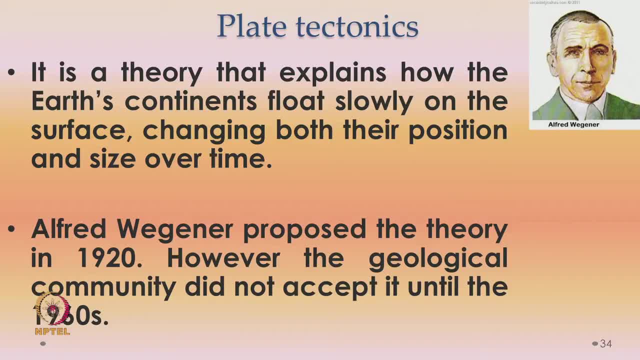 did not accept this theory for a long time. ok, So it took about 30-40 years. So it was: the geological community accepted this theory only in the 60s. So this acceptance of this theory was accepted only in the 60s. So this acceptance of this theory was accepted. 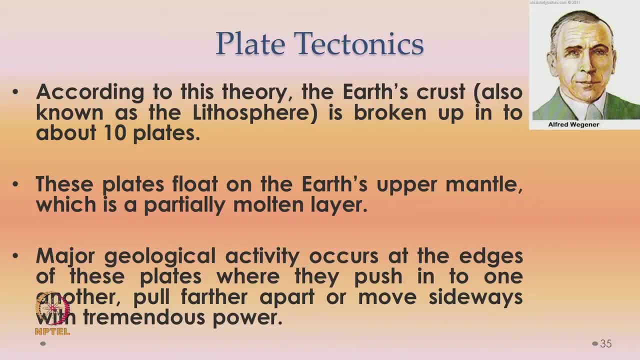 only in the 60s. So this is the Ganoderma region. the second layer of this very large plate is a sheet of metal That is geological part of the plate. so the layer of metal is 10 plates. So the 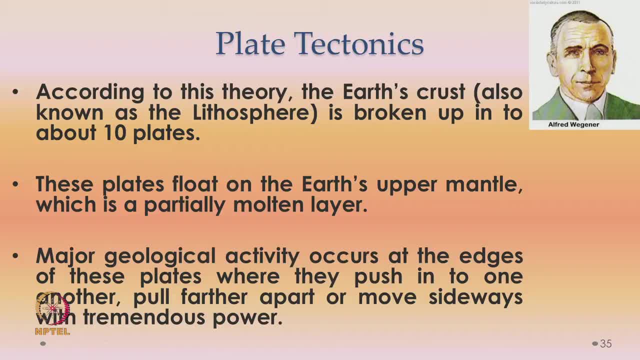 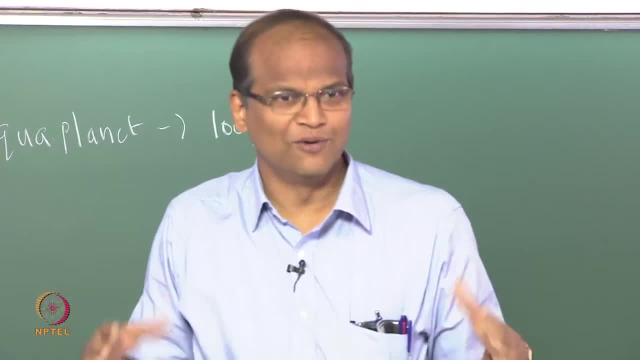 layer of layer is of 10 plates. In theепentheore there are 10 plates. on earth there are 10 plates, so the layer of metal is less than 50, is around 50 years old. What does this theory say? According to this theory, the earth's crust, also known as the lithosphere, is broken. 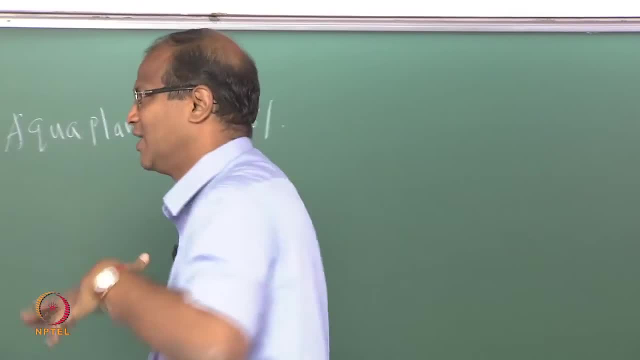 up into approximately around 10 plates. there are some 10 plates. These plates are actually floating. it is scary to hear this, but you hear about this, but this is the truth. they are actually floating on the earth's mantle- ok, On the earth's upper mantle, mantle is. 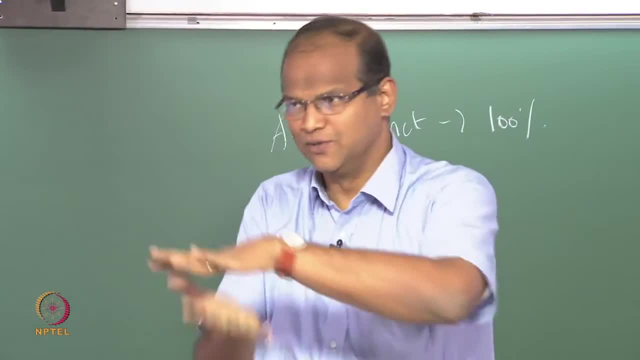 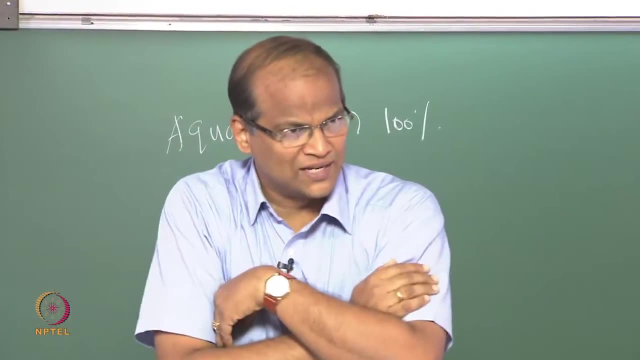 a partially molten layer consisting of various chemicals, liquids and all that, So these plates, liquids and all that, So these plates are floating on this. So the major geological activity takes place at the interface of these various plates, At the interface of these. 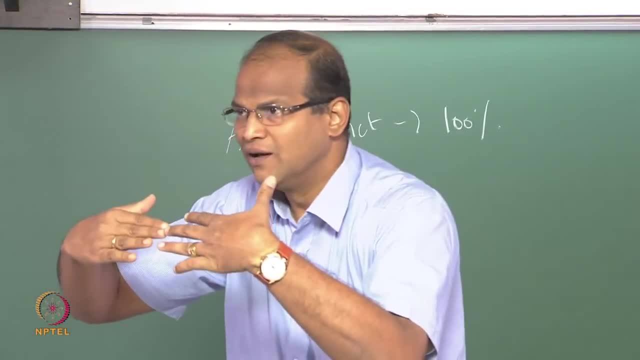 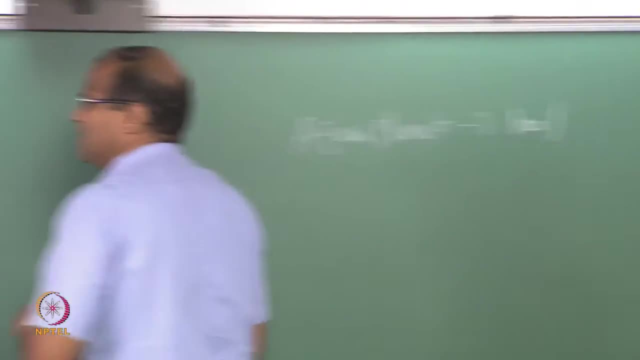 various plates. plates can approach each other. ok, then plates can move away from each other. there could be some shear between this. because of this, lot of geological activities are taking place. What kind of geological activities? Earthquakes, this thing and all that we will. 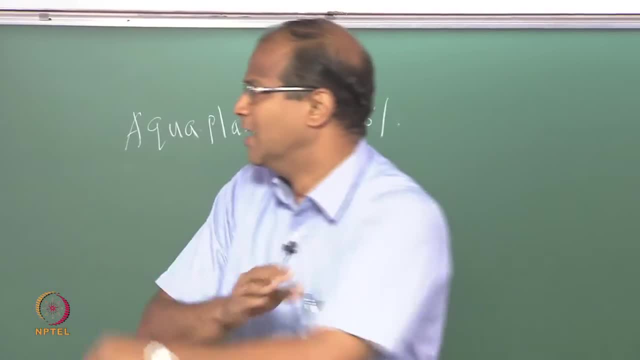 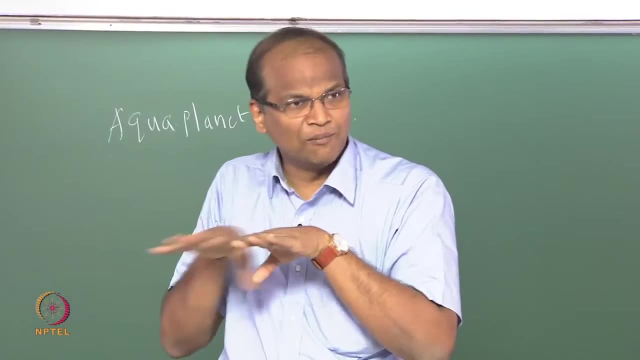 see, there will be some fault lines and all that right. seismologies work on this. So, wherein one plate tries to push into another, they pull further apart or move sideways with tremendous power. When these things are taking place, some action results. What is this action? 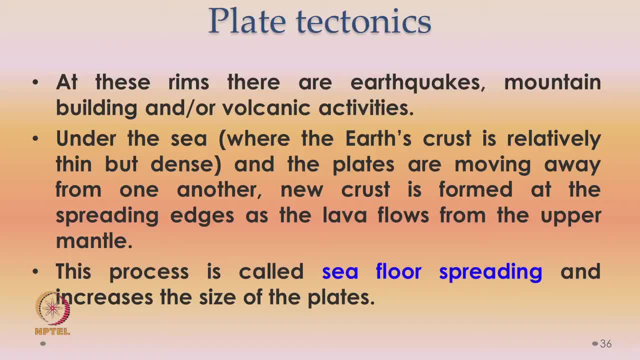 At these rims, where these actions takes place, there are earthquakes, mountain building and or volcanic activities. ok, This is a theory which he proposed. Under the sea, where the earth crust is relatively thin. ok, under the sea, because already a lot of depth is covered. 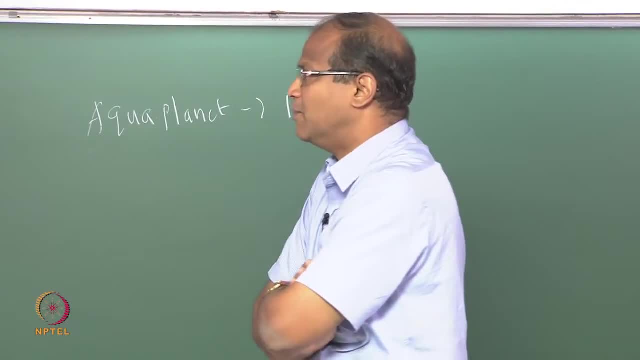 by the water. the earth's crust is relatively thin but dense. The plates of the earth crust are relatively thin, but the plates of the earth crust are moving away from one another. the new crust is formed at the spreading edges As the lava. 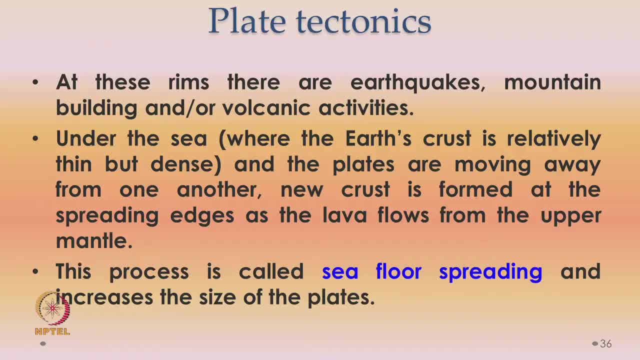 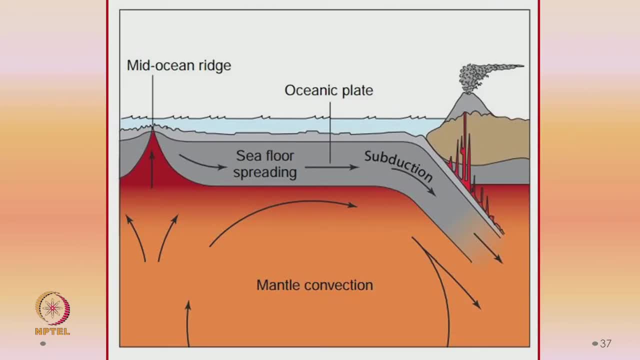 flows. I will show you- it will become more clear with the picture- as the lava flows from the upper mantle. So this process is actually called the sea floor spreading and increases the size of the plates. ok, So I will give this presentation to this, no need. 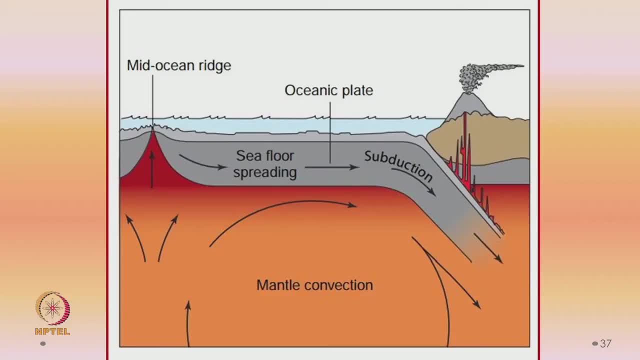 to copy this. So there is a oceanic plate. So I explain this concept. So there is a mantle, So there is a mantle convection which is taking place. So this is the ocean. So here we have a oceanic plate and there is a sea floor. 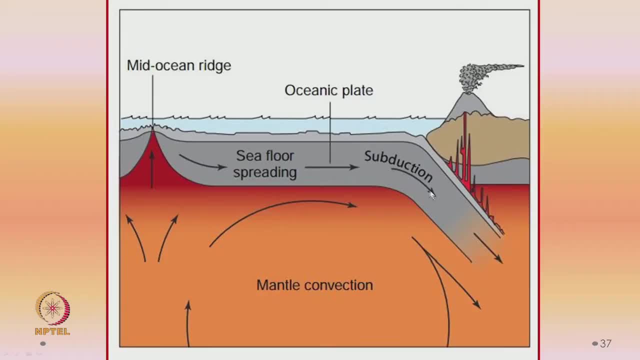 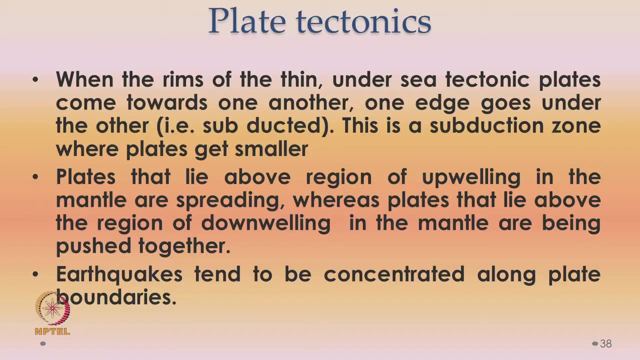 So there is a sea floor spreading and there is a subduction where this plate is just sucked. it goes into this. ok, When the rims of the thin undersea tectonic plates come towards one another, one edge goes under the other one edge goes under. 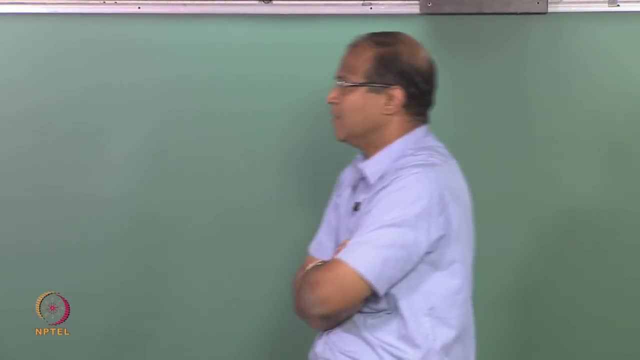 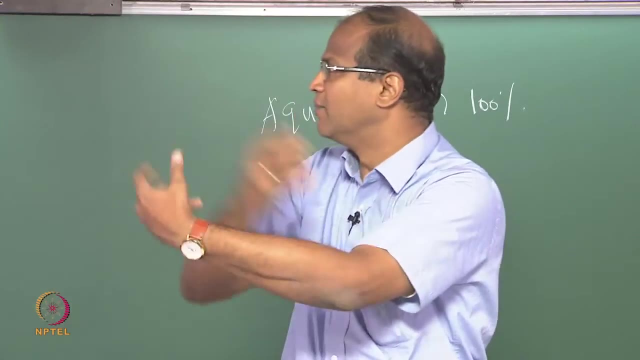 the other. This is called subduction, where the plate gets smaller Plates that lie above the region of upwelling in the upwelling. upwelling is the region where from the mantle, that convection, something is going up. they are spreading, So somewhere it is spreading. 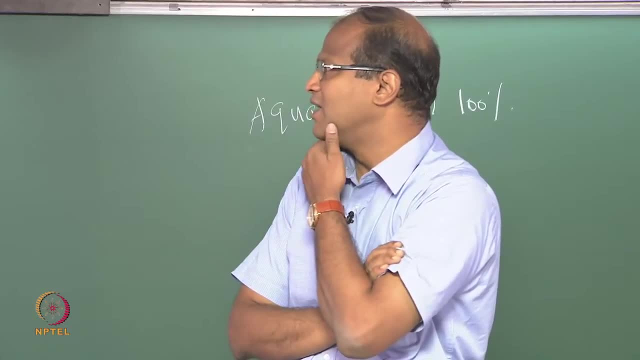 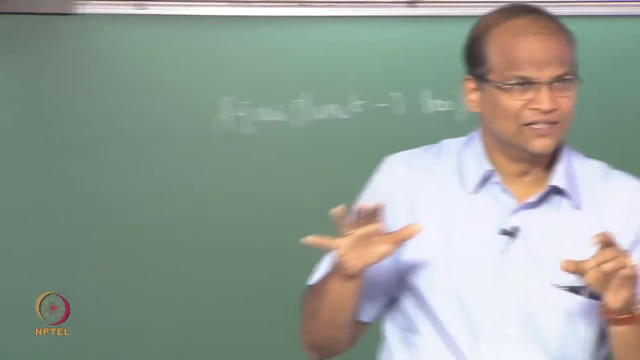 where it is sub subducting, and so on. So, whereas plates that lie above the region of downwelling are being pushed together, So which means, in slowly but surely, the shape and size of the continents is changing, Some geological activities taking place below. 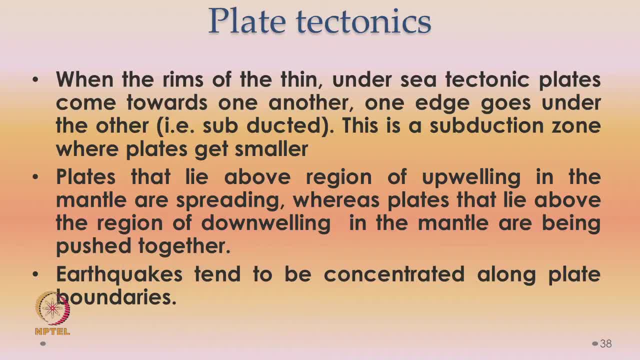 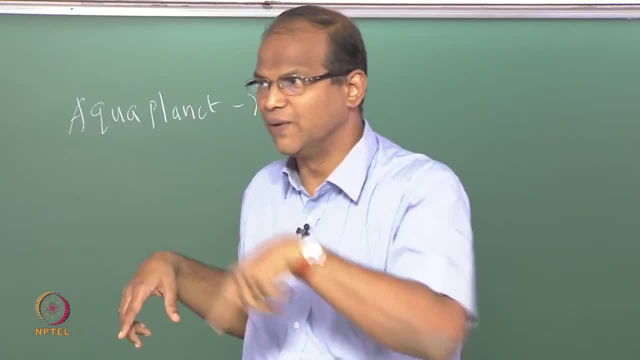 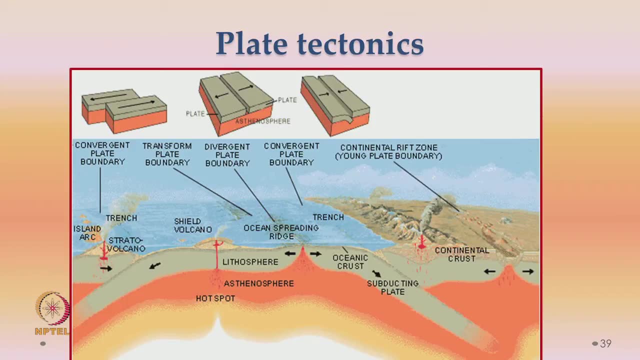 right. So earthquakes tend to be concentrated along the plate boundaries. Wherever there are, there is an interface between the various plates. you can actually see that the fault lines and the earthquakes are taking place along this. You must have- somebody, must have taught you this before right. So this is a picture where the left side 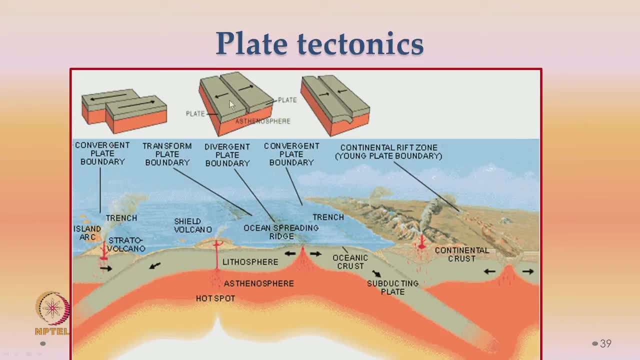 it says there is a shear between the two plates. here the two plates are moving apart. here the two plates are moving towards each other. So you can see hot spots, lithosphere. So this is just a overview, right? So there is something called convergent plate boundary. 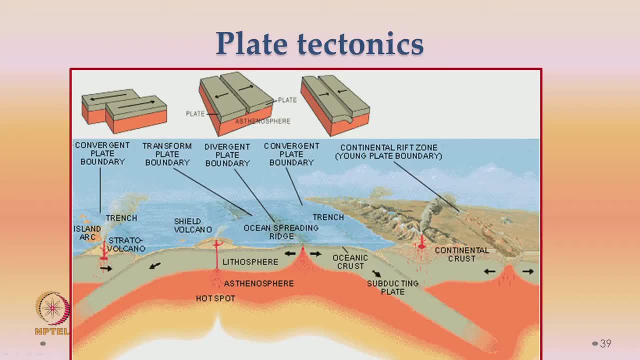 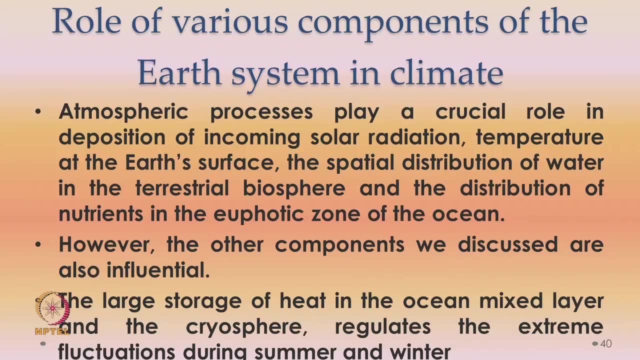 divergent plate boundary. Let us not get into all this detail, because our goal is to study atmosphere. ok, This is just to just to give a overview. all right, I will give you this picture. ok, What is the now? summing up the role of various components of the earth system. What I want: 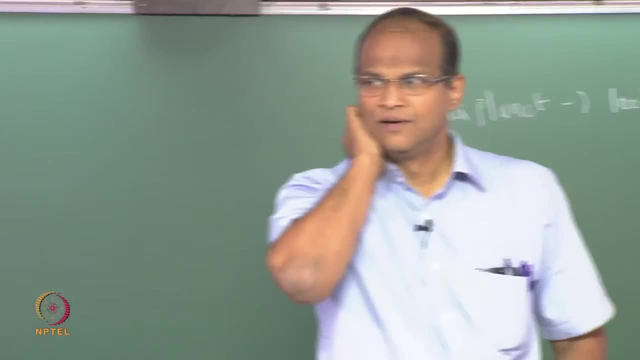 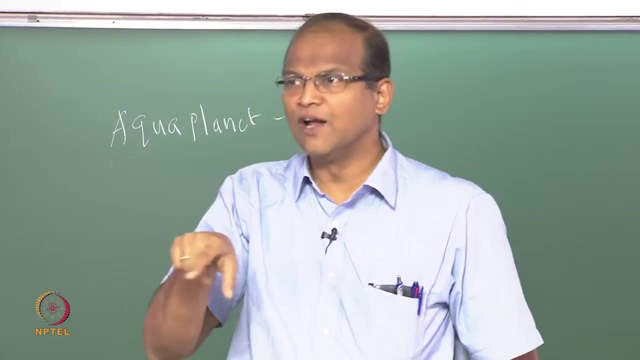 to say is: the atmosphere is indeed the most important. ok, The atmosphere is very important in deciding the earth's climate, but the atmosphere is not the only thing in deciding the earth's climate. That is what we understood by studying, by studying this chapter 2, where we looked. 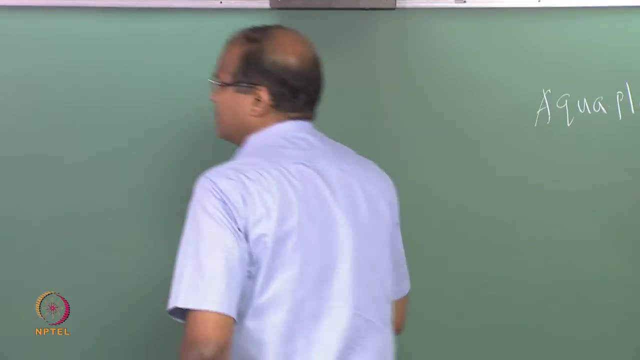 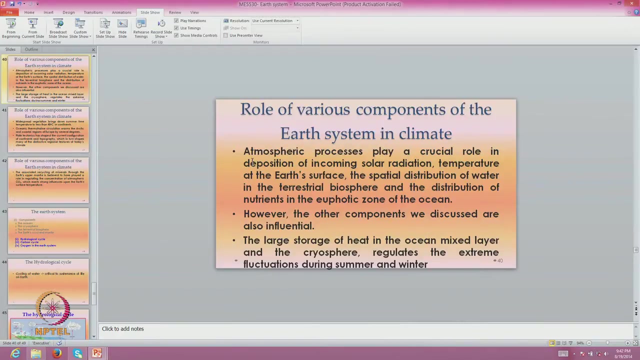 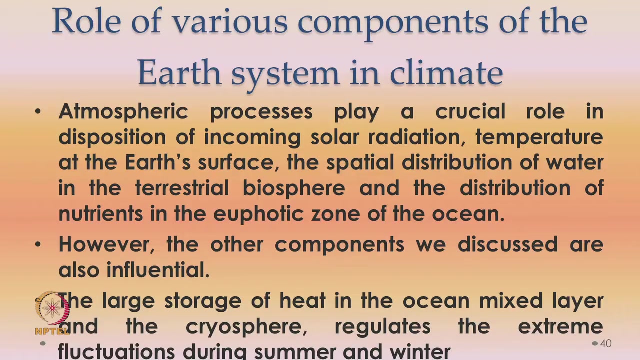 at all the other players right. So let us summarize: atmospheric processes play a crucial role in the- not deposition, ok- In the disposition of incoming solar radiation, the disposition of the temperature of the earth's surface, the special distribution of water in the atmosphere, in the terrestrial. 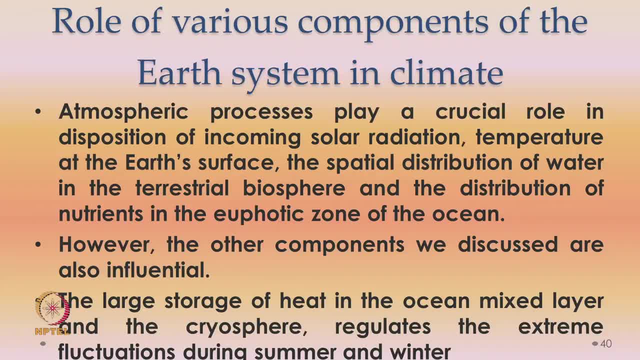 biosphere and the distribution of nutrients in the euphotic zone. So no doubt all these things are controlled by the atmosphere. but apart from that, there are other things. What are these other things? The role of other component is also influential, For example. 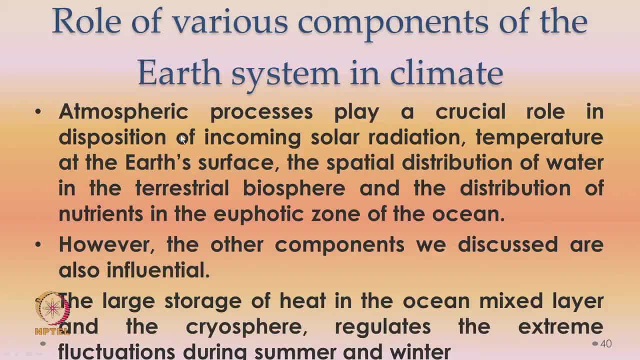 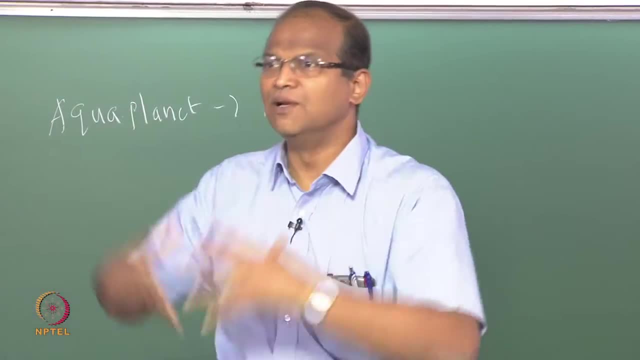 The large storage of heat in the ocean mix layer and the cryosphere regulates the extremes in the weather. ok, It extremes the fluctuations during winter and summer because there is so much of MCP, delta T. there is a thermal inertia associated with this. all right, 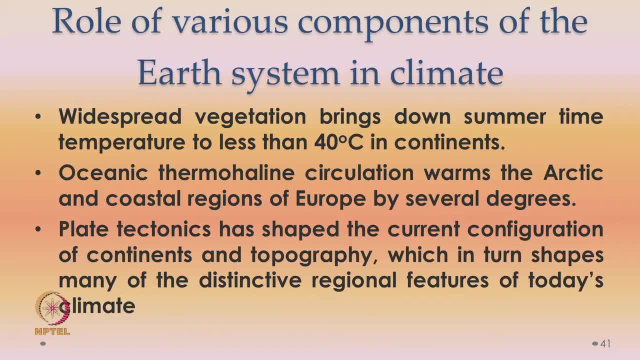 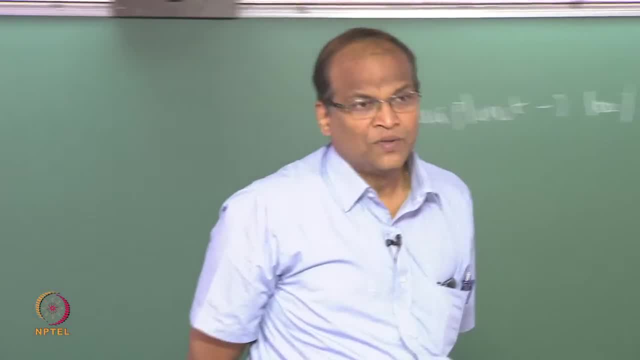 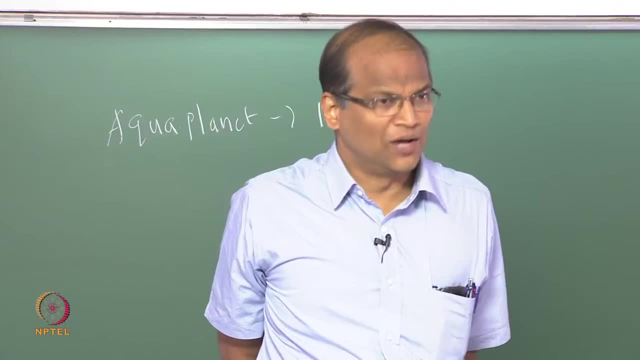 Wide spread vegetation brings down the summer temperatures to less than 40 degrees in the continents. otherwise the summer temperature would have been much higher, all right. Point number 3, the oceanic thermohaline circulation which is occurring because of differences in temperature and salinity. that is why it is called thermohaline convection, if you recall. 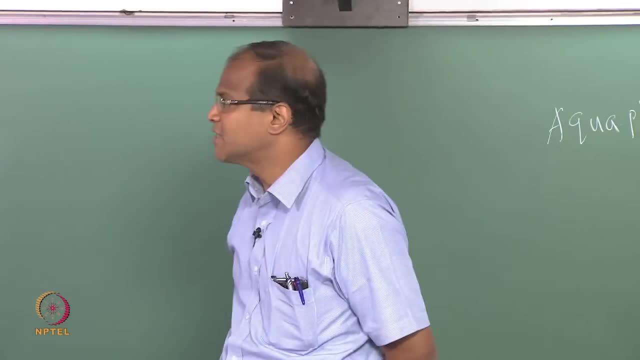 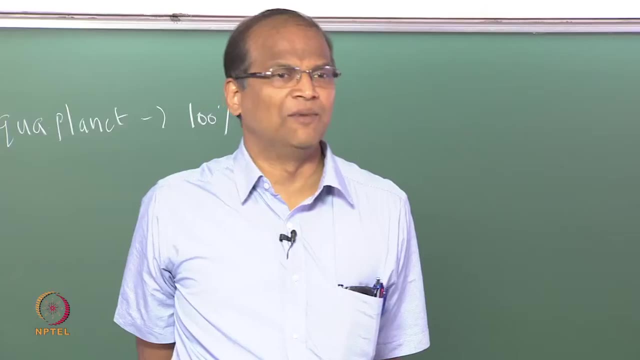 So the oceanic thermohaline circulation. it warms actually the Arctic region and the coastal zone of Europe by several degrees. that is why Europe is very, very has a very, very habitable climate, Otherwise for 50 degrees. 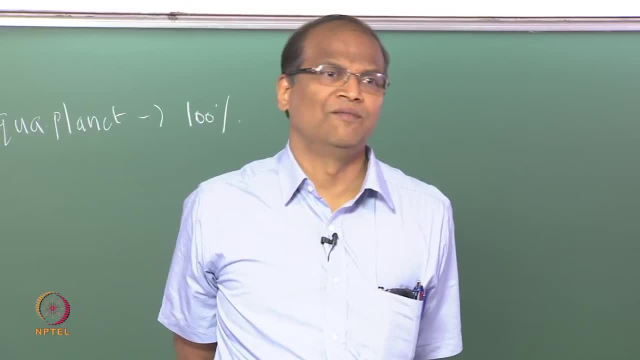 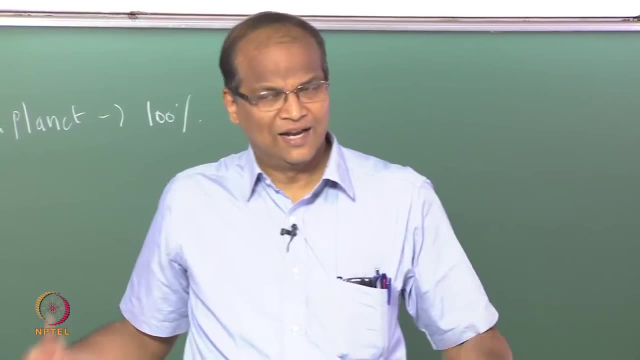 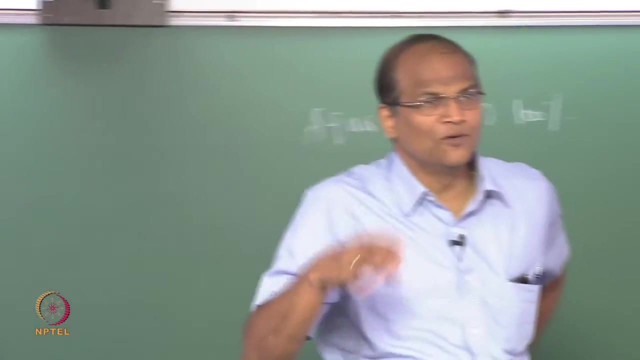 London, Hamburg, all these places should have been minus 40,, minus 50, highly unlivable. So the ocean currents are making a are making, are having a big role in making Europe so habitable. right. That is why lot of population is concentrated in Europe. Europe is a the continent developed. 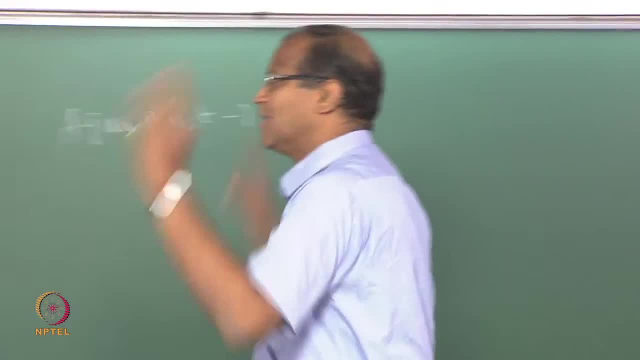 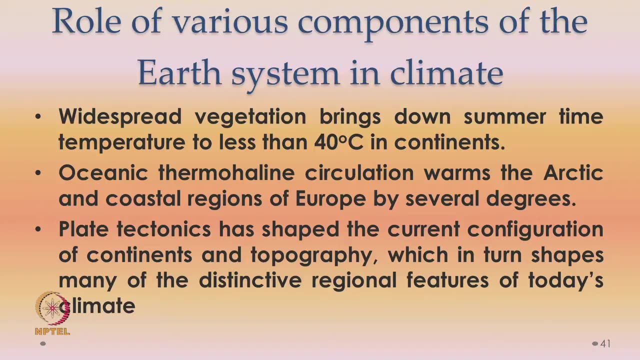 first, much before them. ok Now, plate tectonics, which we discussed in today's class, has shaped the current configuration of continents and topography And somehow Most of the continents are in the Northern Hemisphere. we do not know why. Most of the continents are in the Northern Hemisphere and Northern Hemisphere appears. 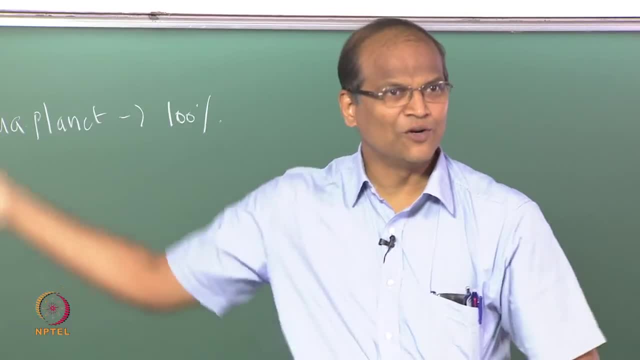 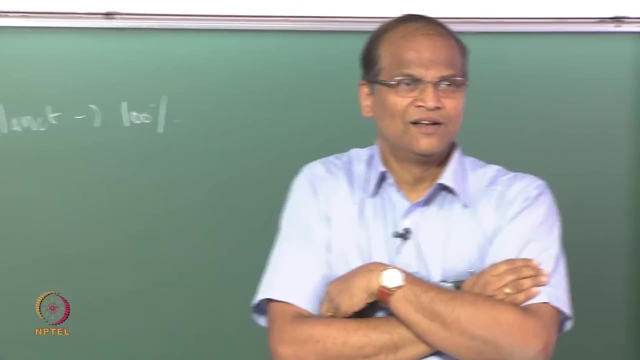 to be more developed. You can see that I showed in one of the pictures. also right, Northern Hemisphere is more developed. If you look at the GDP of Northern Hemisphere and Southern Hemisphere, there will be vast disparity. The only decent countries in the Southern Hemisphere- Australia, New Zealand, probably. 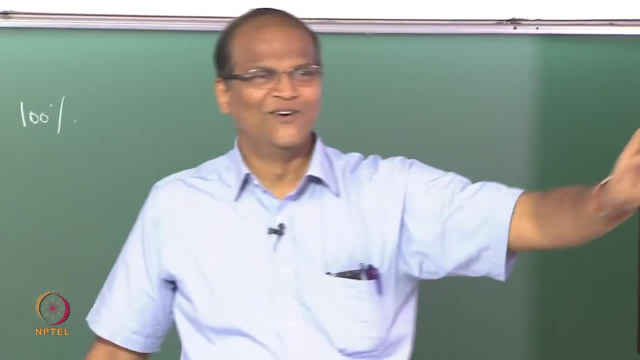 Brazil, now South Africa, ok, most of them, ok. So if you see now Southern Hemisphere, we do not know, We do not know. Ok, Singapore, and all is still 0 degrees. right, Singapore is still equator. 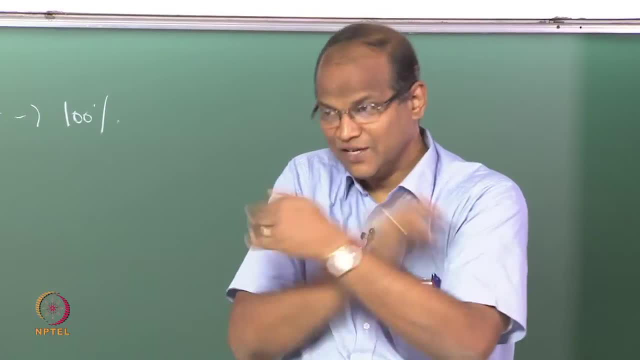 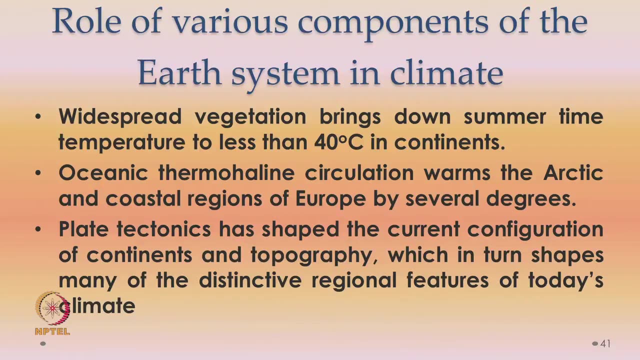 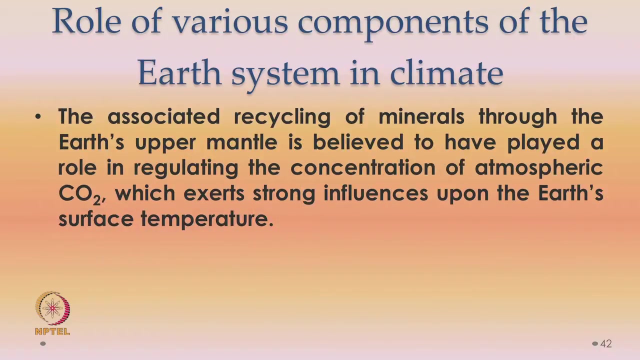 So, South, we do not have many countries which are economically advanced. ok, So plate tectonics have shaped the current configuration of continents and their topography, which in turn, shows many of the distinctive regional features of today's climate. ok, Finally, through the earth's crust and mantle, because of this continent, because of this, 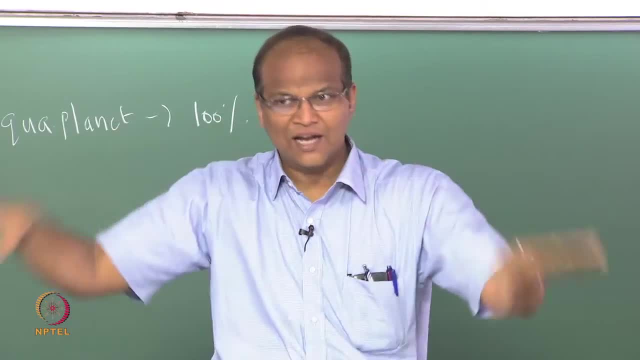 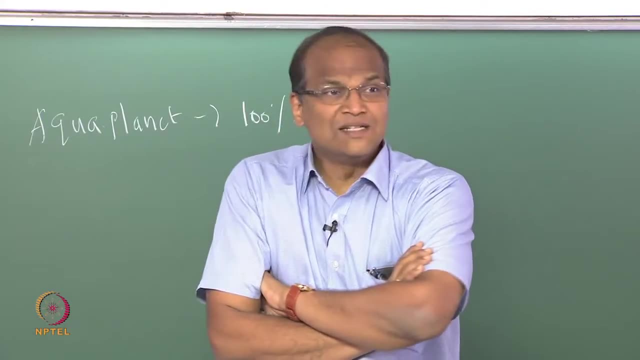 plate, tectonics and all these plates coming together moving apart and all that, and this mantle convection and all that. There is a recycling of minerals through the upper earth's upper mantle and this is believed to have played a major role in the concentration of atmospheric carbon dioxide, which exerts 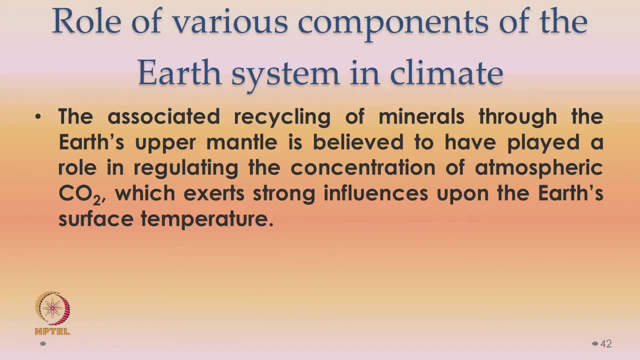 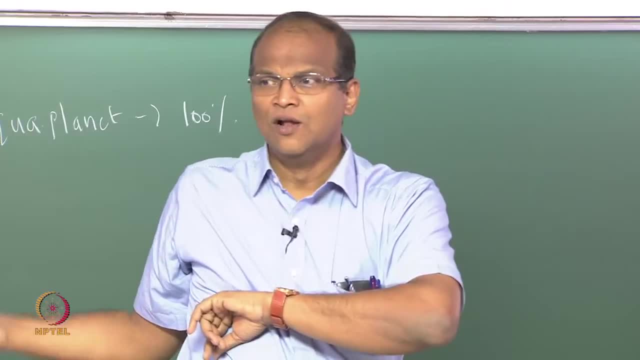 strong influences upon the earth's surface temperature. In fact, the original big bang theory. originally, when earth was formed, there is no oxygen. We will see that Now we will have to find out what is the source of oxygen in the earth. 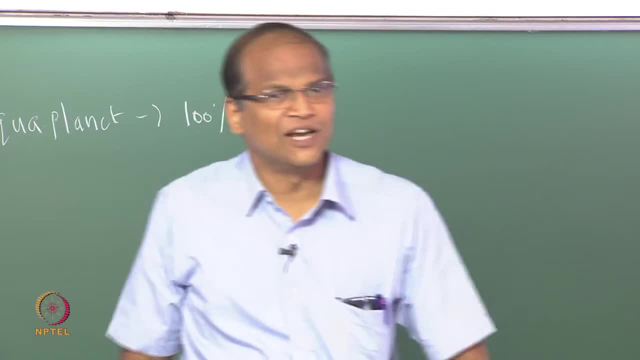 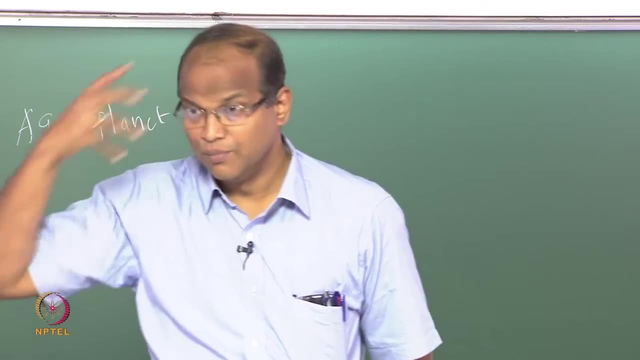 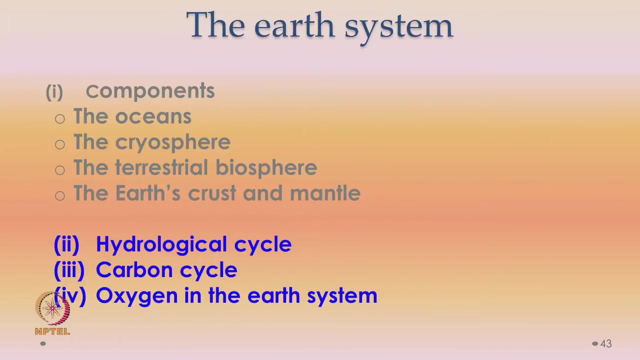 If you do in one of the subsequent classes, we will try to do an analysis and try to see what has resulted in the production of oxygen in earth. ok, But the oxygen has built up over a period of time, all right. Now, if you look at the earth system, E must be capital anyway, it does not matter. 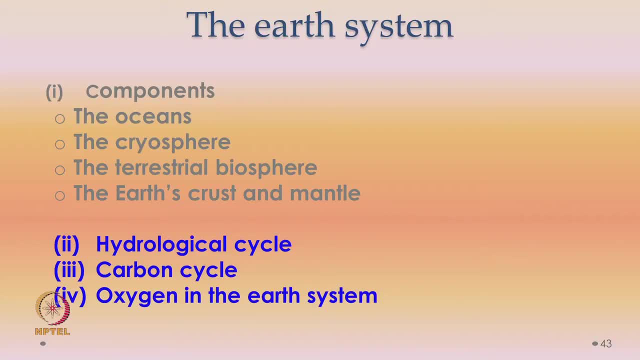 So the various components, the oceans, the cryosphere, the terrestrial biosphere, the earth's crust and mantle, which I have indicated in gray color, we have already considered so far. And now, if you recall, this was the first slide in the second chapter- 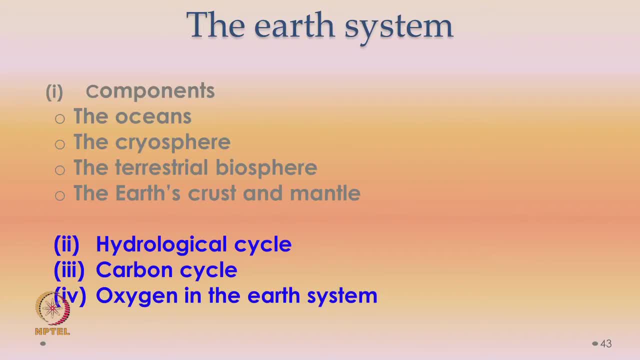 Now, if you recall, this was the first slide in the second chapter. Now, if you recall, this was the first slide in the second chapter. Part 1 was the components, part 2 is hydrological cycle, part 3 is carbon cycle and part 4 is. 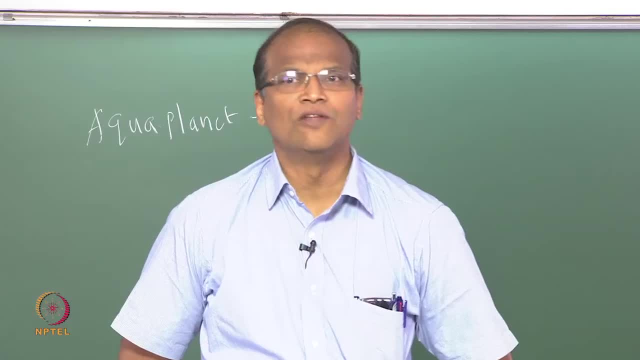 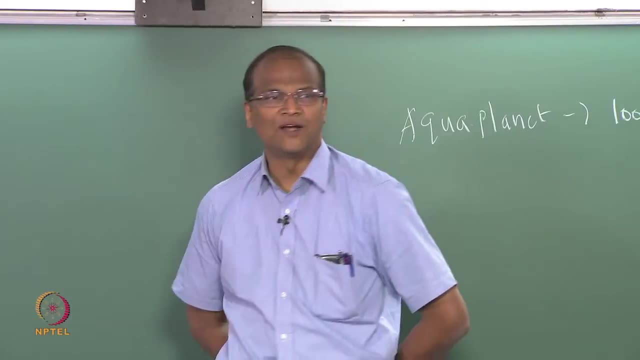 oxygen in the earth system. We need to study each of this. After we complete all the four parts, I promise that we will get into atmospheric thermodynamics. So part 1 is now over. now we will have to go to part 2, where we look at the hydrological 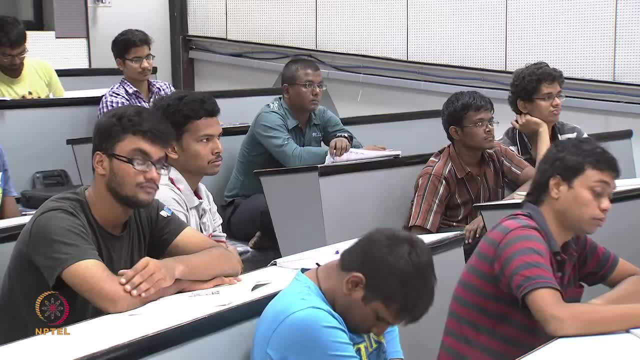 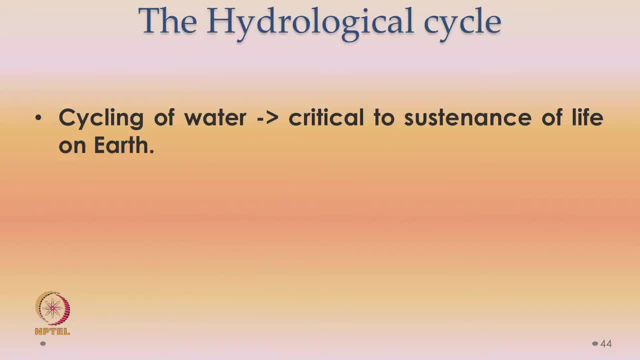 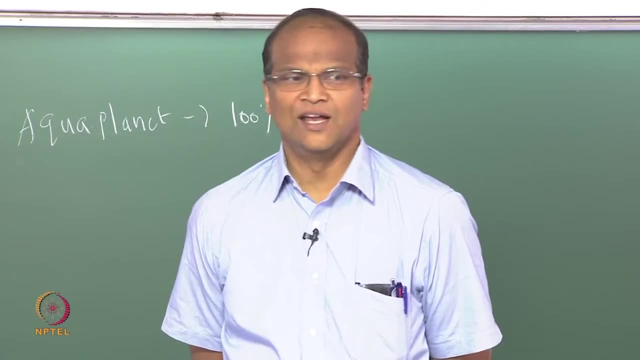 cycle. Any doubts so far. The cycling of water hydrological cycle refers to the cycling of water Hydrological cycle, cycling of water. it is critical to the sustenance of life on earth, because water can exist as water vapor, water can exist as ice, water can exist as liquid. 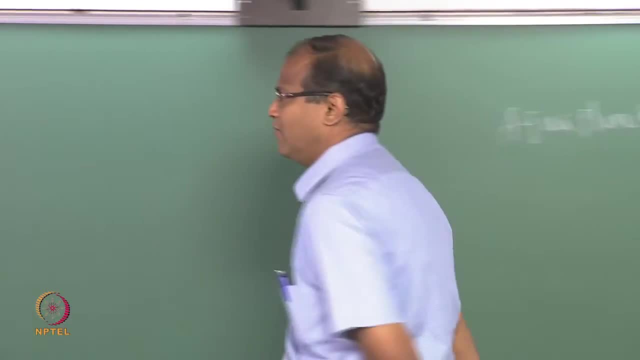 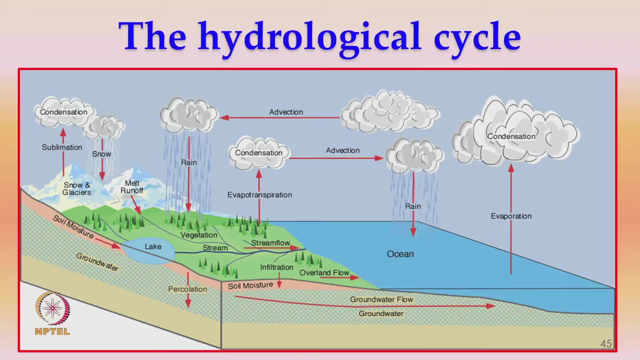 water itself. So it is critical to the sustenance of life on earth. there is no doubt about it. ok, This is. this picture is coming from your geography school days. right Now, let us look at it a little more carefully. 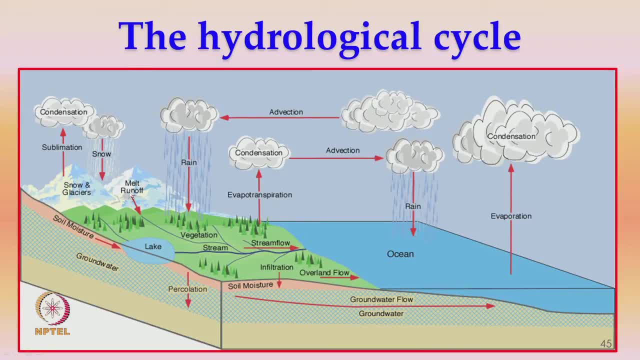 So this is the hydrological cycle, So hydrological cycle, So hydrological cycle. Where do we start? Where do we start? Ok, From the ocean. from the ocean, there is evaporation, then clouds, condensation, and it may not condense. 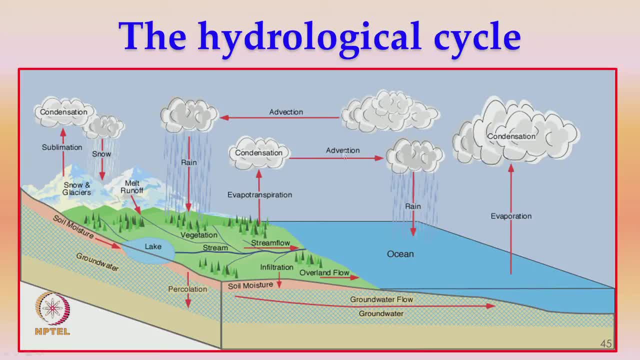 at the same place. by winds it may be transported, so this is called advection right, So there can be horizontal transport. it may rain elsewhere, and we are very happy. if it rains on the land, ok. So if it keeps on raining on the ocean, it is of no use to us. so it rain, and who brings? 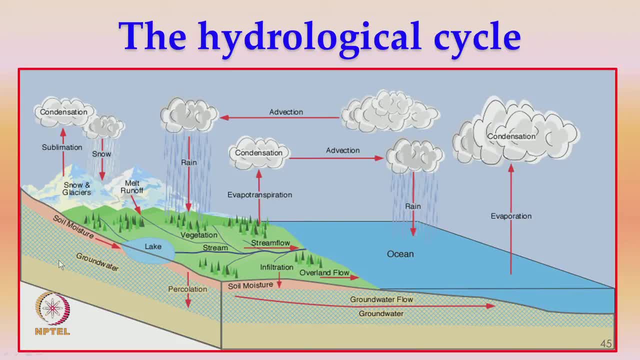 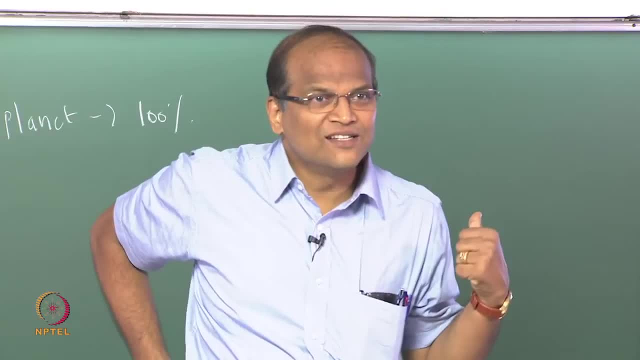 these clouds to the? Who brings these clouds to the land? Winds, Winds, ok, Which are the most important winds. who which are bringing the clouds to the land? as far as India is concerned, North west monsoon. North west monsoon. South west monsoon It is also called. it is mausam actually, it is a modification of the word monsoon, So south west monsoon are also called as the Indian monsoon or the Indian summer monsoon, which cause heavy rain in JGAS, June, July, August, September. ok, 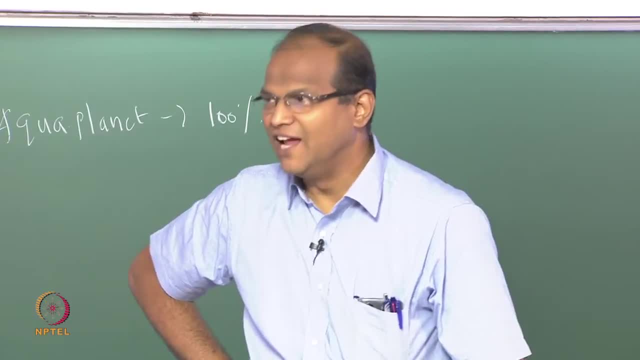 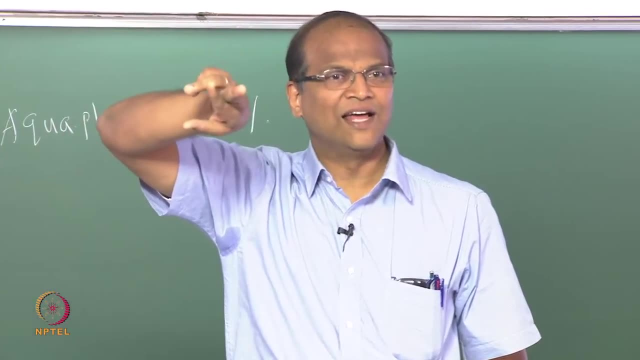 So we call JGAS rain. Now let us see JGAS rain. Now we are in A next S will come. after that it will stop. then the winds will reverse. that is called the retreating monsoon. then the direction will reverse and you will get. 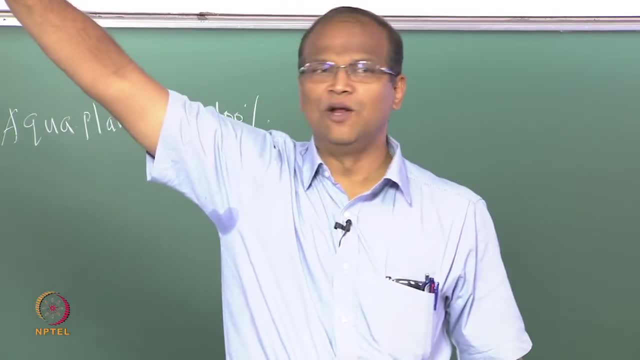 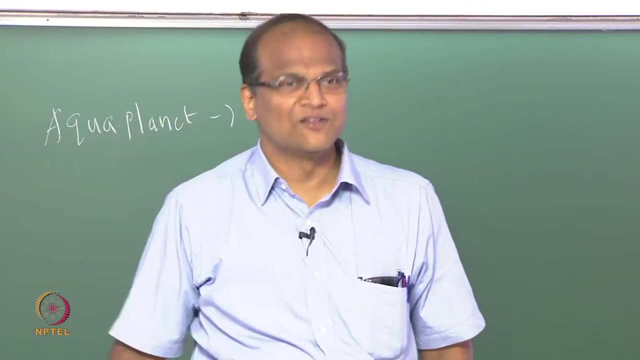 winds, from north east, from the cold Himalayas. it will, and then, because of the Coriolis component of the earth's rotation, it will be, it will basically take a turn. That is why all the cyclones heading towards Madras will then go to Andhra Pradesh or it. 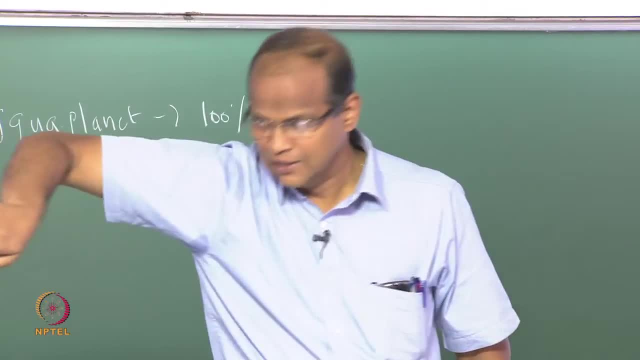 may go to Orissa and finally it may hit Bangladesh also. Have you seen that They? that is called re-curving. So it is a rotation, It is a re-curving. That re-curving can also take place, ok. 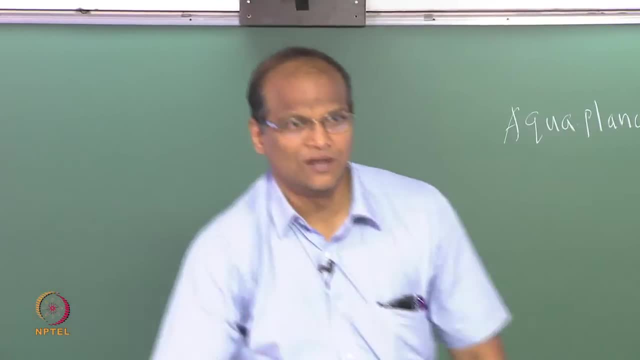 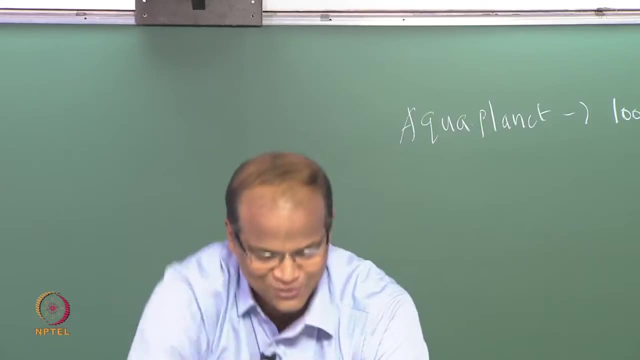 So winds are very, very important. ok, Why you right, Why you Bhagawan? That is what? hey, the very, the clouds have to come from the ocean. ok, so that it lands, it rains on land, then vegetation, evaporation and transpiration, ok, 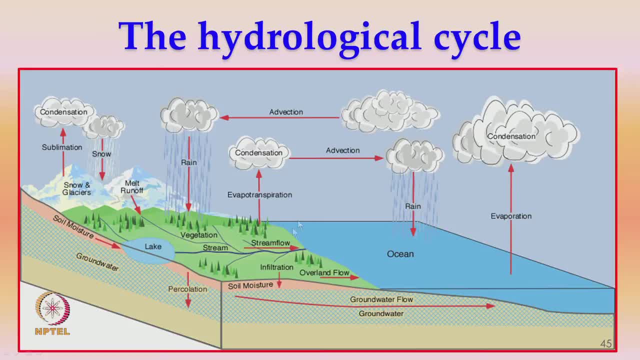 Then this evaporated transpiration again cause clouds, condensation advection. so this is there. Then this rain can come down, it can cause a stream flow and that rain. rain can directly go again into the ocean, ok, or it can do infiltration and become ground water. it can be stored. 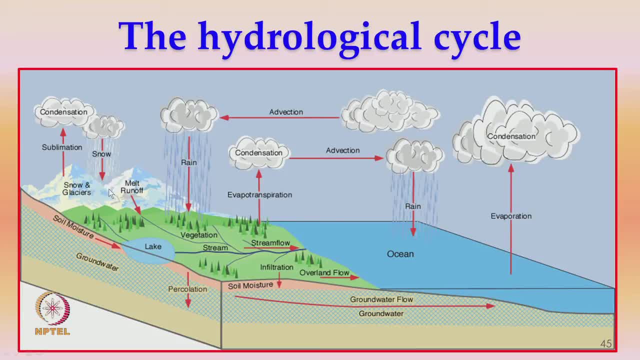 as ground water. Then you can also have snow and glacier, there is melting, and then big rivers are formed, like Himalaya and Ganga and Yamuna, and all that, and then you can have this, and then they go through the plains and finally they join the sea. 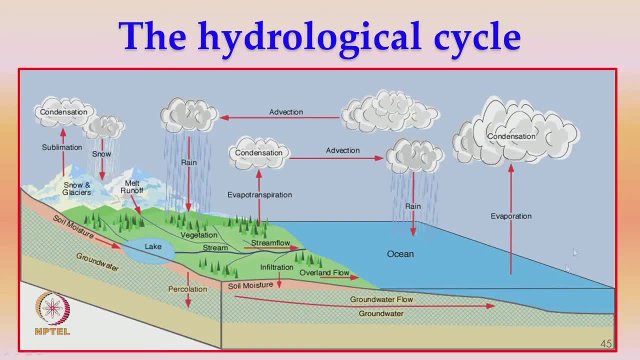 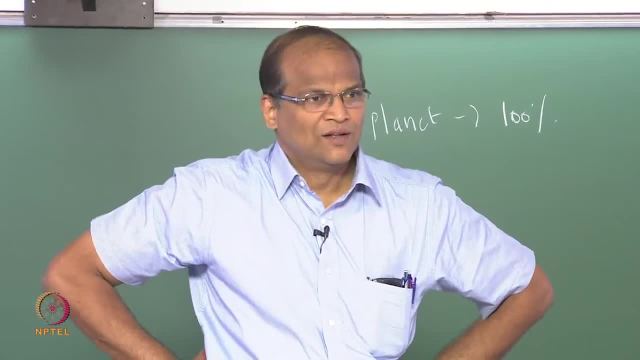 So this is basically the hydrological cycle, so each of this can be characterized. we can have mathematical equations for each of this and then model this over a limited region, or you can model it over regional scale, or you can model it over the whole earth scale. 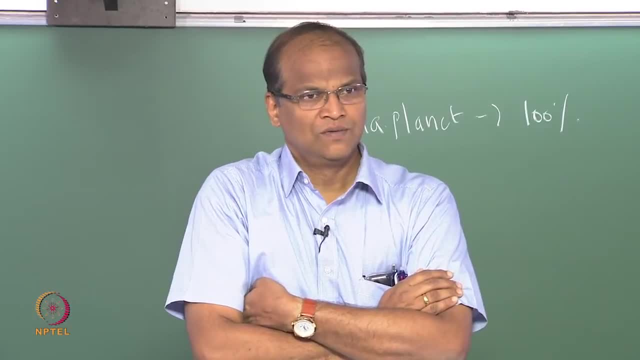 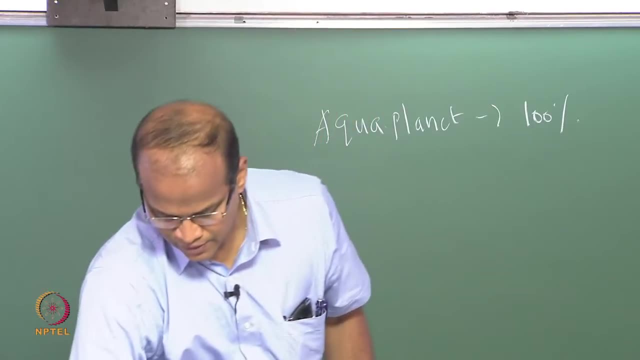 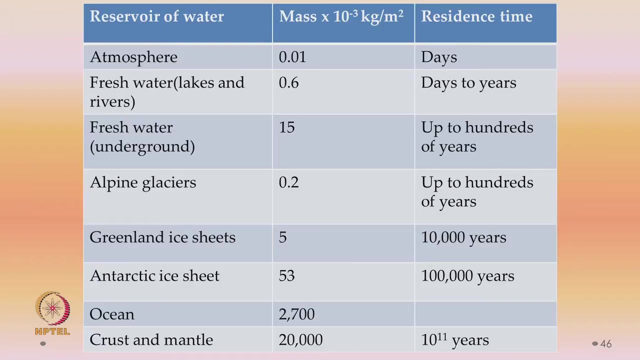 So this comes under the subject of hydrology, which is a big, which is a big subject in civil engineering. ok, Now please take down this figure, please take down this table. so this gives a. this gives a. this is a table which lists the major reservoirs of water and the reservoirs of 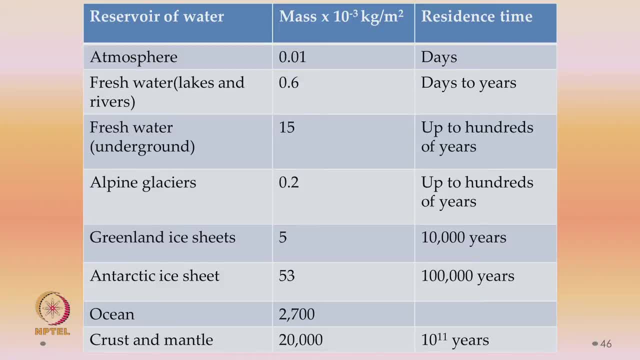 water in the earth and the mass into 10 to the power of minus 3 kilogram per meter cube. that means the mass is the value given in the table into 10 to the power of 3 kilogram per meter cube. is that ok? 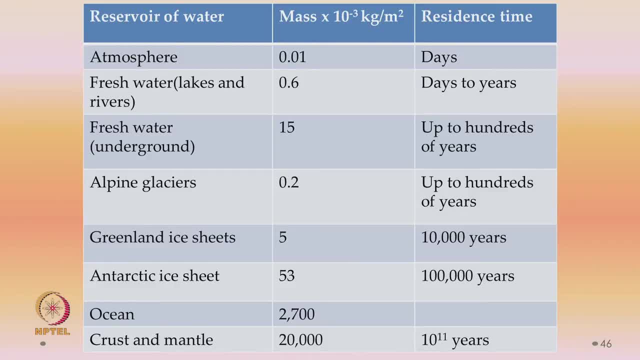 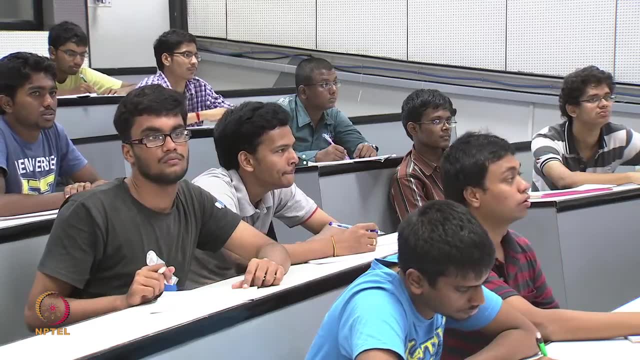 So this is basically mass density per meter square of surface area. whenever you want to find the actual mass, what do you do? Multiply by 4 pi Re square, where Re is 6370 kilometer or 6.37 into 10 to the power of. 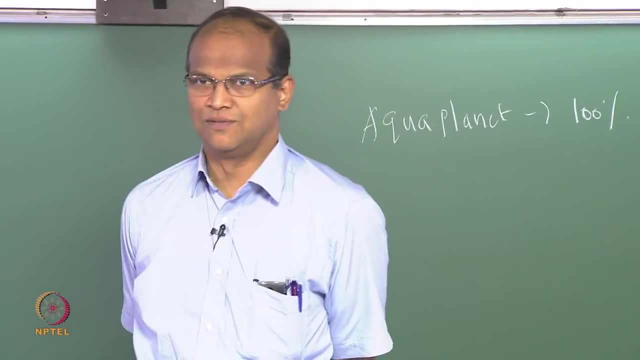 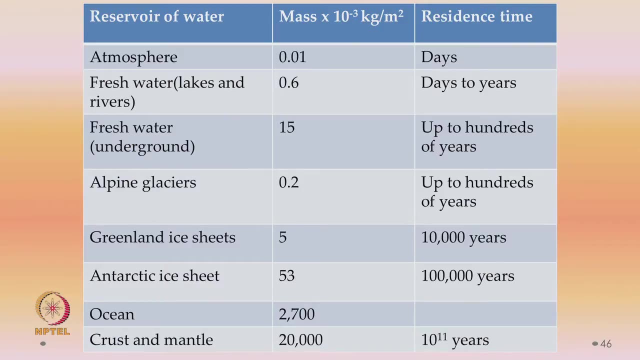 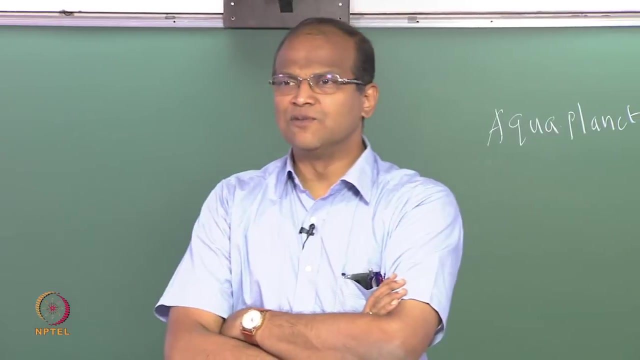 6 meters. this is a value which you should, you should not forget in this class. Ok, Atmosphere: 0.01 into 10 to the power of 3 kilogram per meter cube. the residence time is only days, that is, if you trace a particle, its life is only a day, few days. 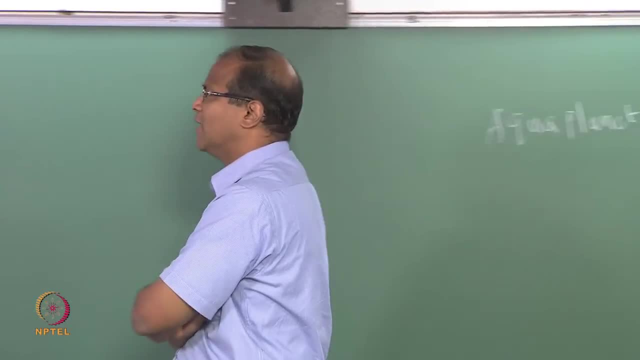 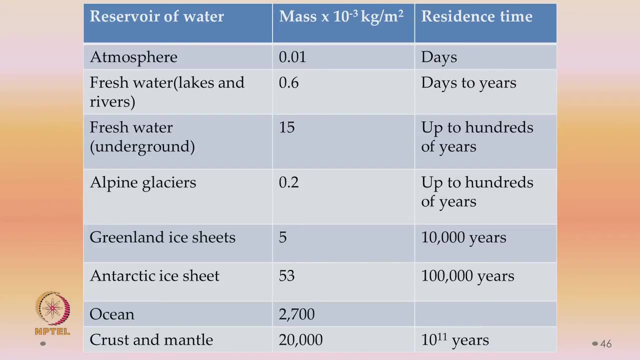 Then fresh water, lakes and rivers mass into 10 to the power. of minus. 3 is 0.6, the residence time is days to years. fresh water is 15,. alpine glaciers is 0.2.. Greenland is 0.2.. 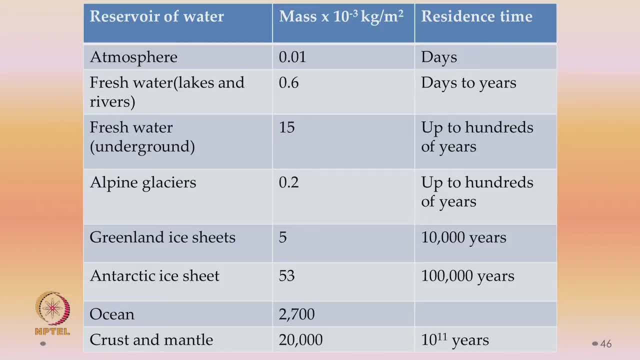 Greenland is 0.2.. Ok, Ice sheets, Ok. Ice sheets on Greenland is 5,. Antarctic ice sheet is 53,. the ocean is 2700 and the crust and mantle is 20,000,. ok, But you see what is the logic behind this table. how has this table been arranged? 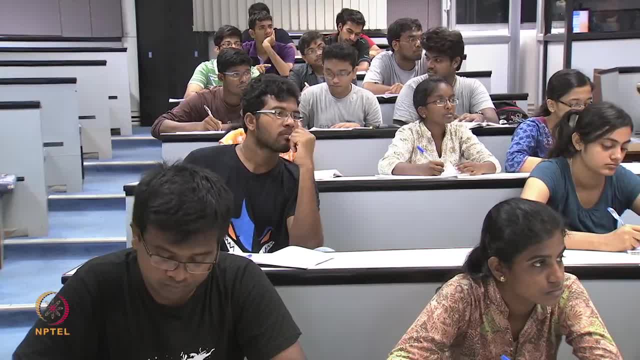 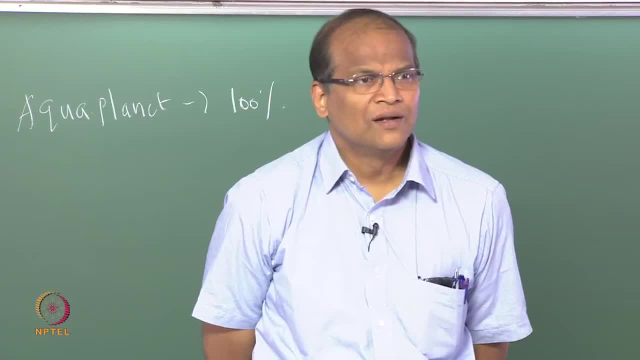 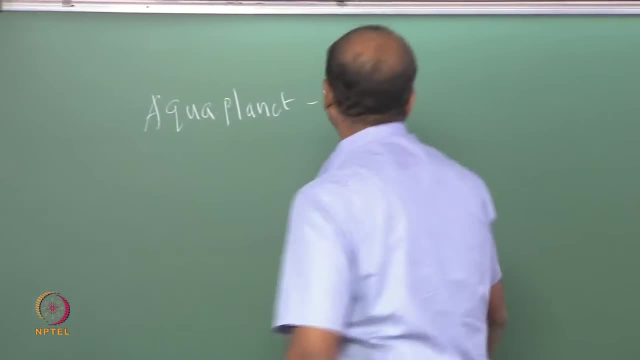 In the order of increasing. very good, it is arranged in the order of increasing residence time: Mantle, look at the mantle. The residence time is how much? Ok, So what is residence time? It is time. Let us assume this is the residence time. 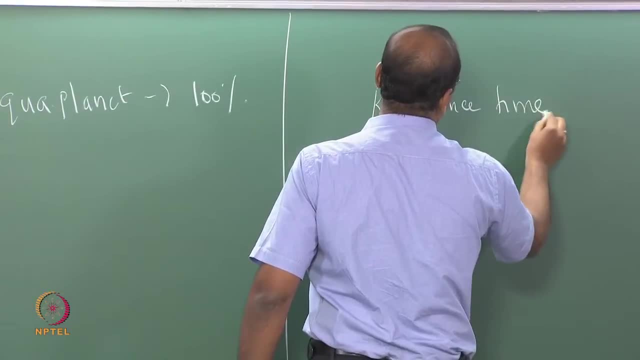 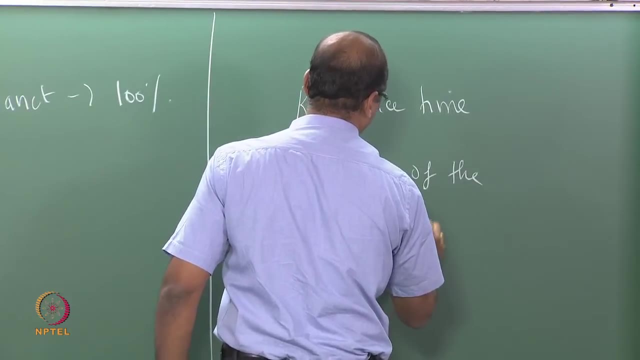 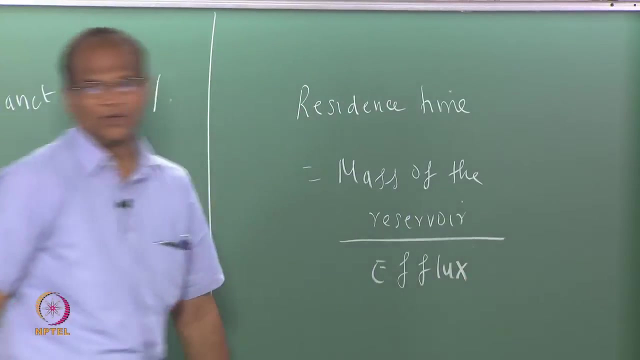 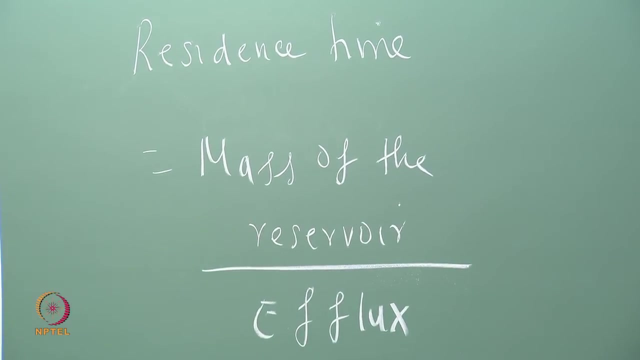 OK, So what is the residence time? It is 5, 4, 3, 4, 5,, 6,, 7,, 8,, 9,, 10, 11.. The residence time is the mass of the reservoir divided by the efflux. efflux. you are copying. 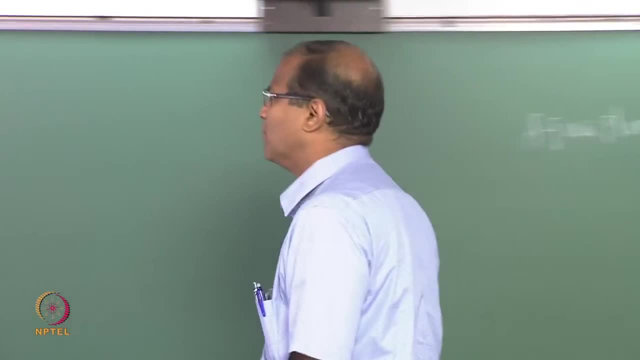 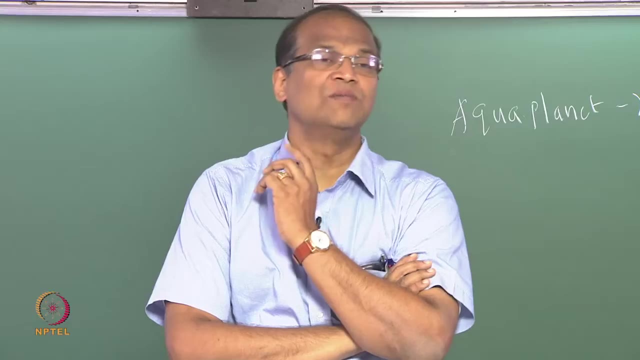 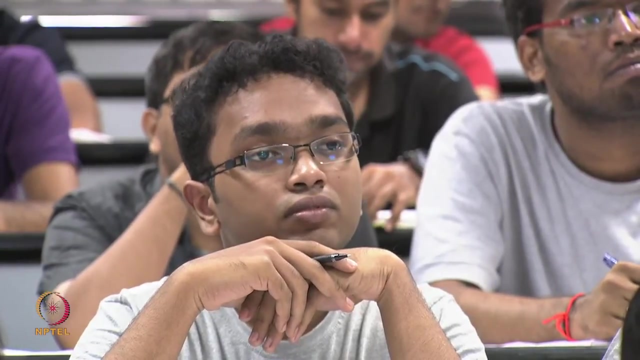 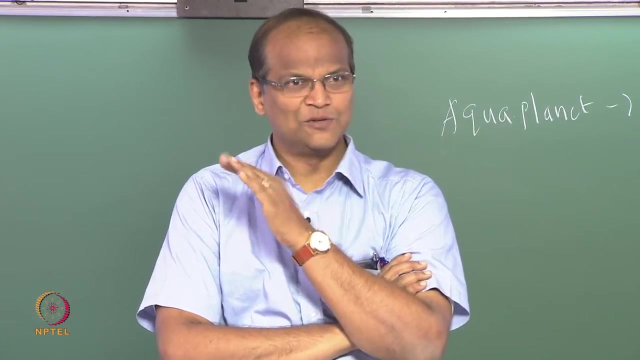 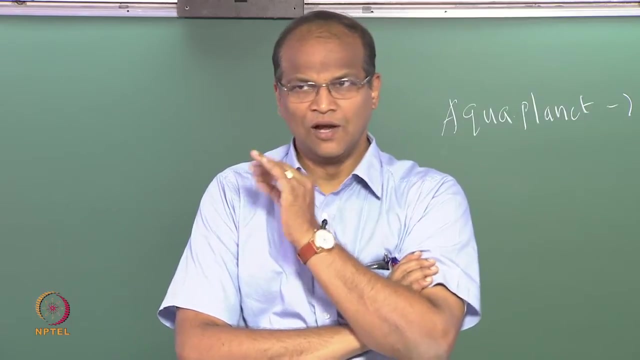 there. okay, then we will solve the problem. now say that again: no, no, that is okay. okay, ocean is basically. sometimes it can drop immediately, and how do we? everything comes back to the ocean. no, that is why it is left intentionally blank, I think, okay. 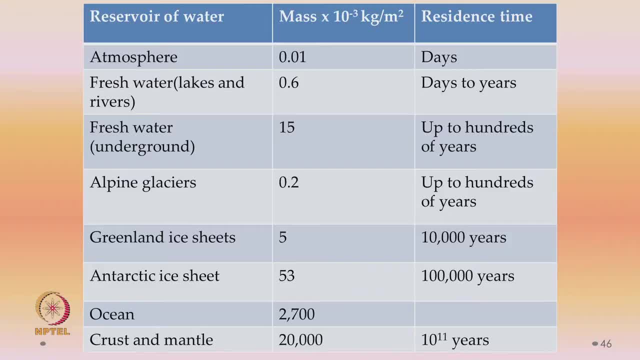 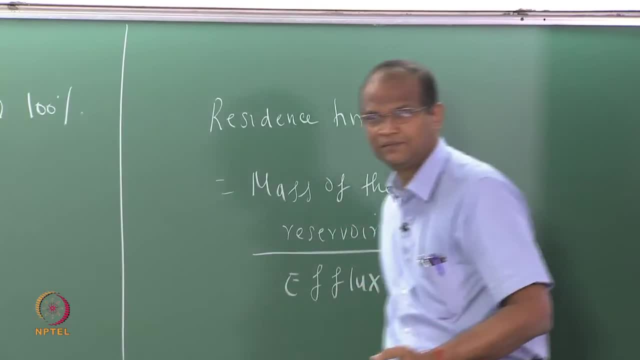 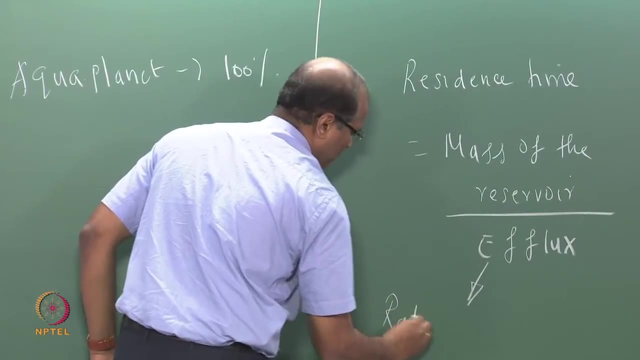 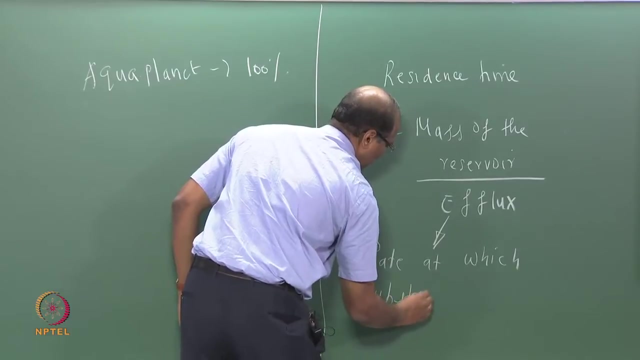 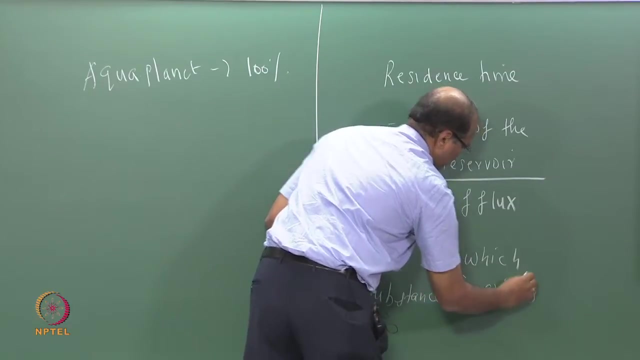 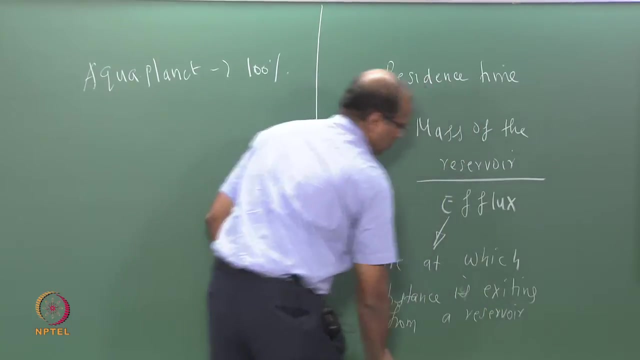 Now, what is the residence time in the table? the residence time is basically the mass of the reservoir divided by the efflux. efflux is the rate at which substance is exiting from the reservoir. okay, Okay, Okay, Okay. So the Okay. 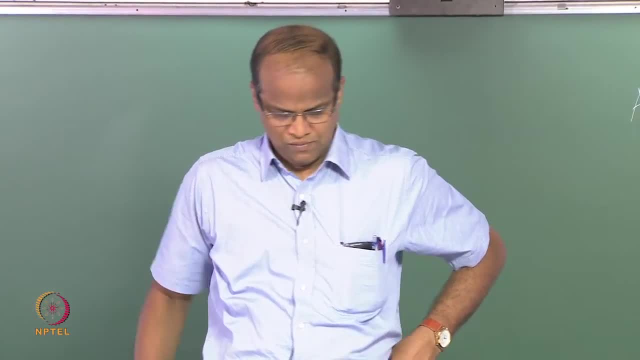 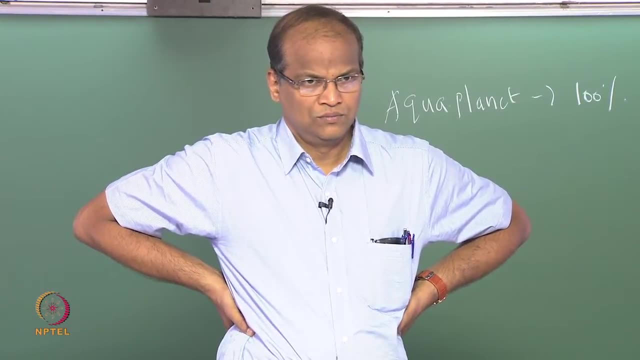 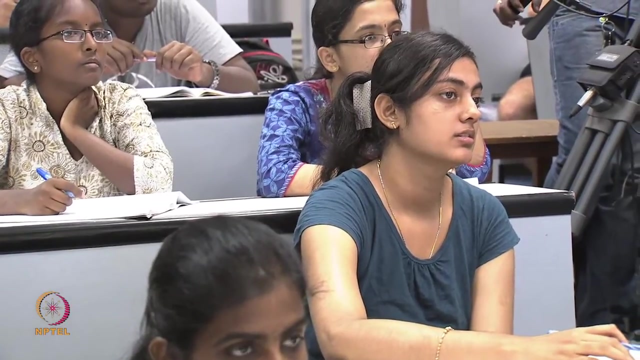 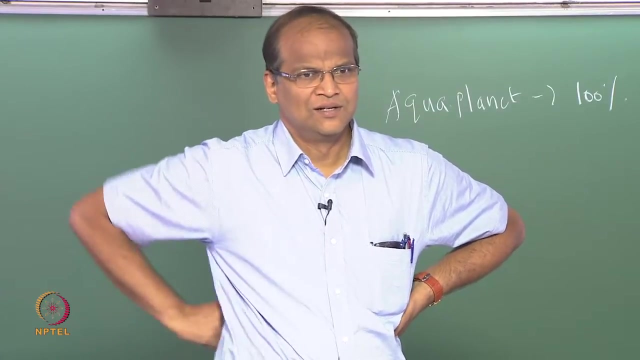 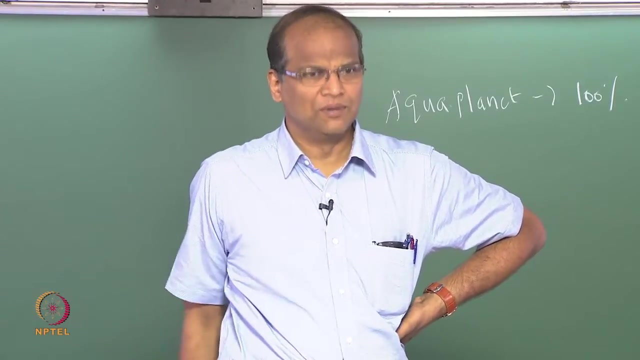 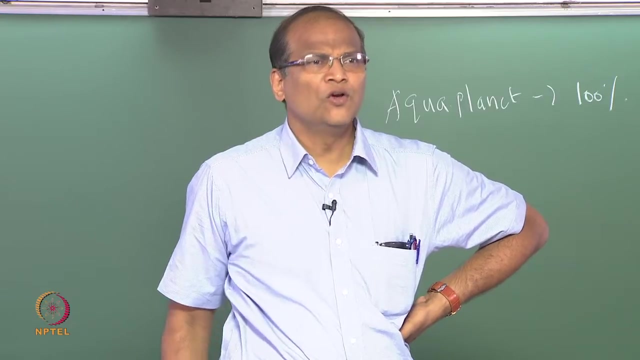 Okay, Okay, Say that again. these can. there are various estimates for that right, So you can have some proxies based on some analysis, some correct- there will be an error, man, but agreed upon by many people. This: you can use some dating and this thing: how much time it is. 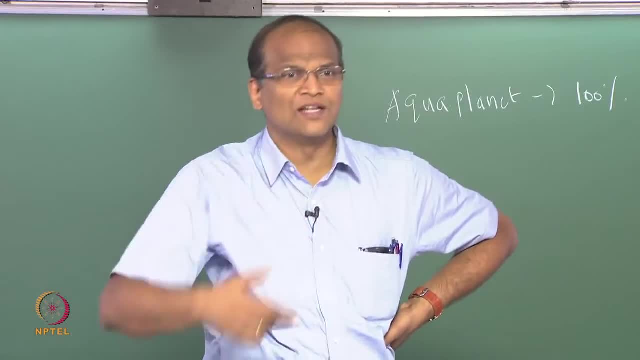 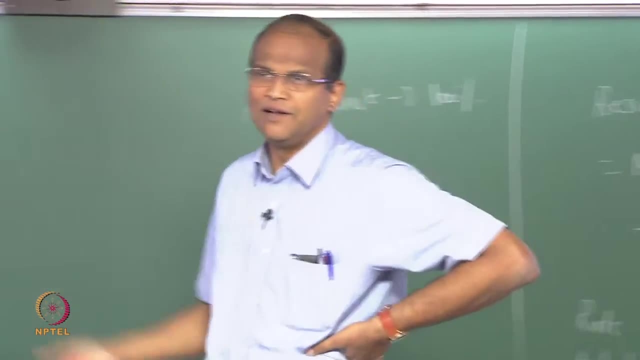 taken or some approximate calculations. just how do people say that big bang theory and all that is something like that. So some little bit of approximation will be there, but that, As you say, it is correct. it can be 10 to the power of 11 or 2 into 10 to the power. 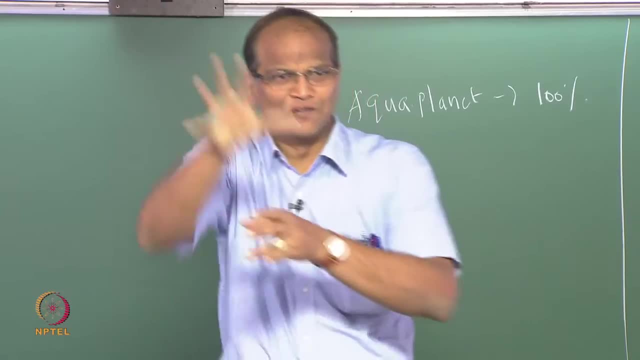 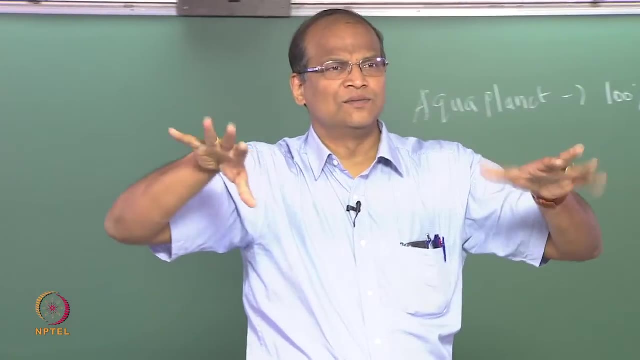 of 11, or 4 into 10 to the power of 11, or 5 into 10 to the power of 10, it is of that order. it is very huge. So what we can do is, I do not know, for example, as far as climate. 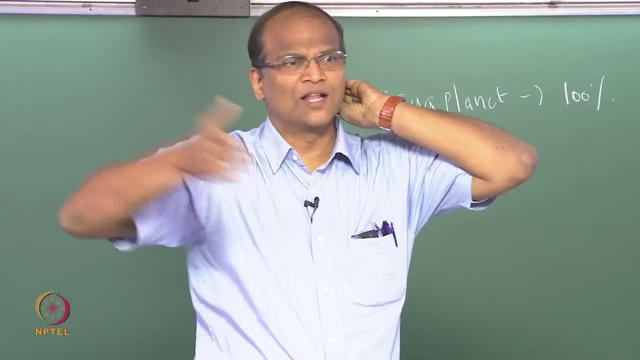 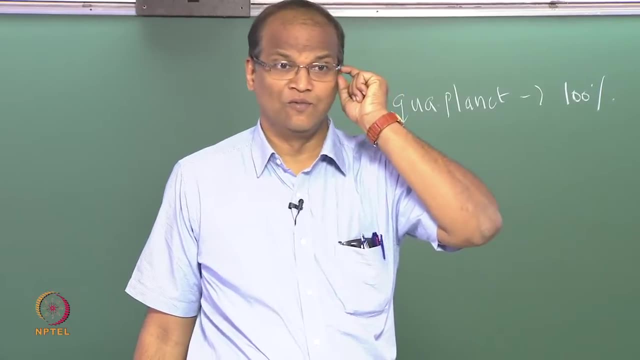 is concerned, the satellites are available only for 40, 50 years. So if you look at the change in pattern, we can extrapolate by a few 100 years, but for 10 to the power of 11 years. what data they have used, we do not know. 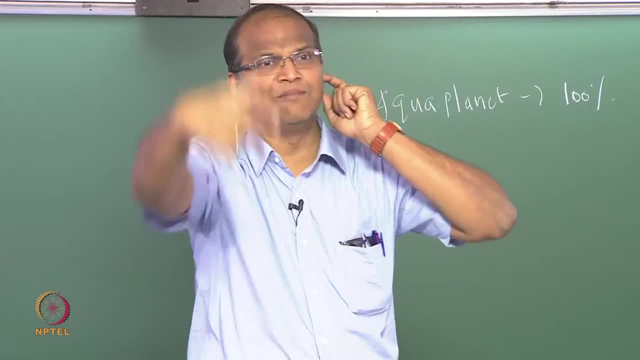 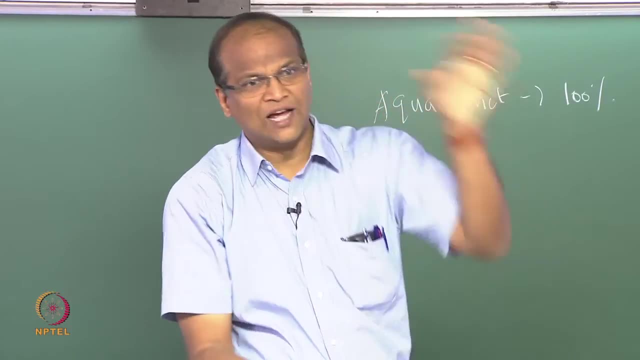 So we can do is we can do is we can go into Siberian, go deep down and get the ice sample at various heights, various depths. then you can correlate with the carbon dioxide and for a particular depth, So the ice is continuously forming on it. you can actually 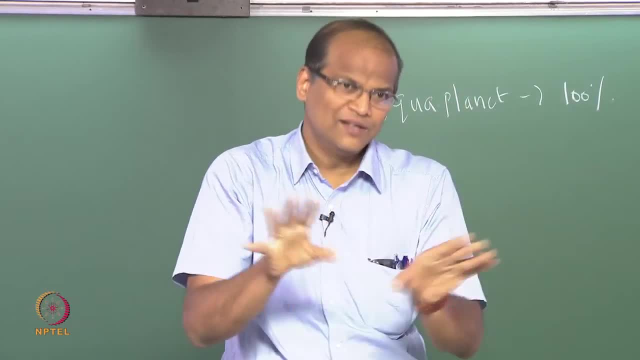 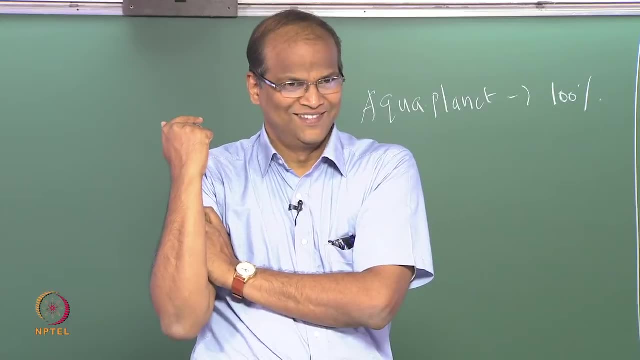 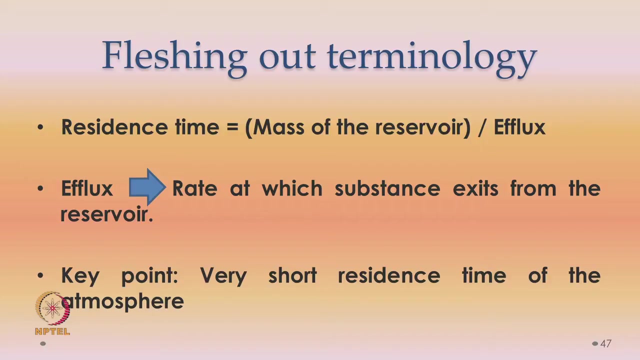 get the time. that is how they do, So it is a mixture of science plus some, So we can say it is a guesstimate. ok, let us flesh out some terminology. the residence time is the mass of the reservoir divided by the efflux. efflux is the rate at which substance exits. 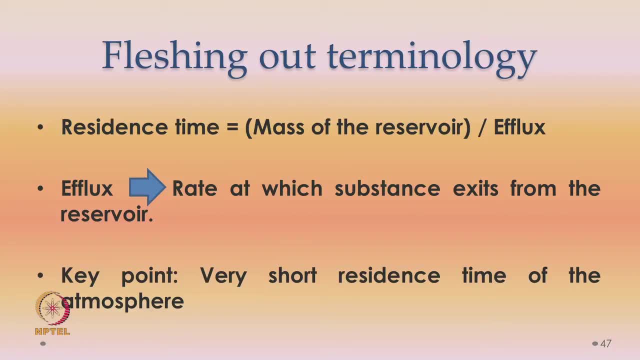 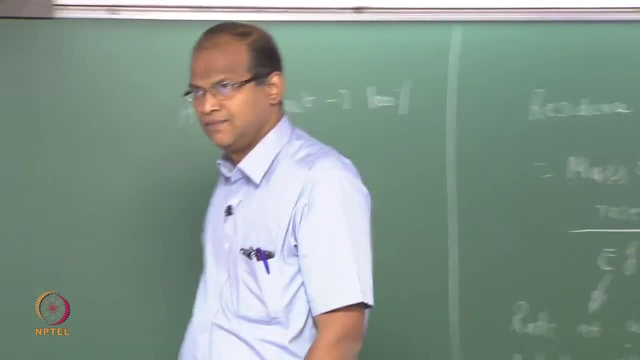 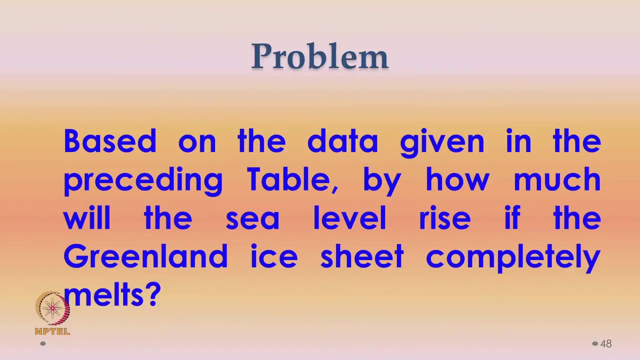 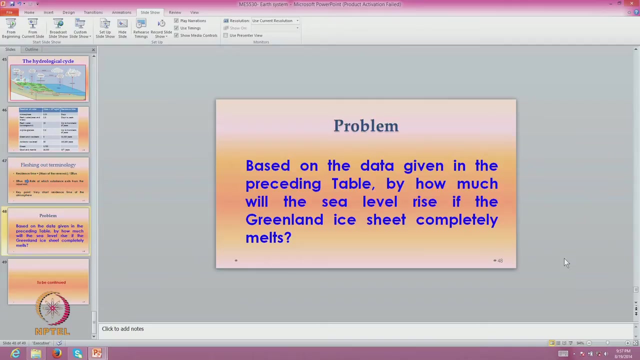 from the reservoir. The key point, what you have to understand from this previous table, is extremely short residence time. of the atmosphere of the order of few days, shall we move on to the next one Based on the data given? please take down this problem, problem number 7. is it? ok? then we will 7.. So I will just pack it. I want to. 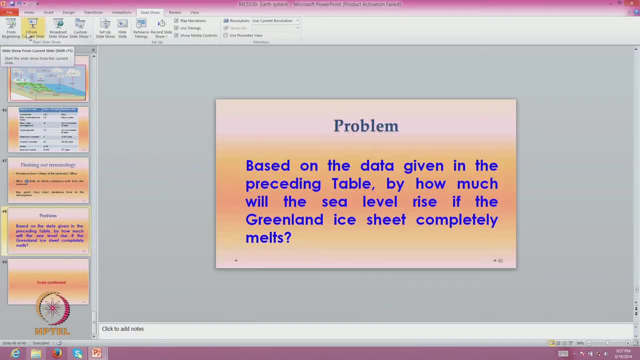 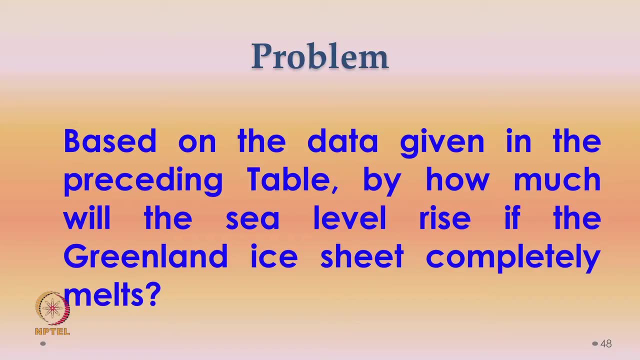 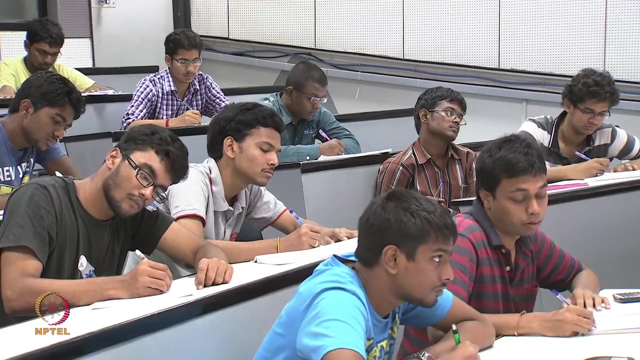 use the number. ok, what happened? ok, Please take down problem number 7 based on the data given in the preceding table. based on the data given in the preceding table, by how much will the sea level rise If the Greenland ice sheet completely melts? ok, so take a few minutes and 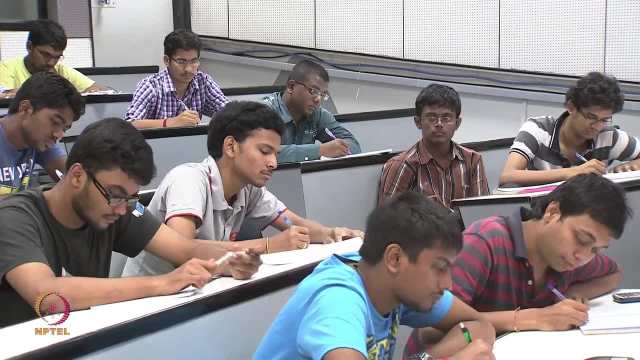 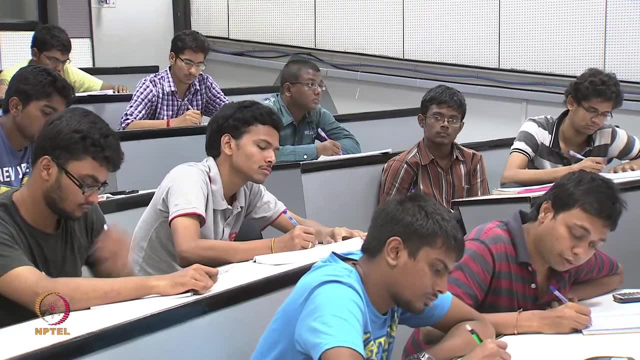 ok, So this is the problem number 7, ok, So this is the problem number 7,. ok, So this is the problem number 7, ok. Ok, So this is the problem number 7, ok. 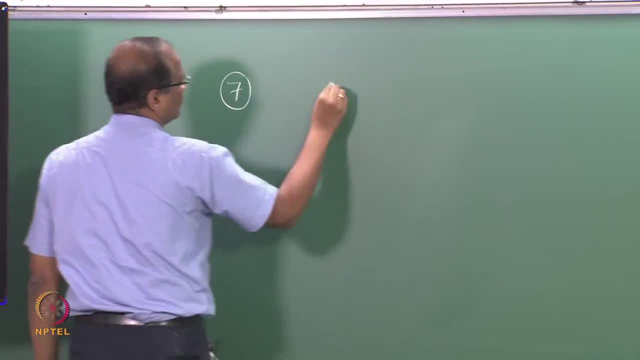 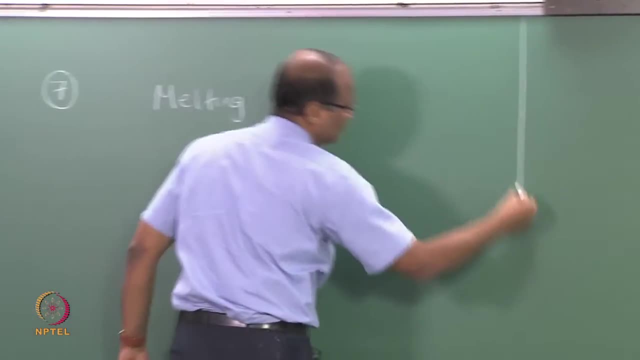 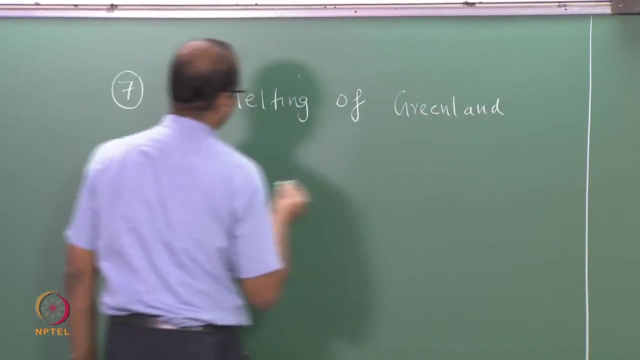 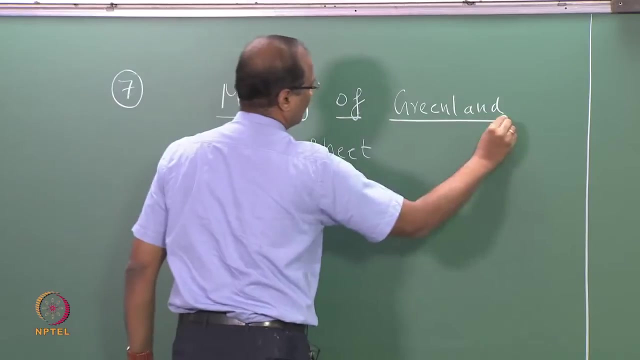 Ok, So this is the problem number 7. i have already shown. Ok, So this is the problem number 7, ok, Alright, so let's divide this by 2, i just do like this. ok, Ok, and again you can describe the one again. 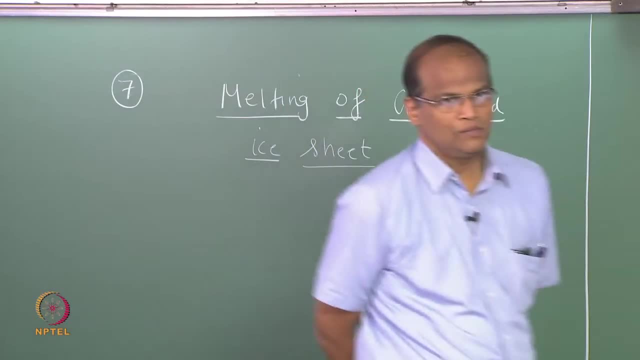 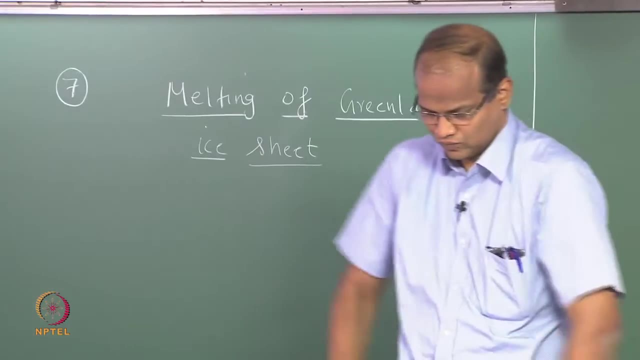 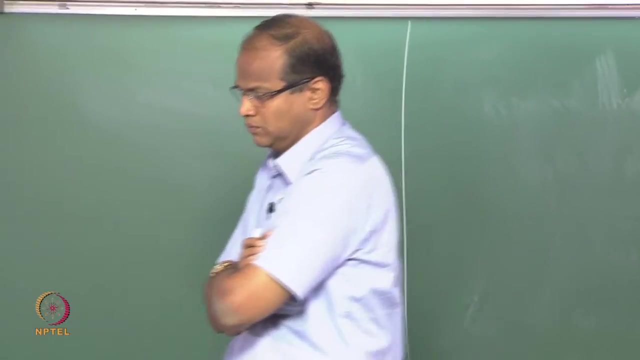 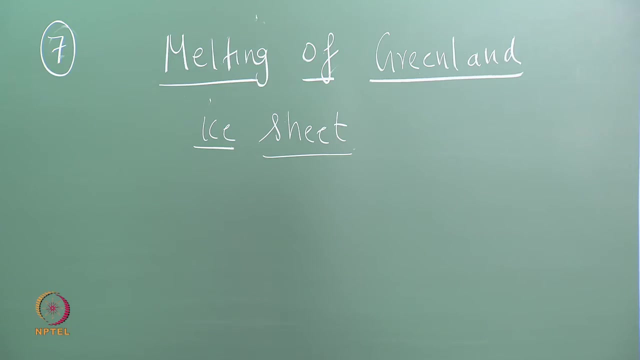 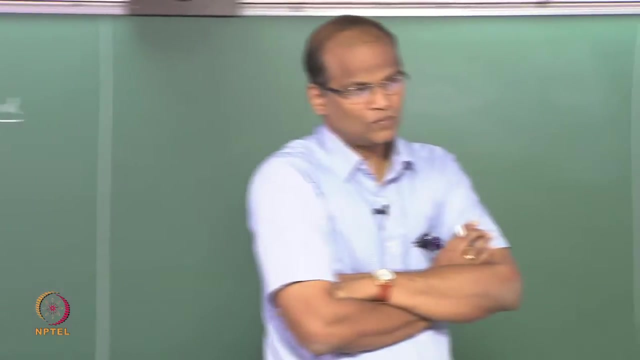 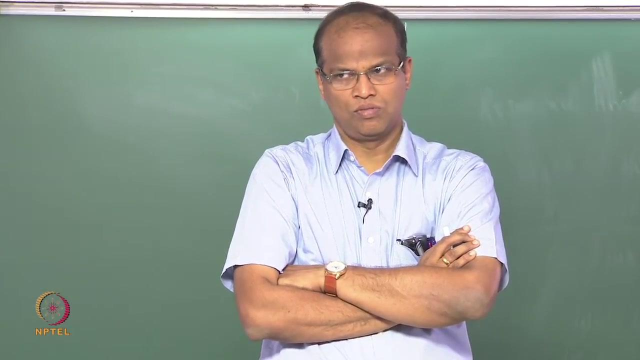 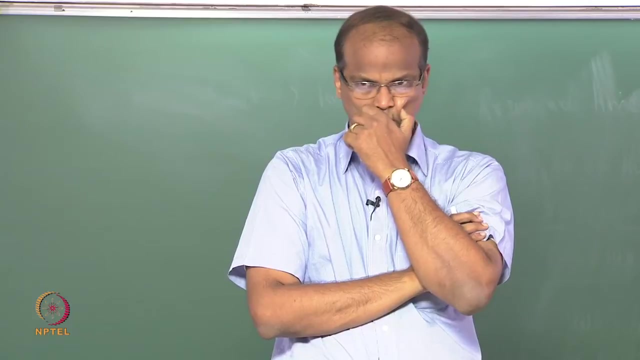 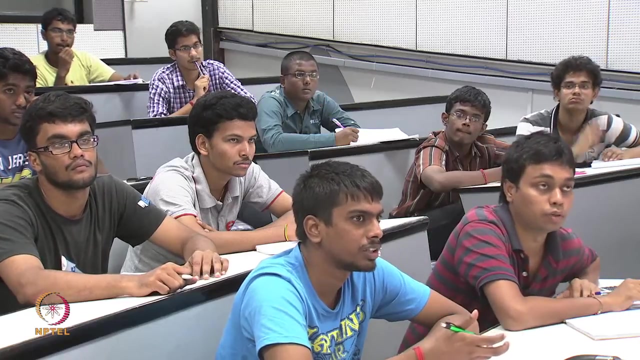 Ok, Ok, Ok, Please start solving. So first you will have to calculate the mass of the Greenland ice sheet, correct? that is the first step. What is the area over which the ice sheet is? It is always based on per meter square of the surface area, So you have to multiply. 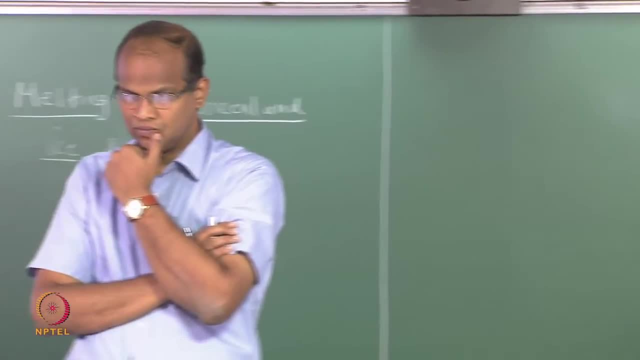 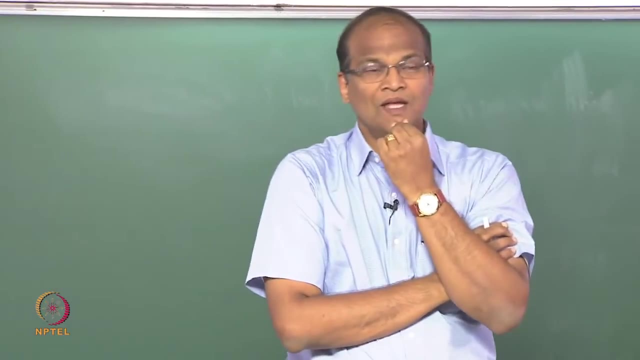 it by 4 pi r e square. ok, Ok, It is kilogram per meter square of the earth's of total surface area of the earth. that is the way it is. the. these are the units used in atmospheric science. I told you in the first. 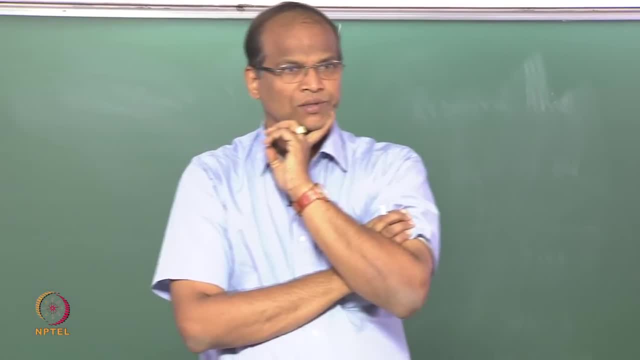 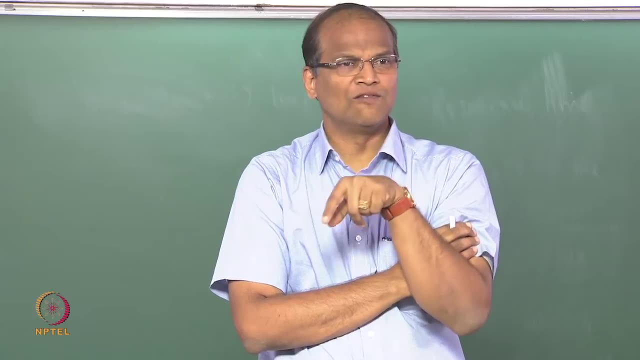 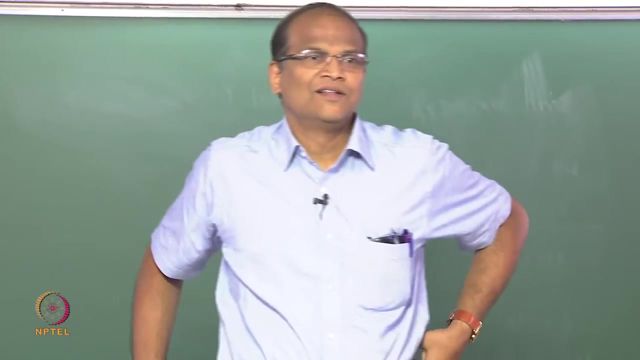 class itself. What is the per meter square of the ice sheet? Then you are tying yourself up in knots, isn't it? there should be a baseline for this thing. then you will never be able to calculate that value, right? so next you will ask me, sir, what is this square area? surface area of the Antarctic ice sheet. 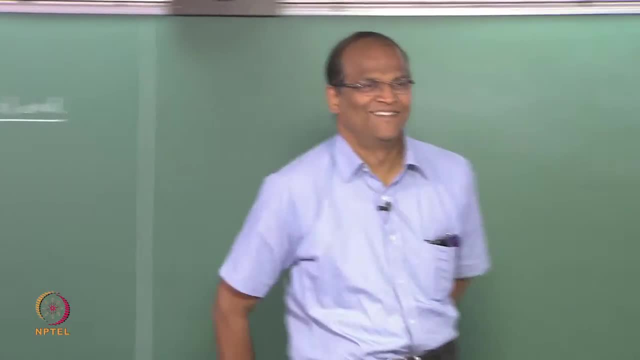 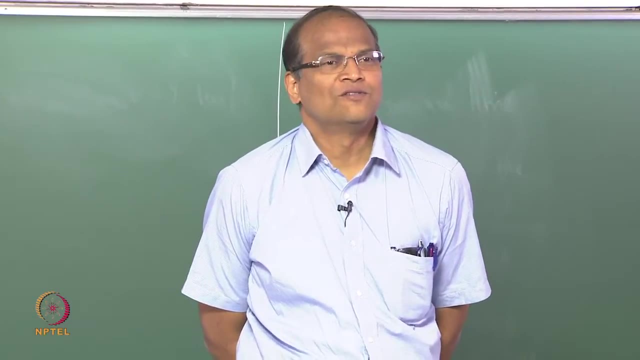 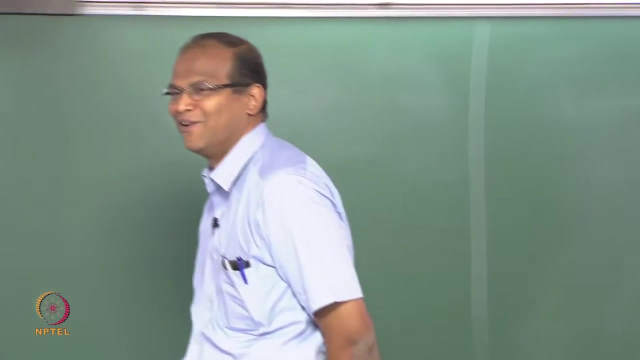 So this will go on. so somewhere you have to understand: Where is your house? my house is next to his house. where is his house? His house is next to my house. I mean, means that problem cannot be solved? ok, Let us work it out slowly. 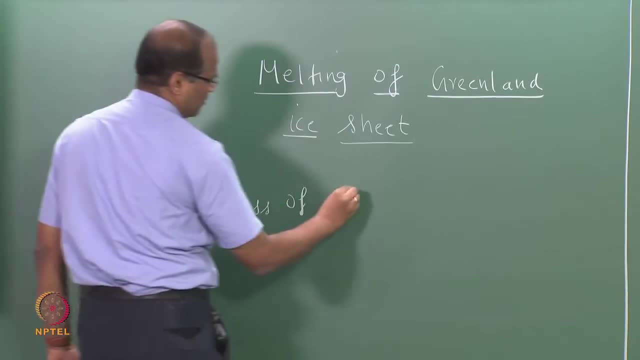 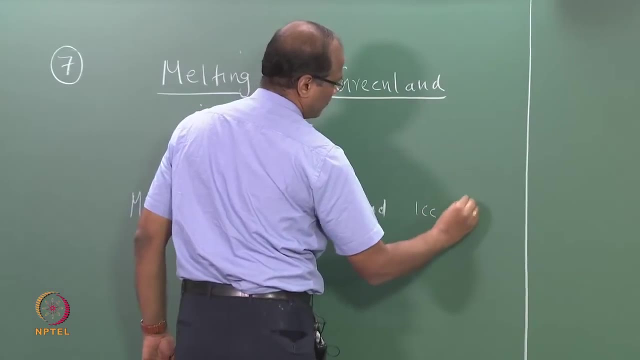 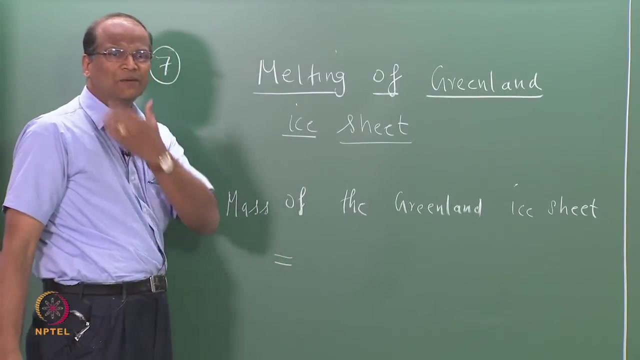 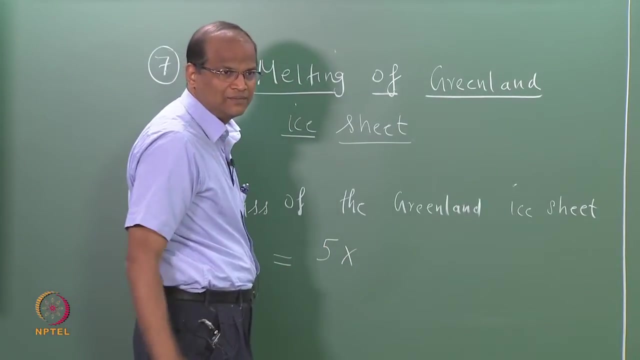 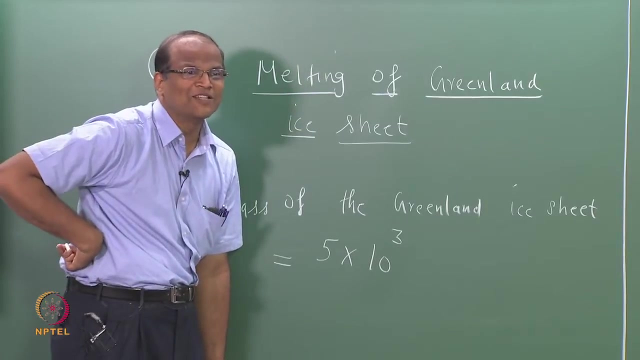 If, Yeah, Yeah. So mass of the Greenland ice sheet is what is the value given in the table 5, 5 into 10 to the power of plus 3? because mass into 10 to the power of minus 3 kilogram per meter. 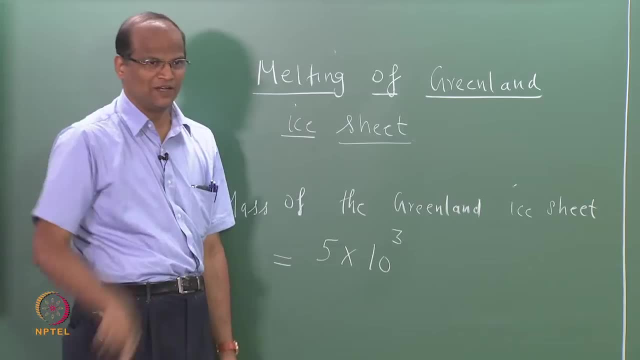 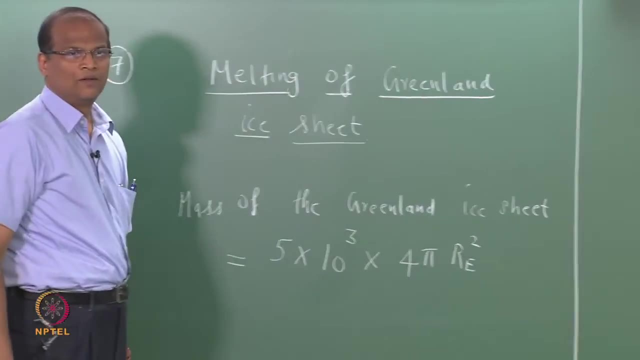 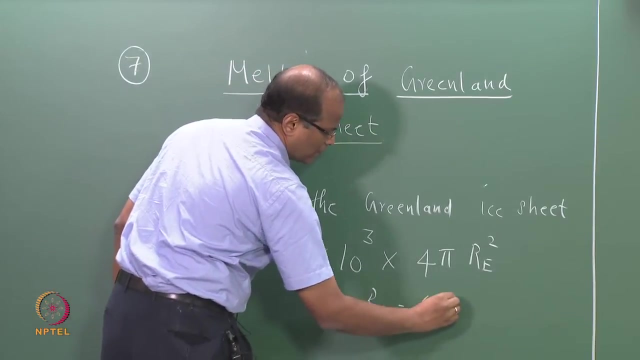 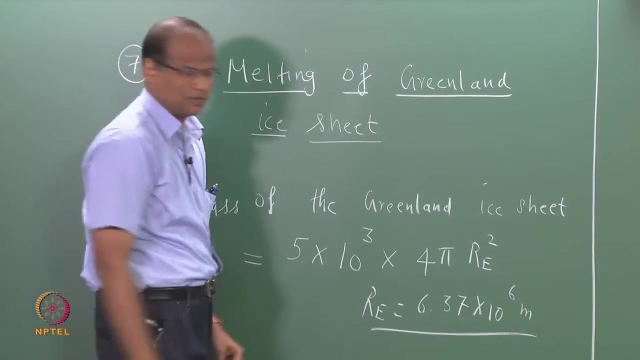 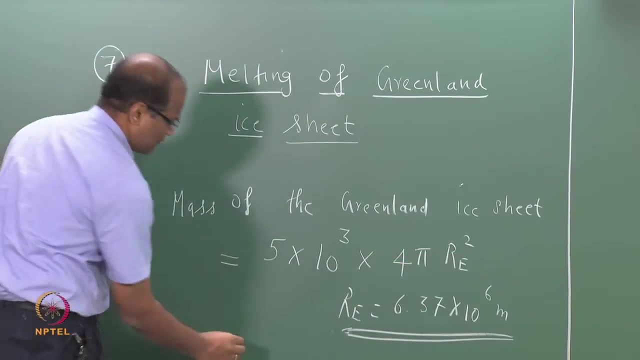 square is 5.. Therefore, mass is 5 into 10 to the power of 3 into okay. So this is the radius of the earth. please do not forget this in this course. okay, Yeah, substitute 6.3 into 10 to the power of 6, tell me some huge number. 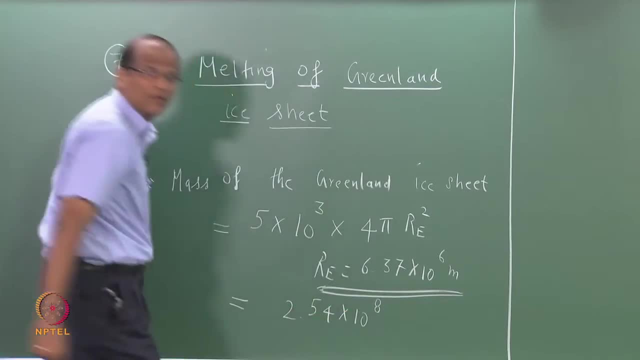 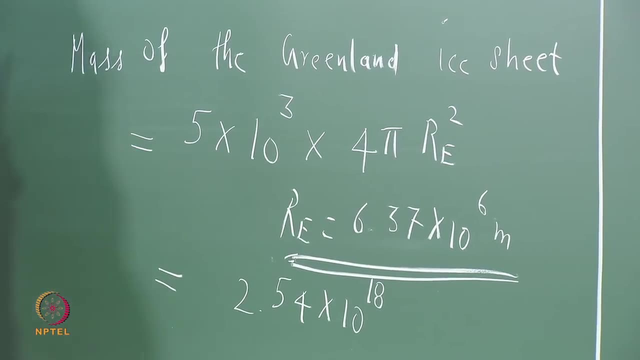 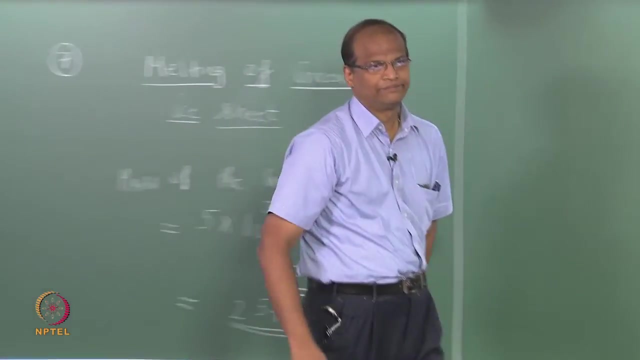 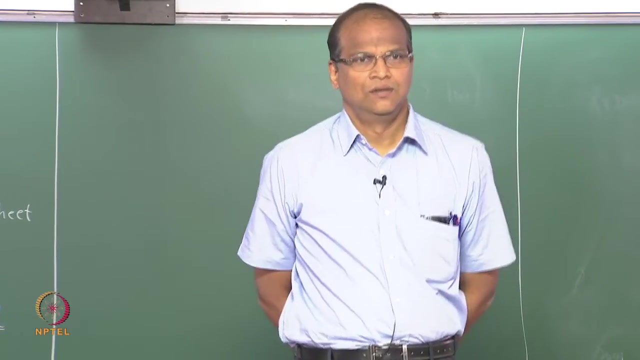 2.5 into 18.. Oh, kg, or tons, Kg, Kg, is it okay? Now we have to find out how much the level will rise. For that you have to make an assumption. Density, sad Density, okay. 1000, 1000 kilogram per meter. 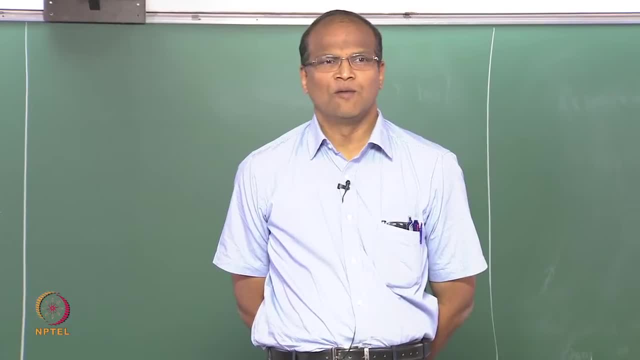 cube Density 1000. Version: friendship Density: present Density: Okay, 1000 kg per meter cube. assumption number 1 density is 1000 kg per meter cube. forget the 1025,, that is okay Then. 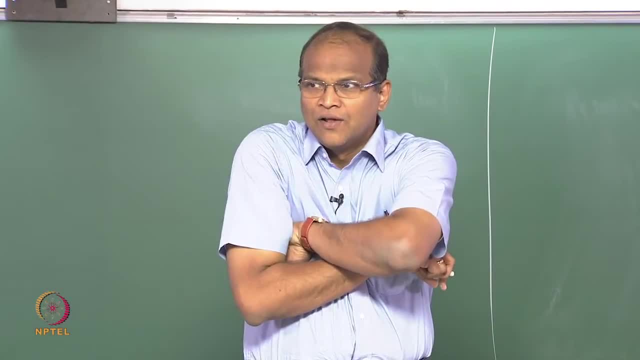 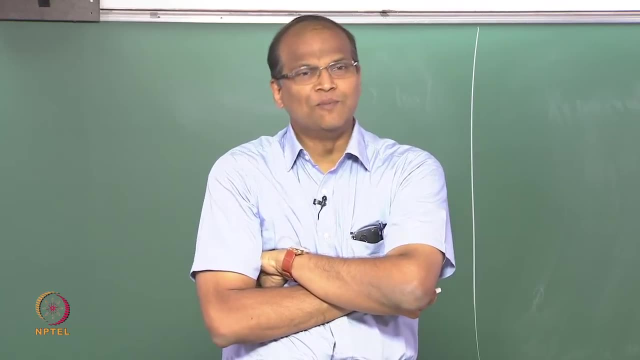 2 third of the earth surface is covered with water. Not 2 thirds. what is it? We have to make couple of assumptions. 72 percent of the earth surface is only covered with ocean. density of water is 3.. So 3.2 정도 we only can. 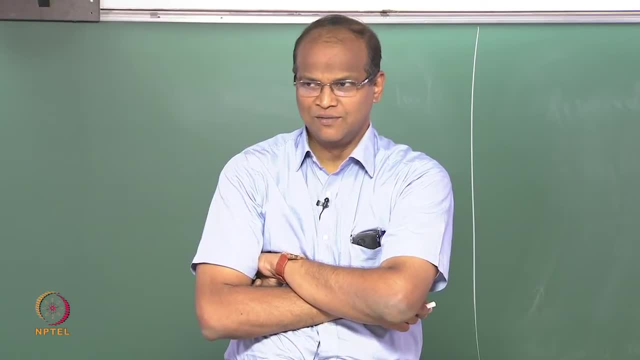 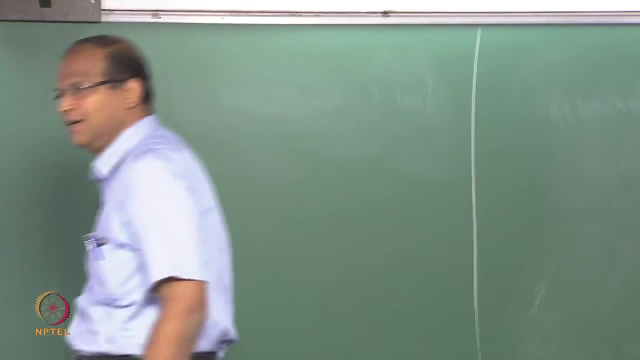 have enough paper for this right. That is why we have to make 2 parts of F, where the species Tensity of water is 1000 kilogram per meters meter cube and when it melts it will be uniformly distributed over this 72 percent correct. 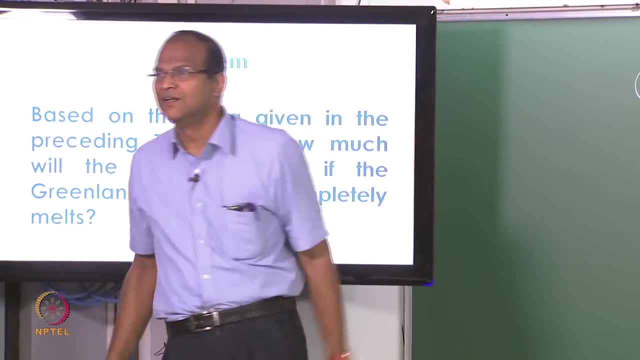 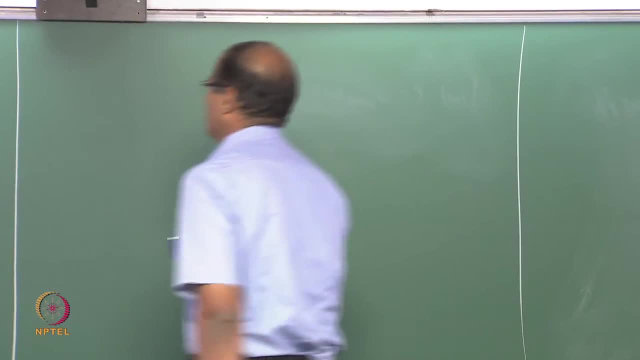 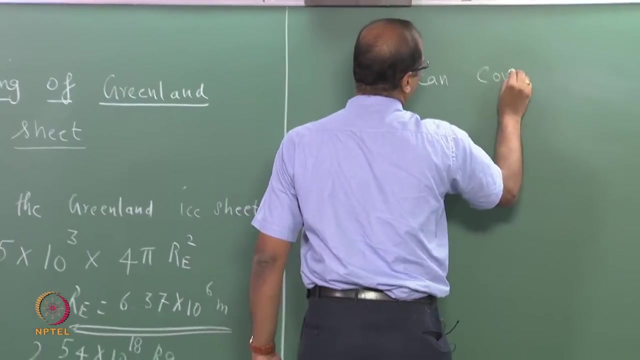 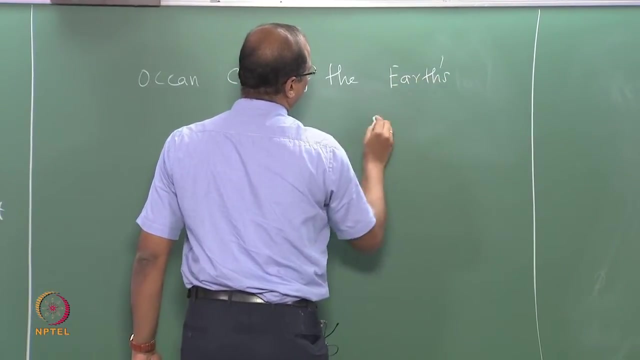 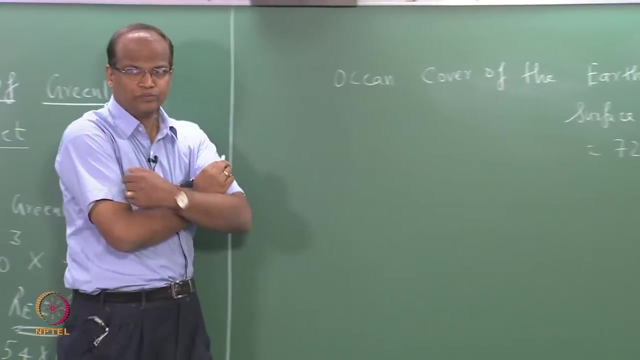 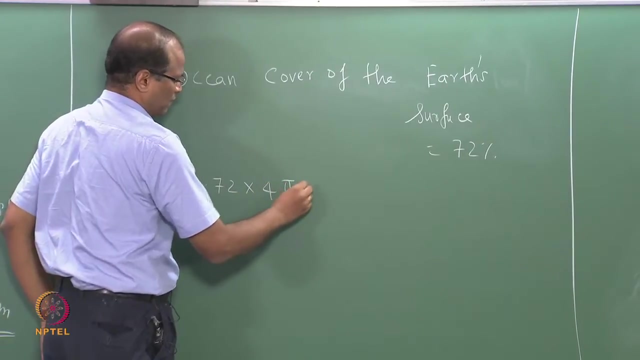 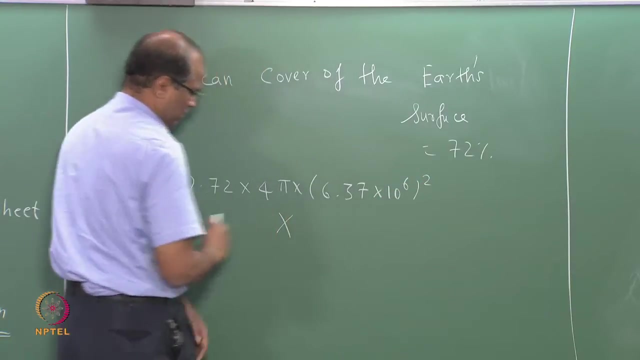 Now calculate the keep, the height by which it rises as x. pull out the x. ok, Now what is it? So this is x 1 minus x 2 plus x 1 minus x 2 plus x 2 minus x 2 plus x 2 minus x 2 minus. 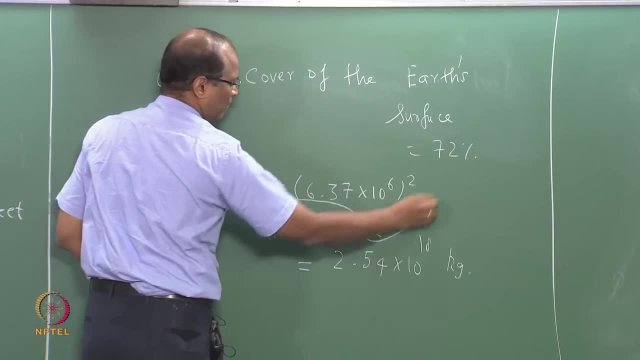 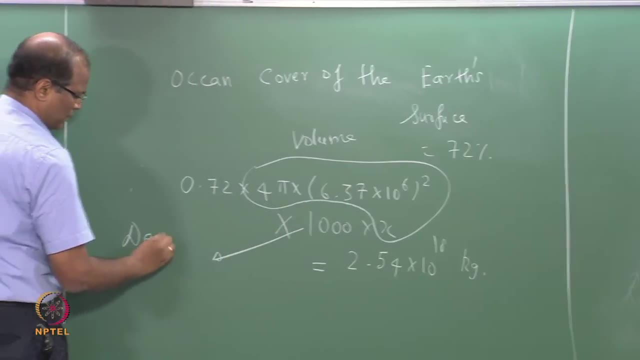 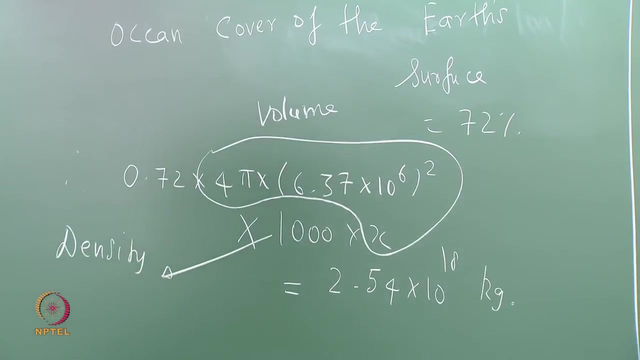 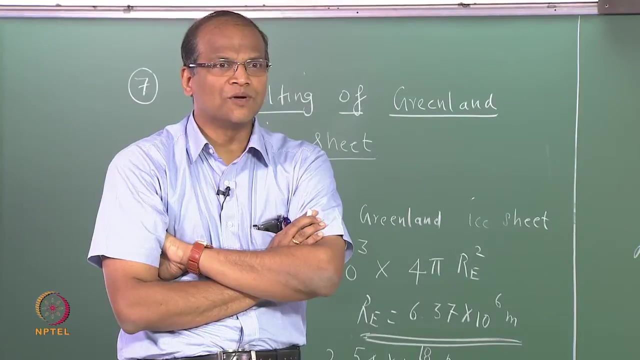 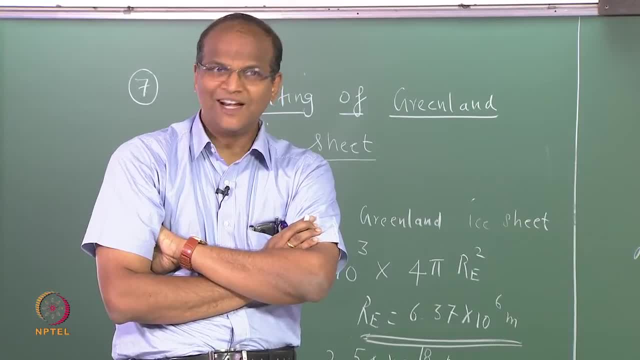 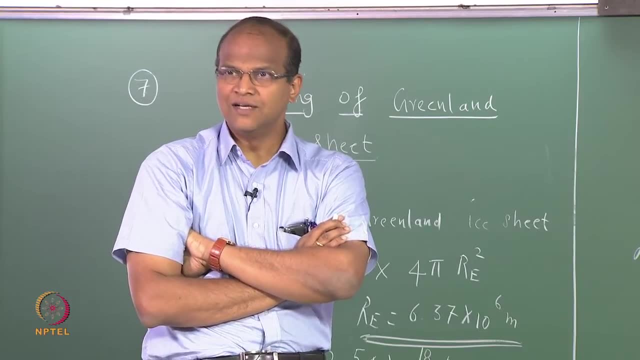 So what will happen to the whole Greenland? ice sheet melt, 6 points something. Yeah, Ok, 5 meter is like 22 feet or 23 feet. very bad scary, is not it? So you can find out, if any of the other things melts, what happens. you can do the calculations for other things also. 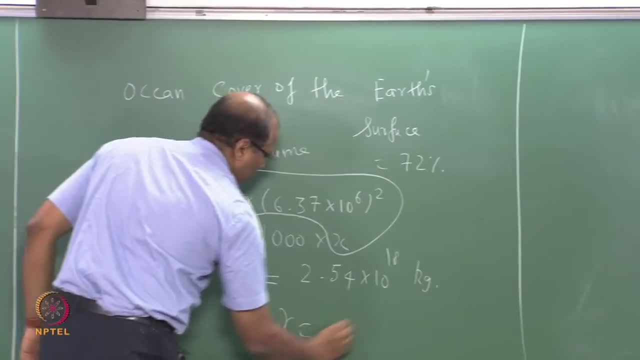 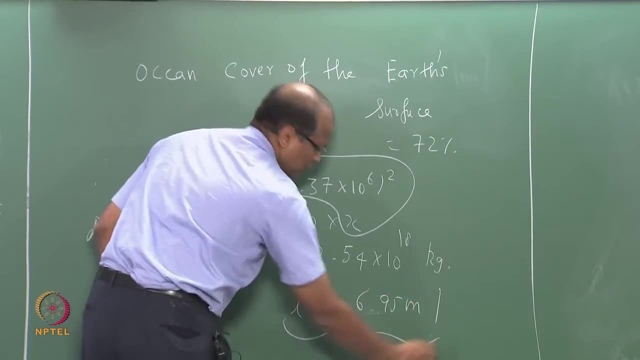 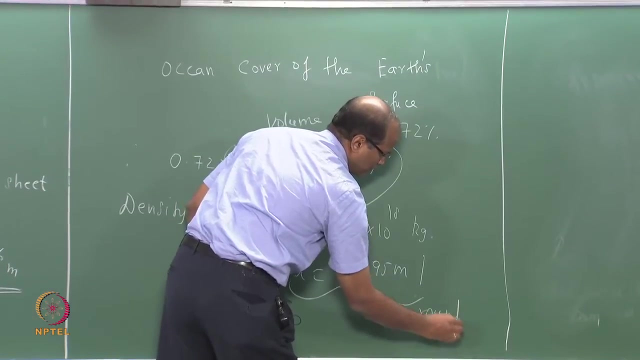 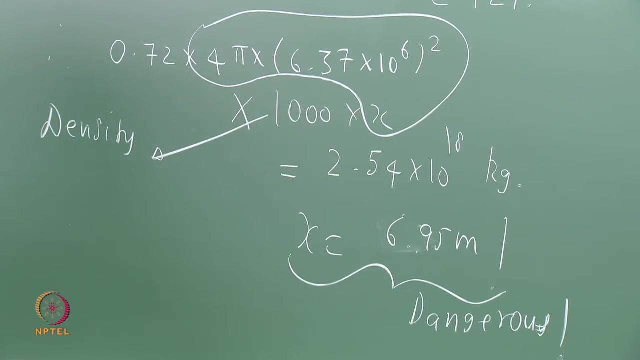 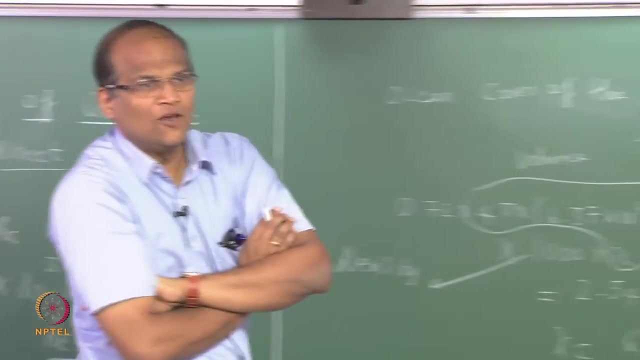 right. x is 6 point. So it is a. it is dangerous, right. simple analysis we are able to say: but it would not melt day after tomorrow or tomorrow, right, do not worry about that. but if it melts, then like that, any of those, any of those things which are remaining as ice if they melt. 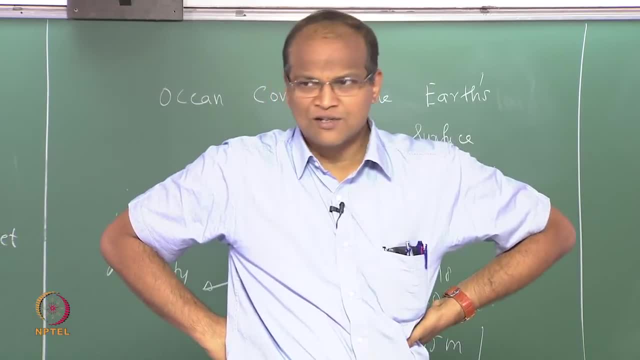 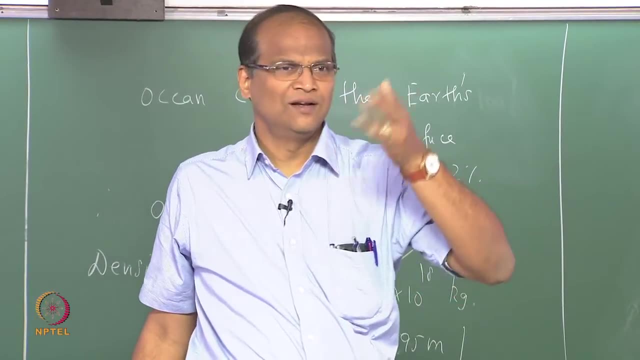 That means we are going to have trouble for a long period of time. the trouble is not next week or next month, but this is: if the global warming takes place slowly but surely, the temperature is increasing and the temperature anomaly is correct, as reported by Charles. 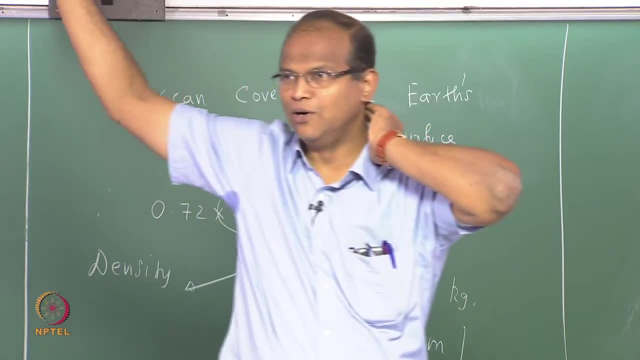 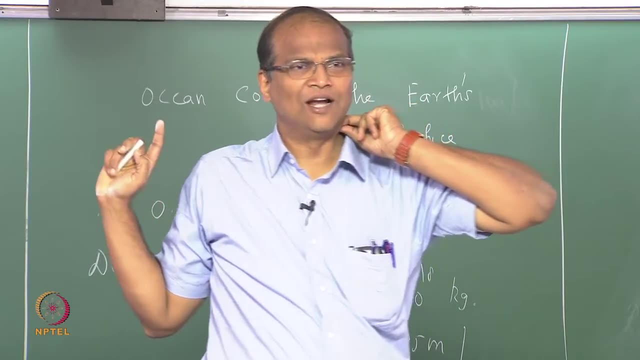 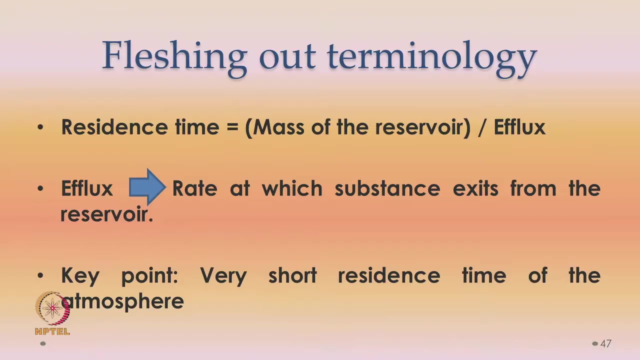 Keeling carbon dioxide and Monolova Hawaii. if that were to be true, then you can say that we are in trouble. man will come out with some solution. that is a different matter. Okay, but right now, this, it is a cause for concern. all right, now let us go back to the 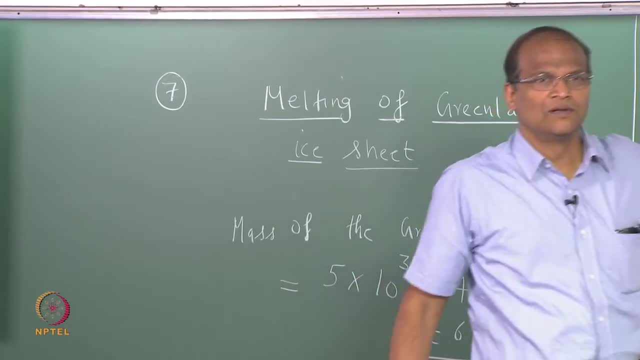 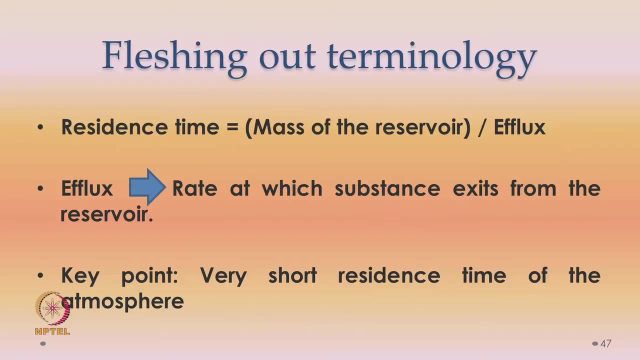 why is the residence? is everybody through with this problem? 6.95 last bench, is it fine? 6.95 meter, Okay, why do you think we have a very short residence time? on the atmosphere, this one right. can you tell me some reason? 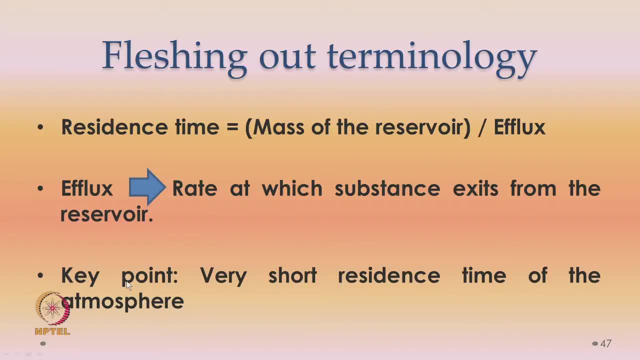 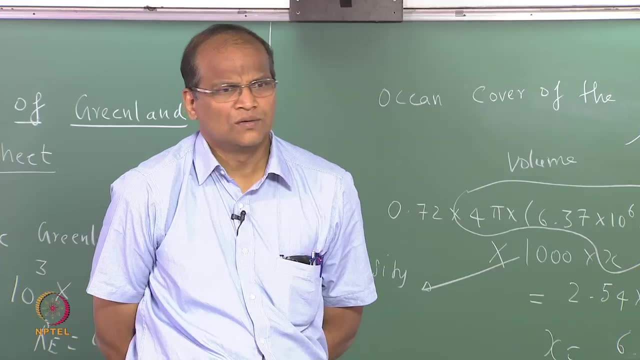 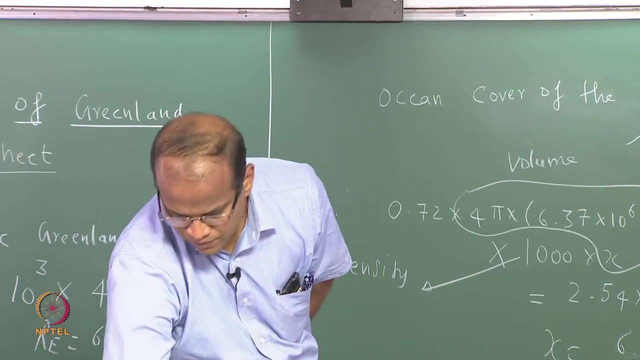 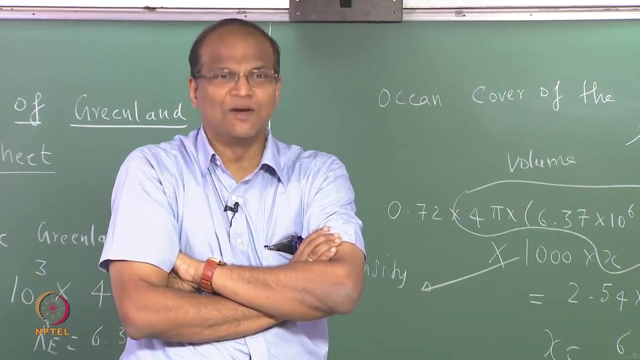 Okay, Anybody, No, no. what is the for atmosphere? what is the? what could be the reason? residence time is. mass of the reservoir divided by a flux. What is the mass of the reservoir? mass of the reservoir. So, if you want to have low, 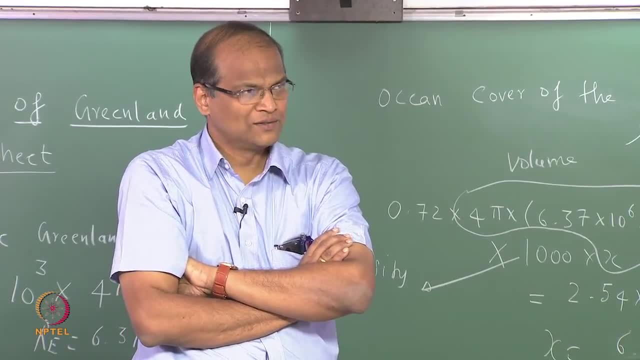 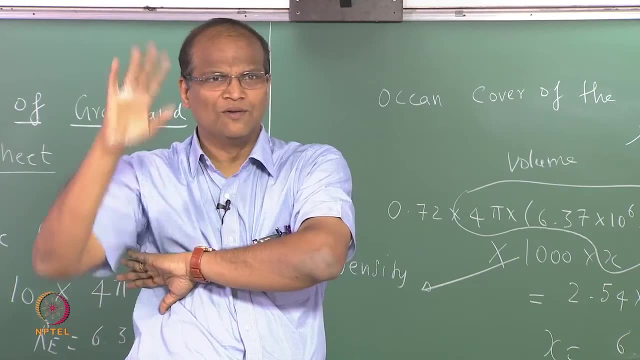 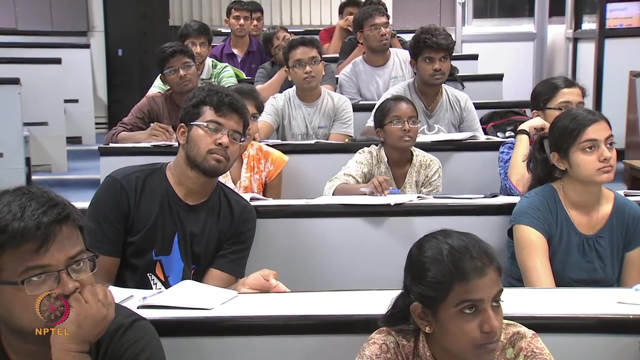 residence time you have. you either have low flux or you have high efflux or low mass of the reservoir. The mass of the reservoir is reasonably low. we will remove that. the efflux seems to be very high for the atmosphere. why Continuous interaction? Continuous interaction, large exchange rate because of winds and other things, So atmospheric. 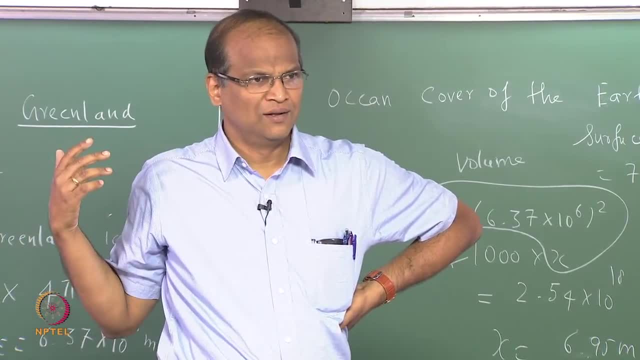 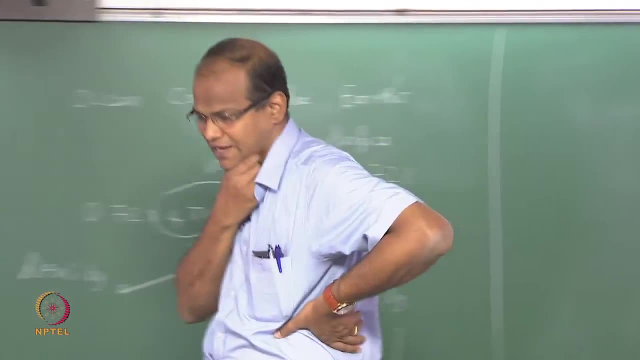 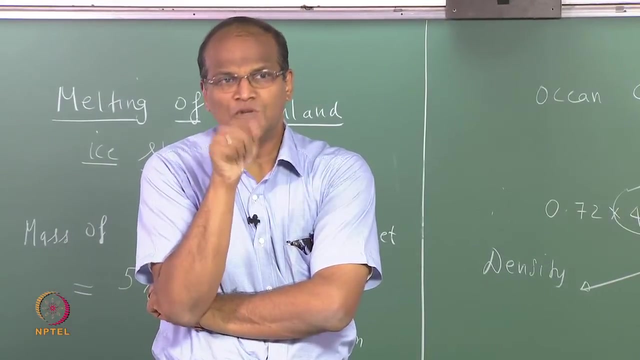 processes are very fast compared to the processes in the mantle, okay, and there is a large latent heat of vaporization of water. Because of this, Because of this generally, the atmospheric time scales are very less okay. So therefore, the atmosphere is a very efficient component of the earth surface in transferring the energy. 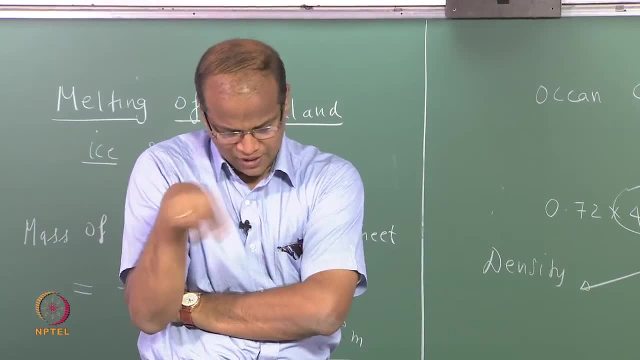 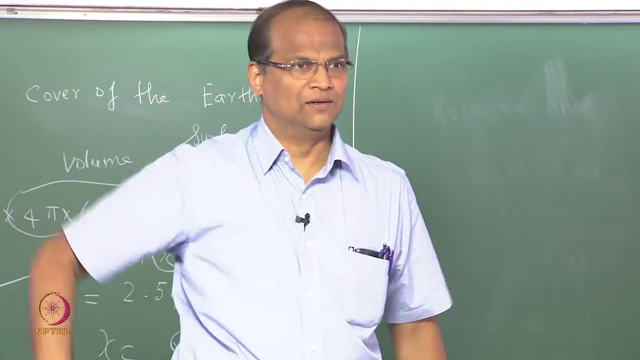 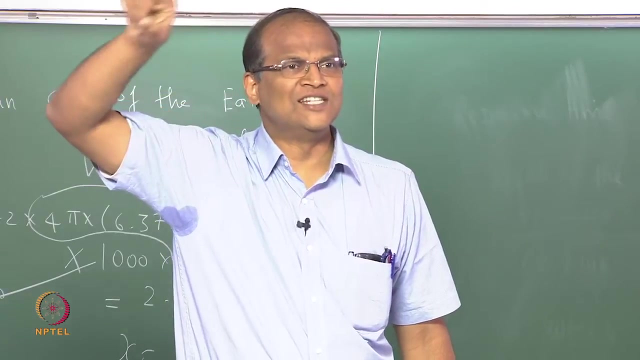 and water from the earth surface to the atmosphere. right, are you getting the point? See, the atmospheric- sorry, the atmospheric- branch of the hydrological cycle is very efficient because it can do things very quickly. Okay, In your hydrological cycle. this complex interplay of various things in the hydrological cycle. 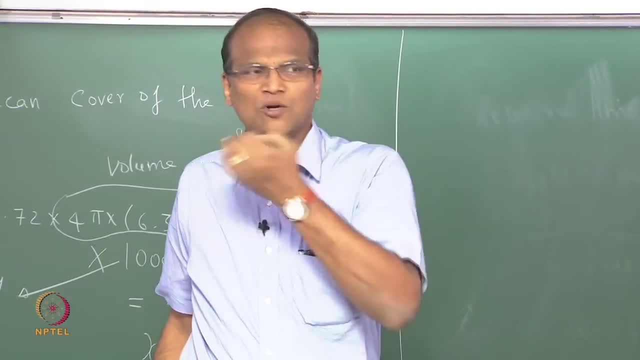 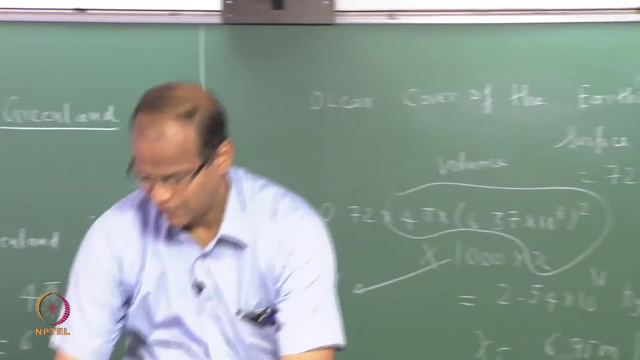 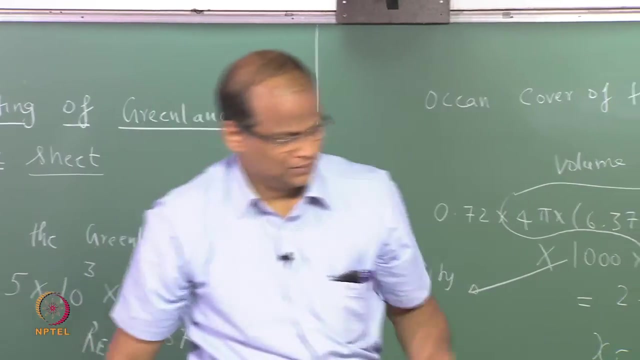 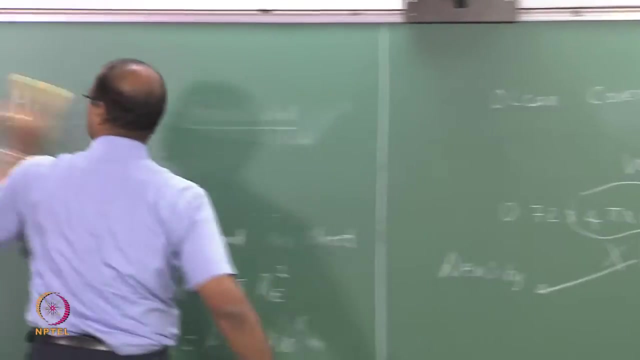 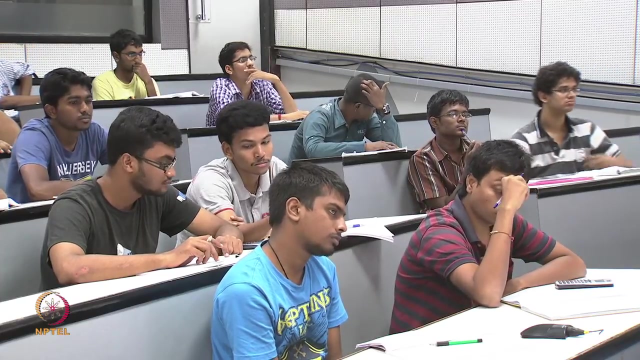 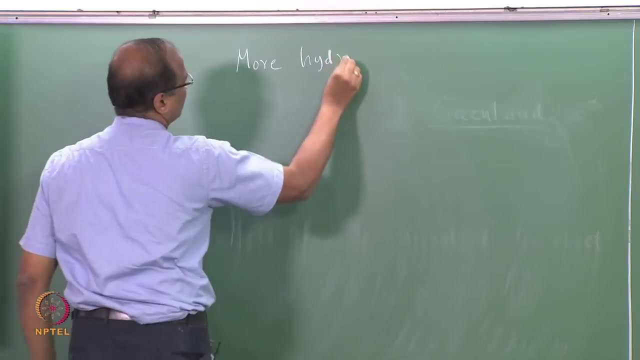 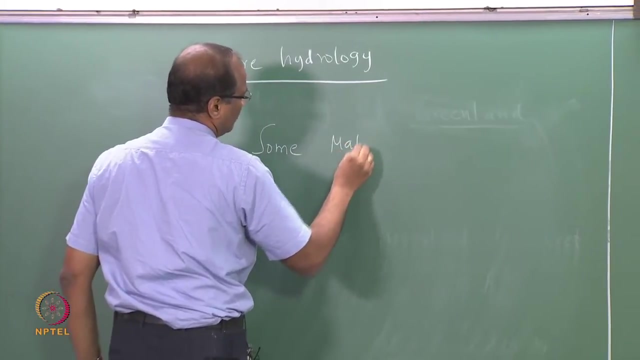 the atmosphere plays a very important role, because processes- processes- are very quick in the atmosphere, is it okay? next we will have to go to next two classes. Let us do some little bit of math in hydrology, okay, Okay? So let us look at the 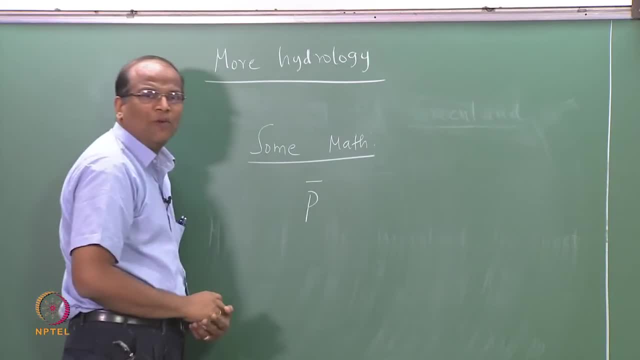 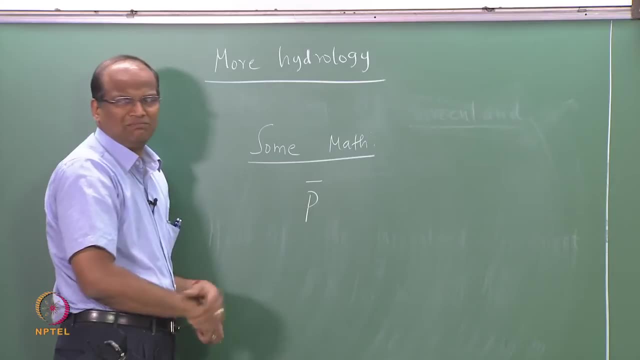 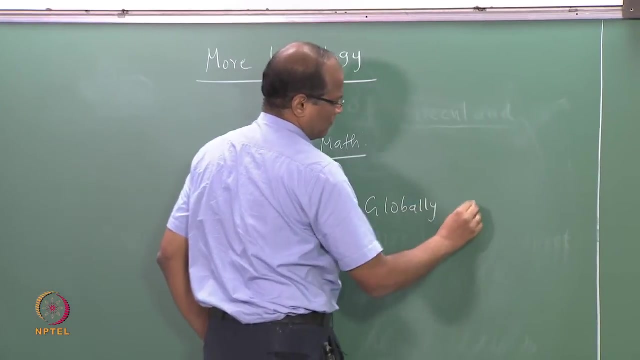 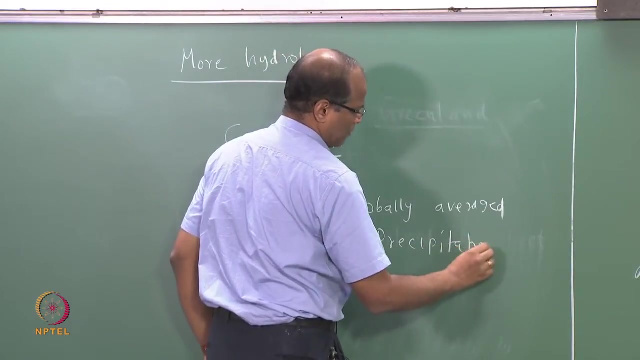 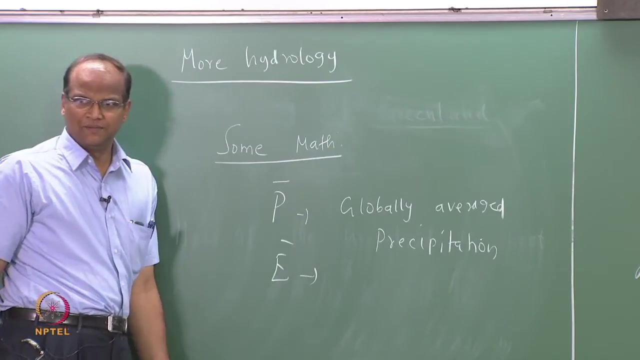 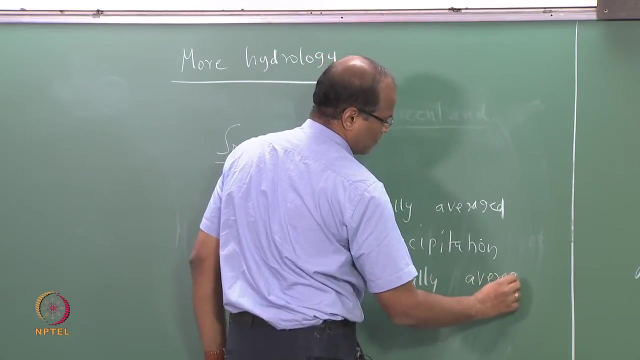 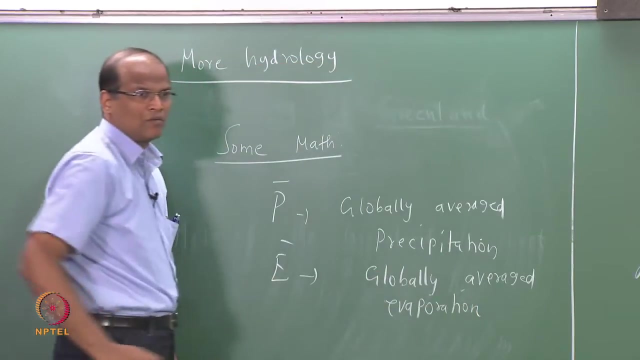 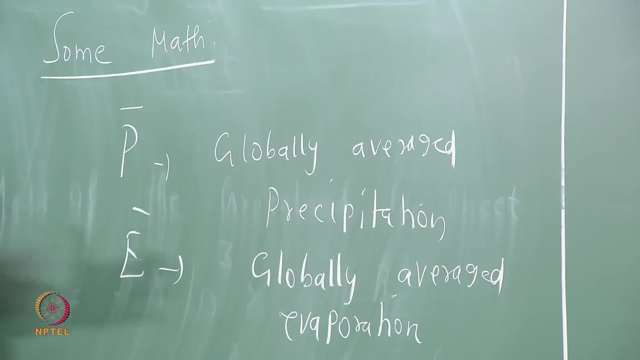 let us say that the Okay Globally averaged precipitation- centimeter per centimeter per year or millimeter per month or something- is globally average and E bar is a globally average evaporation. What can you say about the two On an average? if you are sufficiently average, P P equal to E, very good, that is what you. 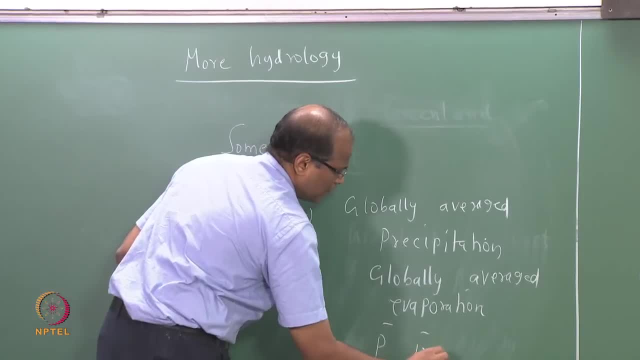 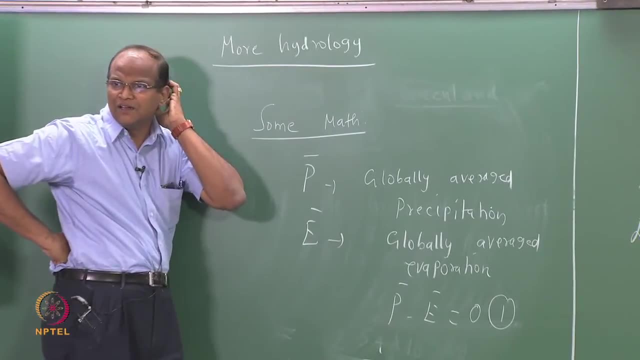 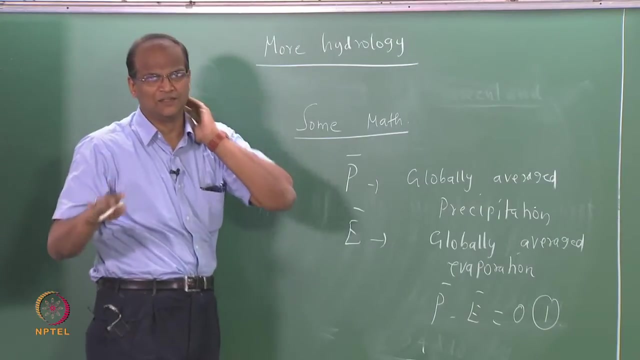 can say- That is our first equation. At a global scale, precipitation is equal to evaporation. If this were not to be the same, some lot of changes would have taken place which would have been noticed by several scientists, which would have caused some other changes. 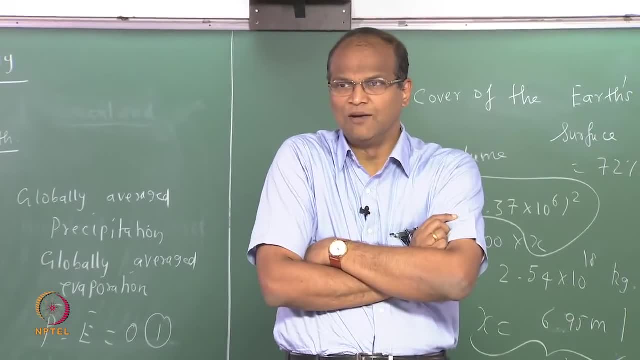 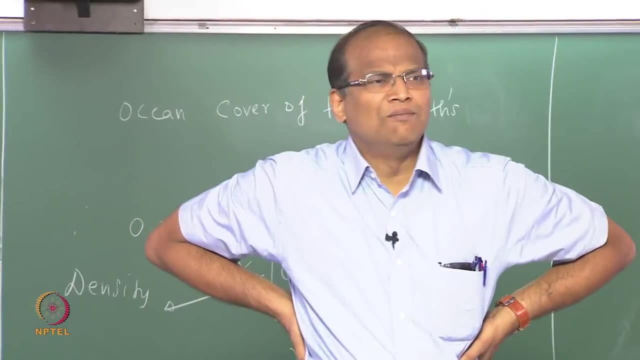 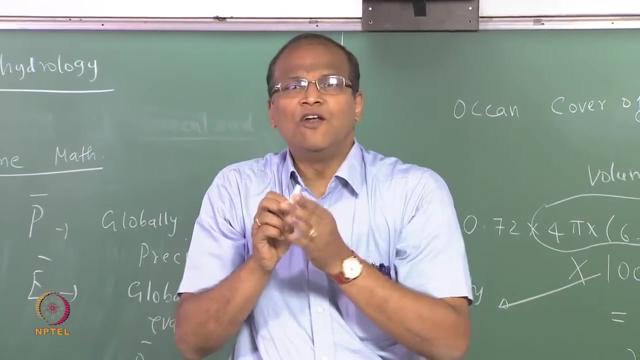 So we have proved that it is clear that those changes are not taking place. Therefore, there is no appreciable imbalance. There is no appreciable imbalance between the globally average precipitation and the globally average evaporation. However, when you analyze the hydrological balance for a limited region, P is not equal. 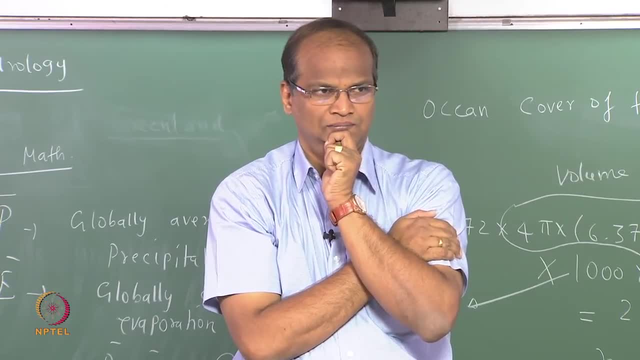 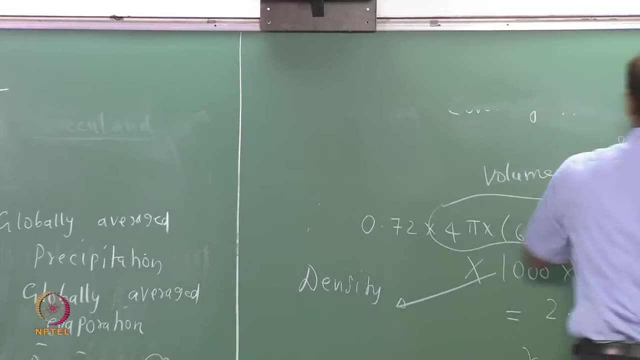 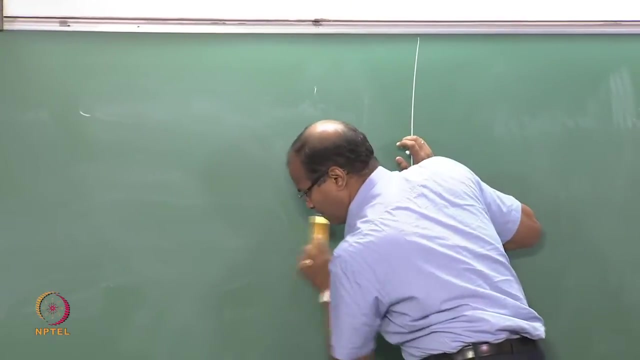 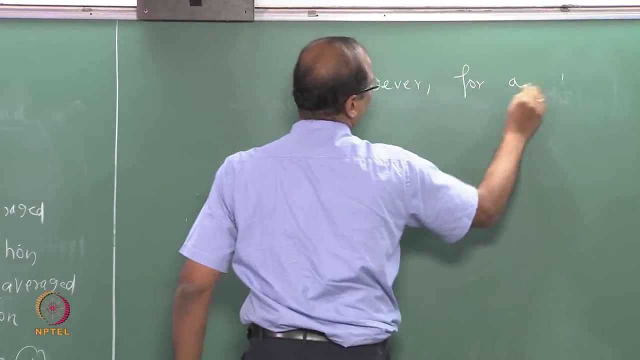 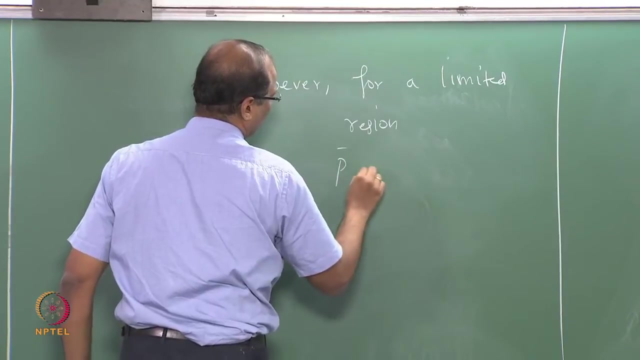 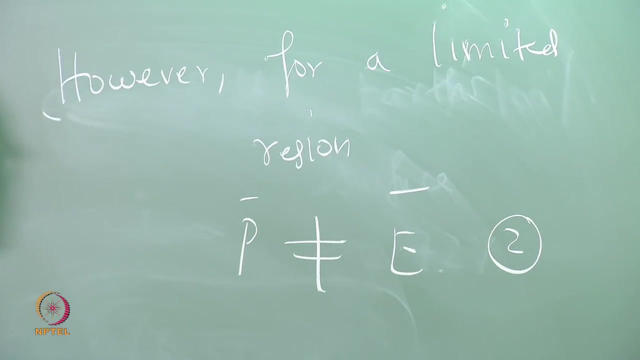 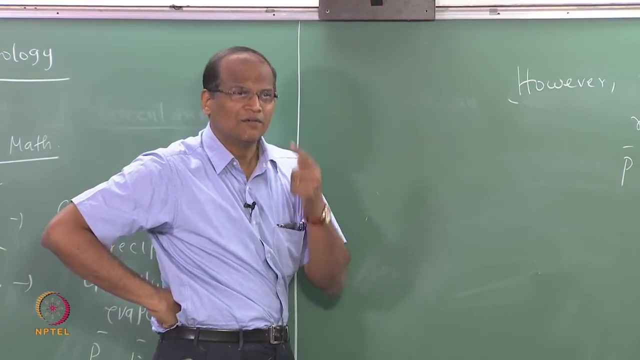 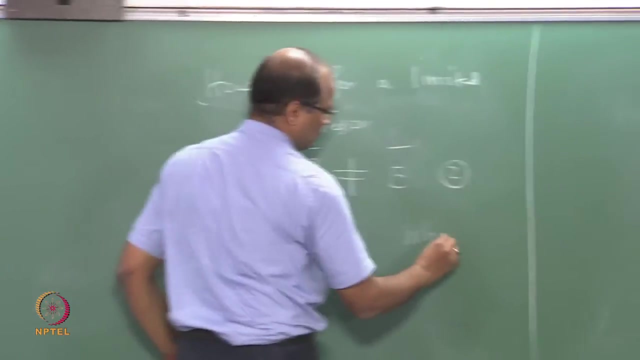 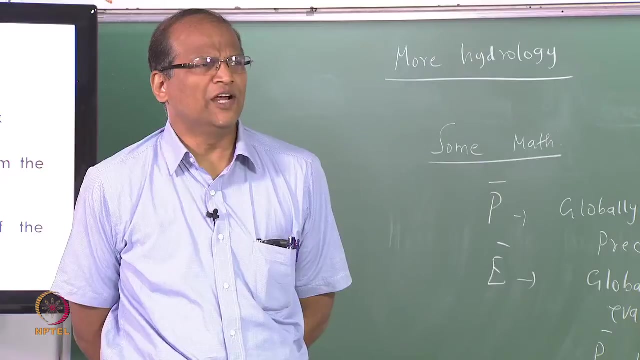 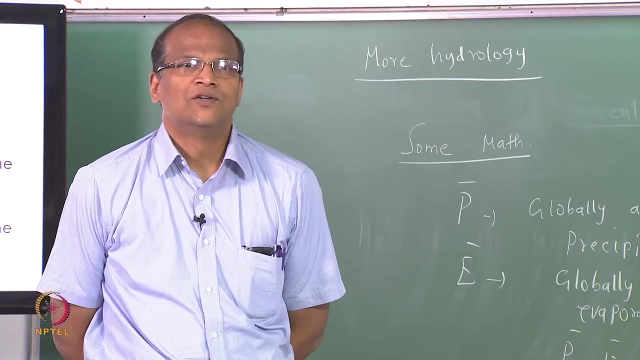 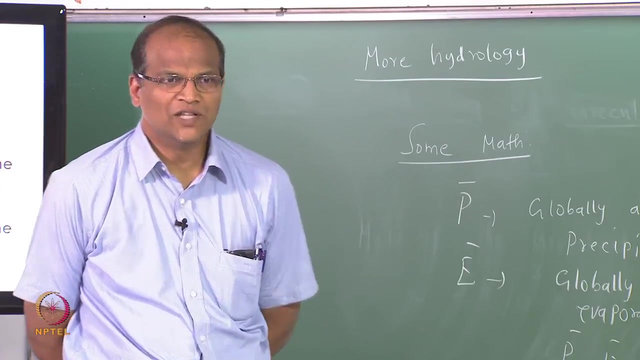 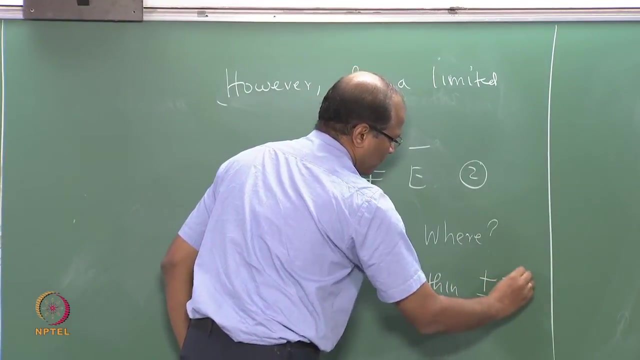 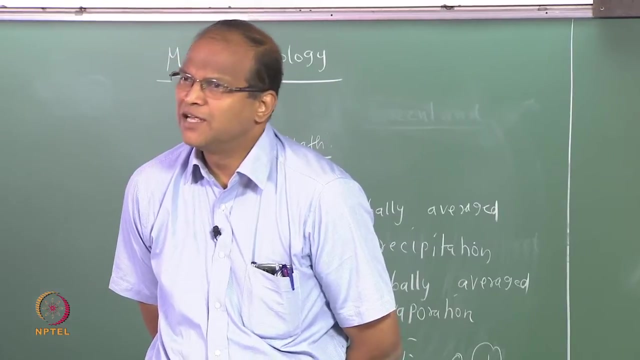 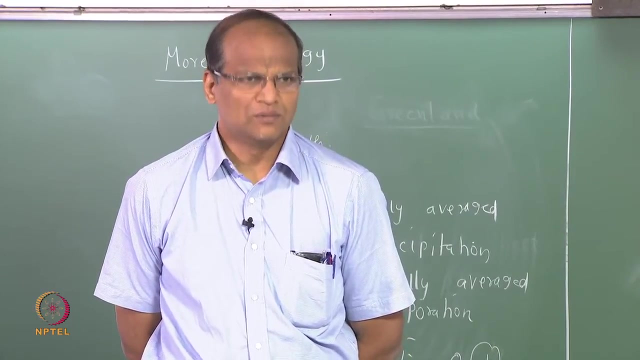 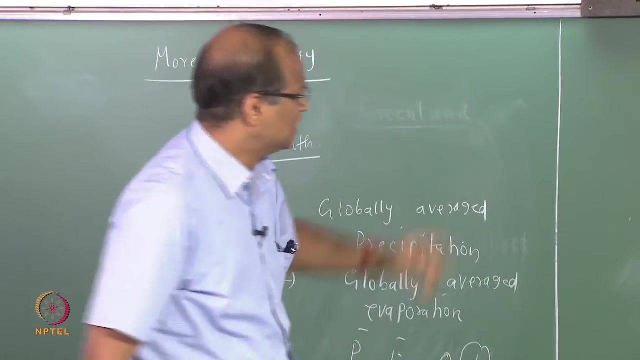 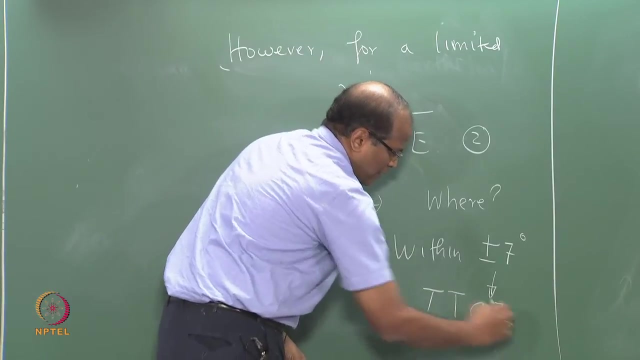 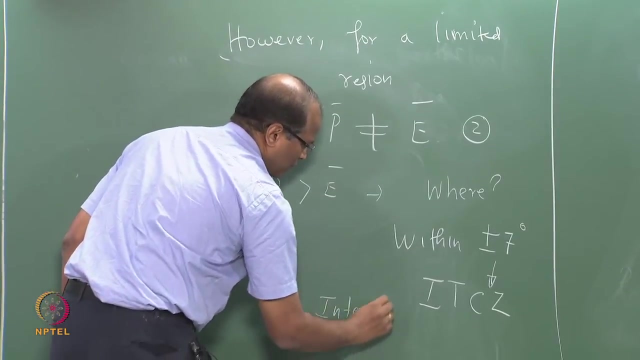 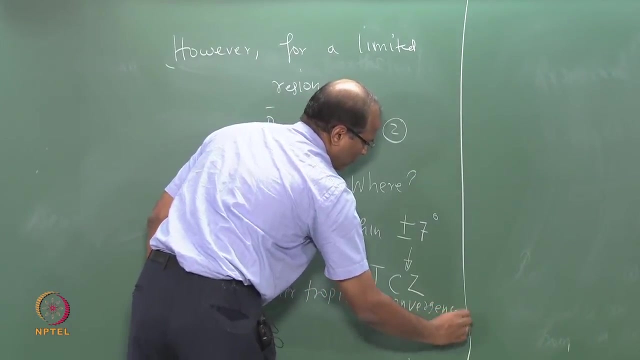 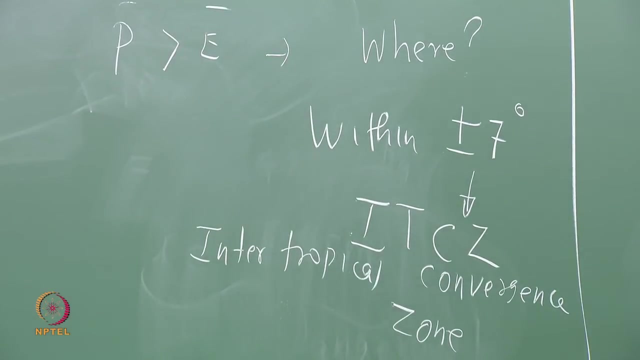 to E. Now you are able to understand what I am the subtle difference. A probedite is called an inter-tropical convergence zone. 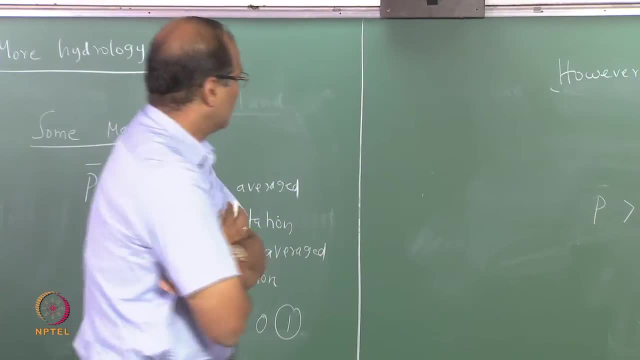 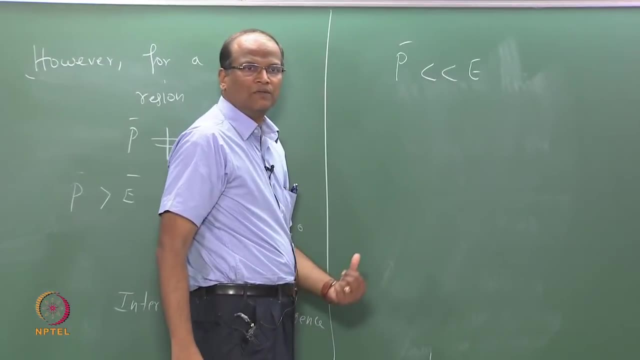 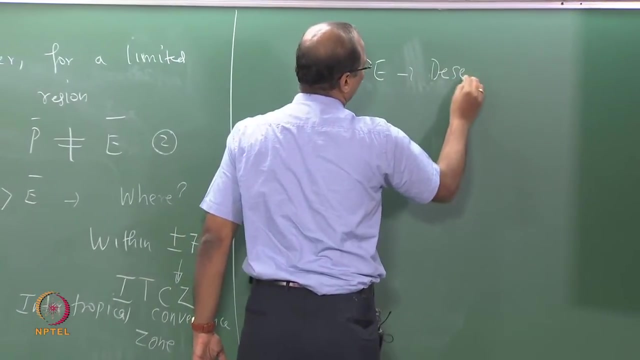 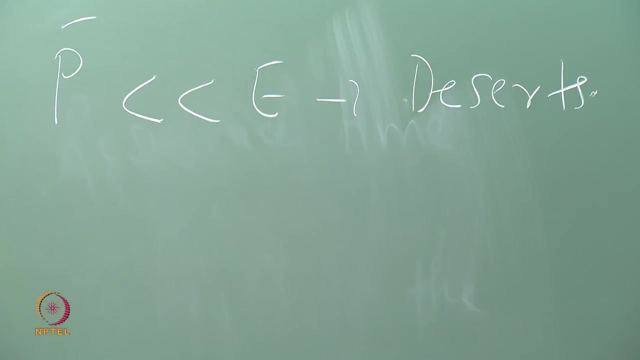 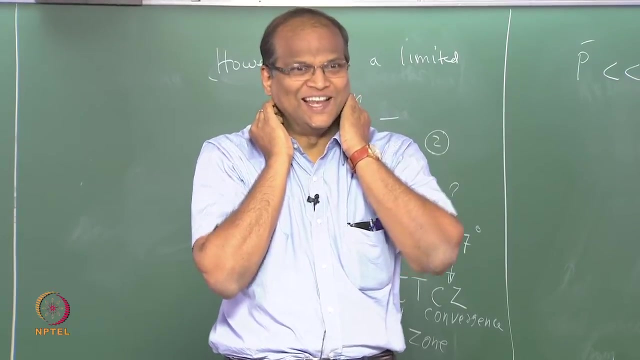 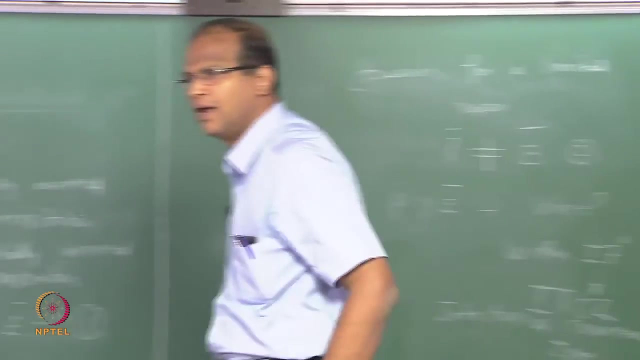 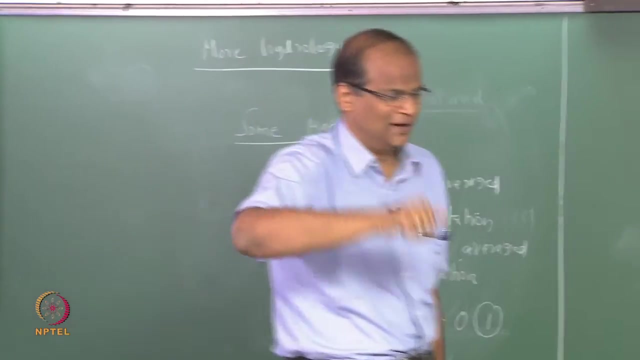 Now P is where Deserts. If P is much, much smaller than E over the desert, evaporation is very less, sorry, precipitation is very less, evaporation is very high. Now this water vapor. where is it going? The question clear. Where is what do it? Now you are able. 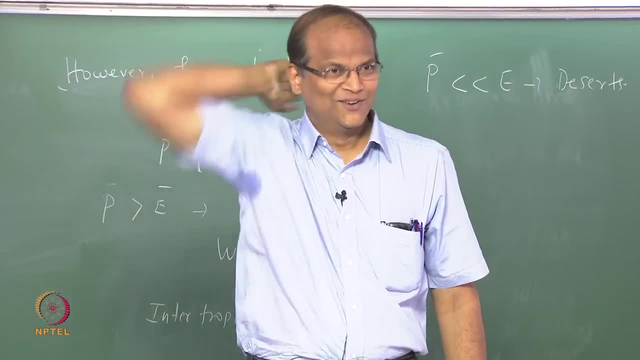 to understand that is called RG. ok, Lot of evaporation is taking place. these deserts are basically 10,, 15,, 20,, 21,, 22,, 23,, 24,, 25,, 26,, 27,, 28,, 29,, 30,, 31,, 32,, 32,, 33,, 34,, 34,, 35,. 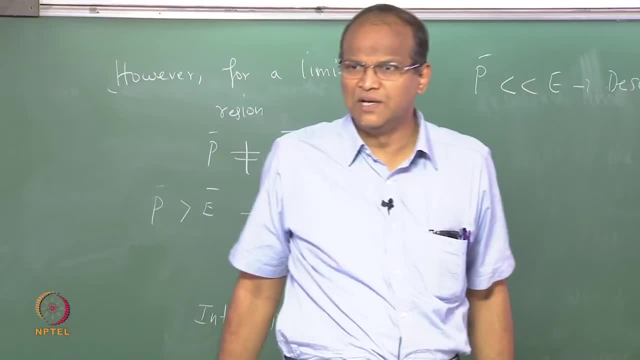 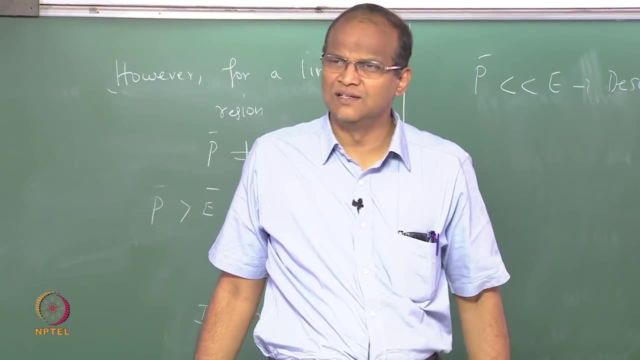 32,, 32,, 34,, 35,, 38,, 40,, 40,. Chaitanya audience can talk. fanンy 2025, 0°, whatever. if either Dubai 0° must be, 20° Dubai 15 to 20° are fine. China 0°, Delhi 30,, 29° Dubai must. 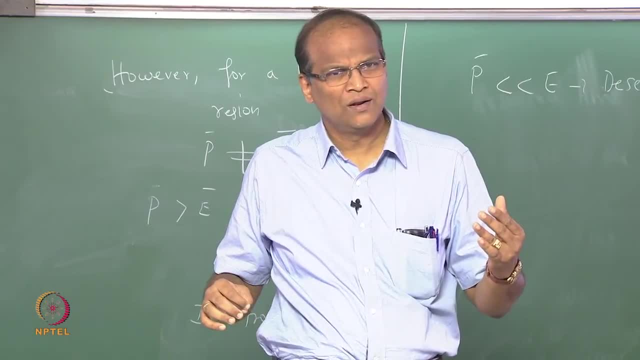 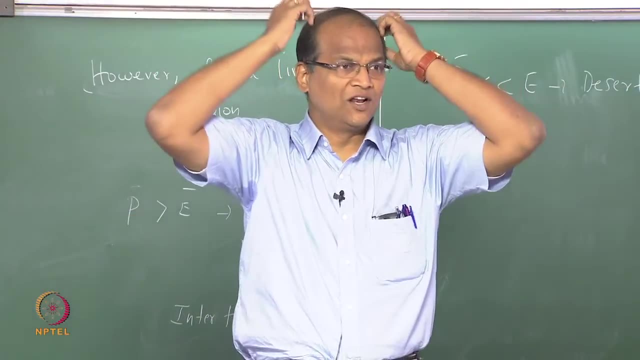 be 25, I don't know more around that. only so as this water evaporates and becomes water vapor. this water vapor is carried either to the intertropical convergence zone or it is taken. So that's all. And if you look here, completely other than water, overly vaporization. 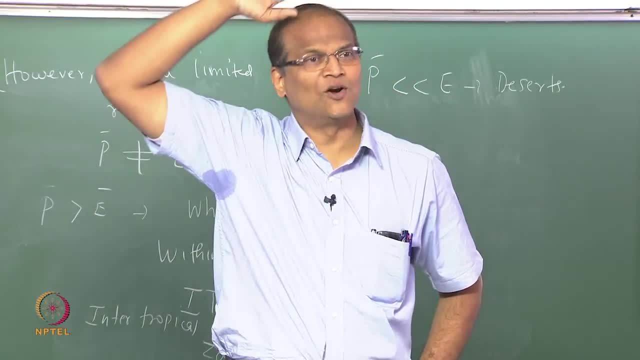 as this water evaporates and becomes water vapor. this water vapor is carried either to the intertropical convergence zone or it is taken to thebe tropical convergence zone, taken to the mid latitudes where it causes lot of rain in Europe and other place. So 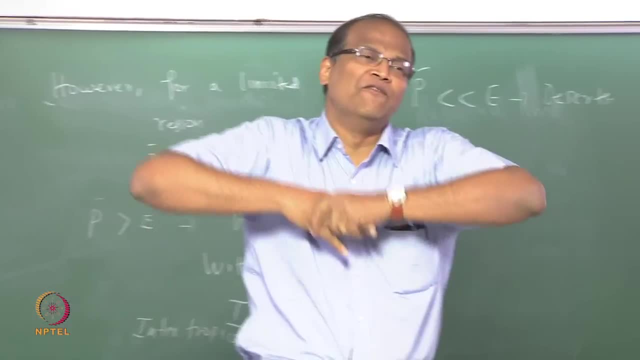 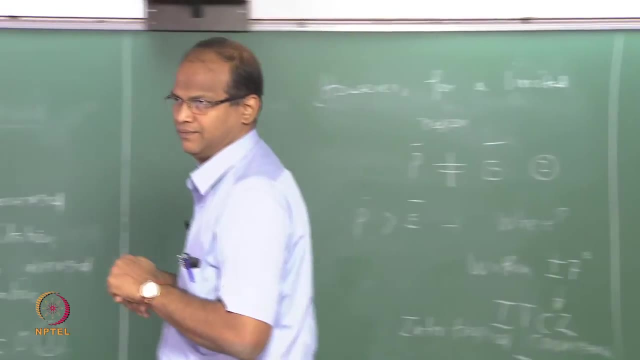 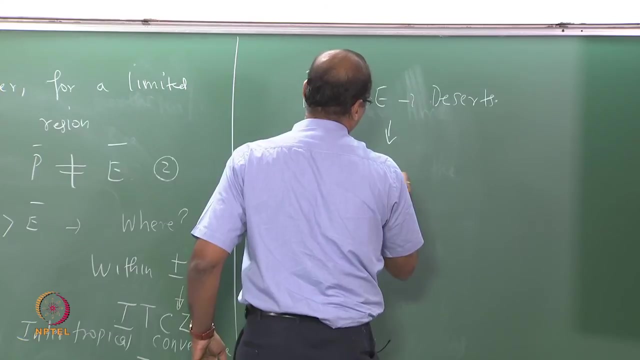 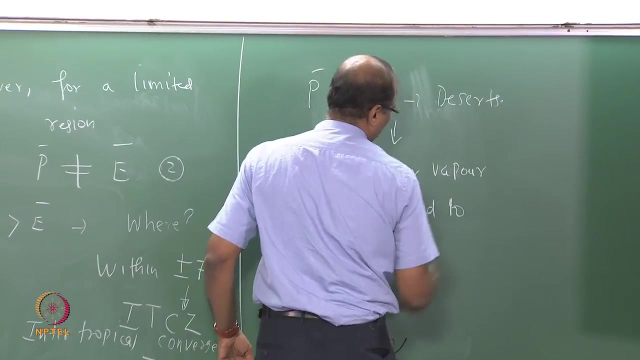 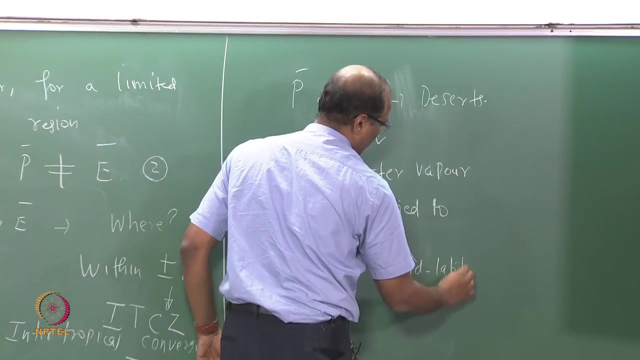 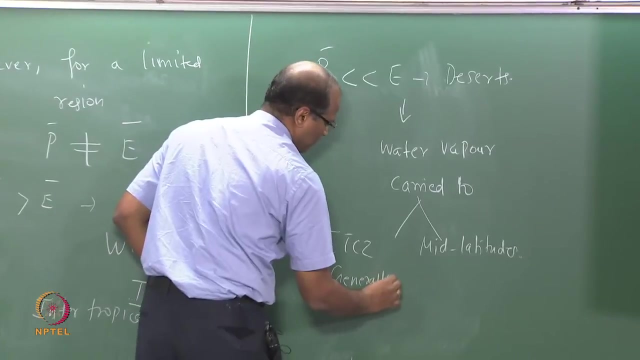 it will go either to the mid latitudes or to the equator. So there is heavy incoming solar radiation, lot of clear skies, heavy evaporation, but no rain. ok, So the water vapor carry to, but generally in continents it is available only at low and low pressure. So this is continue to be the case In the 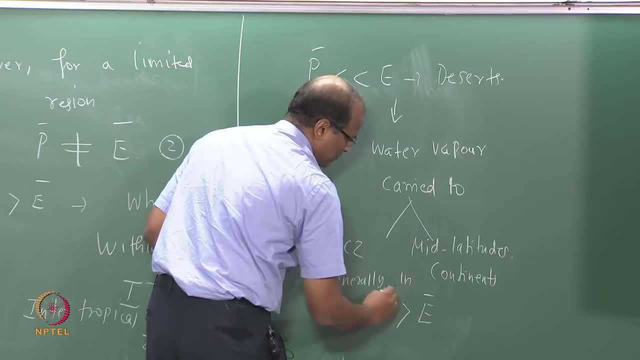 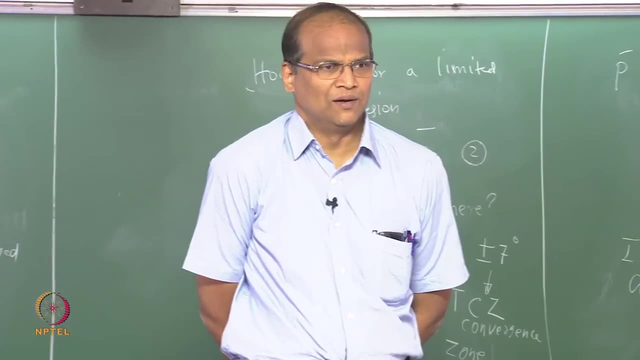 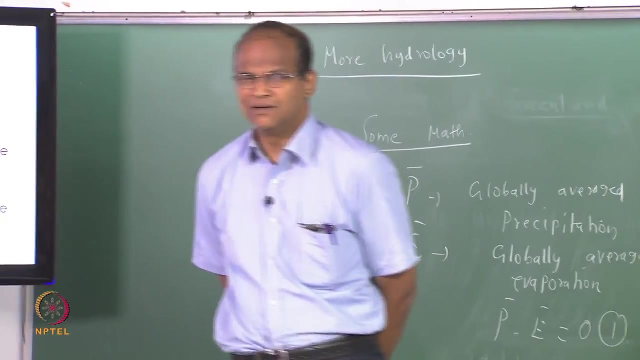 seen that P is greater than E, which is very good for us. this is responsible, So this P is greater than E, one of the primary reasons why there is sustenance of plant, animal and human life continents. So all right over the continents, it is seen that the precipitation 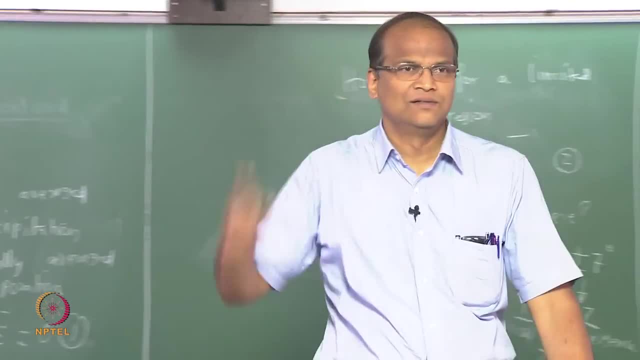 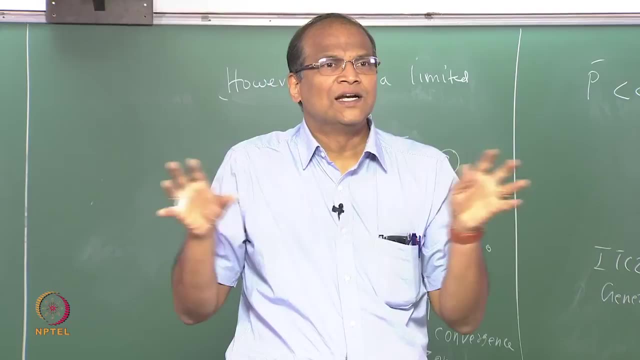 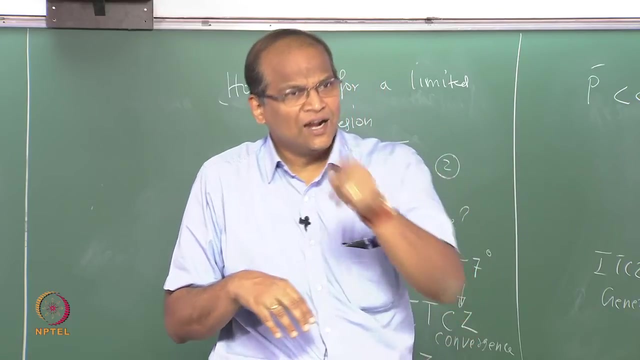 is more than the evaporation. Now, in the next class, in the next class, we will just take a column, we will just take an atmospheric column. apart from P minus E, there is also a transport of water vapor which is coming by the winds. So P? E and transport by wind. 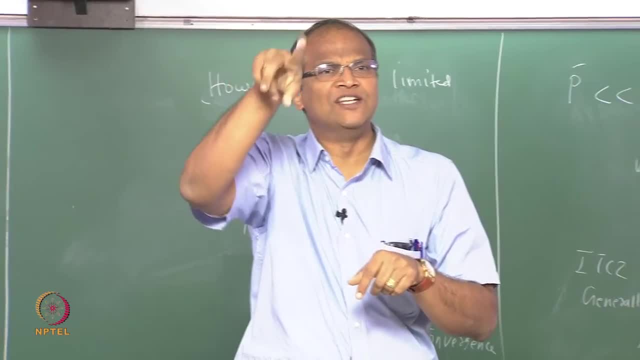 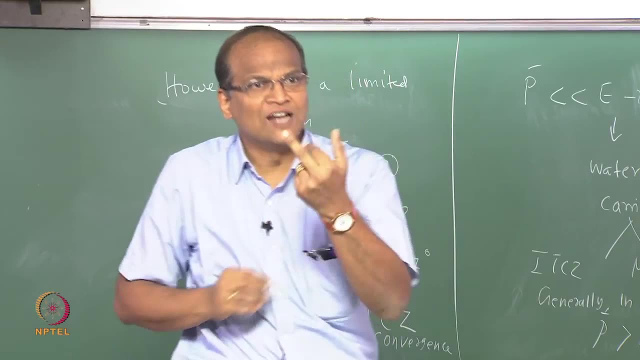 must also come. and if P, E and transport by wind T are not in balance, there is a net change of water vapor in the reservoir. So you will get an unsteady equation. that will be the. so that is an atmospheric unsteady equation. ok.